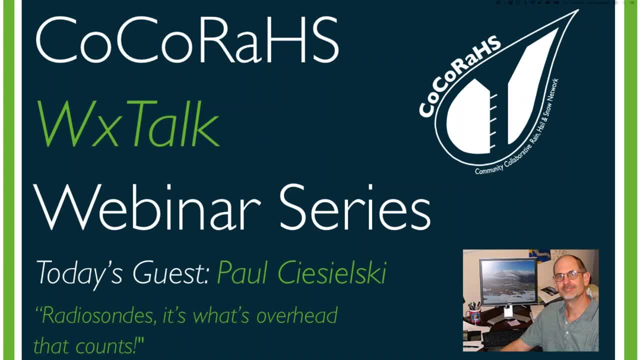 those are, but we're going to talk more about those and we're very lucky to have with us today, on this lofty subject, Paul Ciselski from CSU. Paul was born and raised in South Bend, Indiana. He was a professor at the University of Minnesota, at the University of Minnesota. 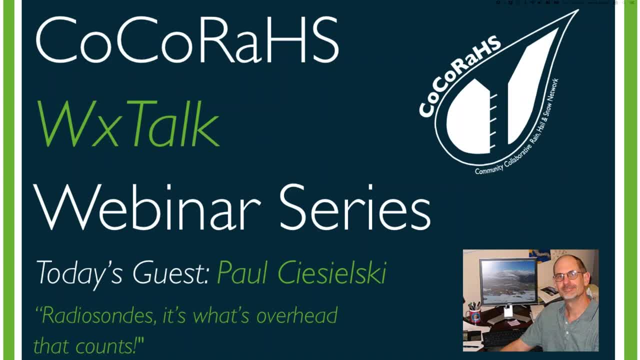 He got interested in weather. Well, South Bend lies in the spot where you get lake effect snow and he would check the nightly weather TV forecast to see if school would be closed the next day. I remember doing that too. where I grew up on Long Island, Paul went and got his undergrad degree. 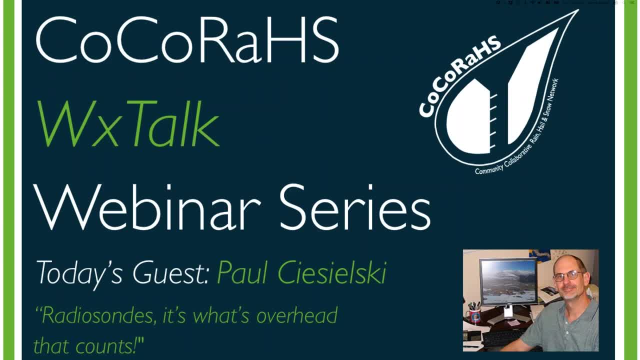 in meteorology from Purdue University and then received his master's here at Colorado State University. His hobbies include cycling, gardening, fishing, climbing 14ers and I forgot. I think he was a student. He was a student at the University of Minnesota, at the University of. 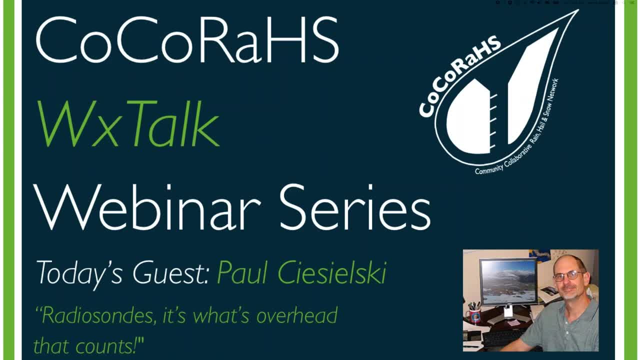 Minnesota. He's done over 20 14ers and then he spends a lot of time with his family and friends. So, Paul, welcome, It's great to have you with us today and thank you for joining us. Well, thank you, Henry. It's a pleasure for me to be here with you today and give this talk. 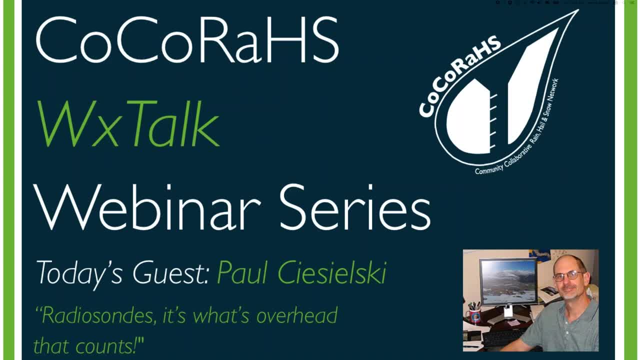 about radiosomes. Paul, let me ask you quickly: how did you get interested in radiosomes, Any event, or anything like that? Well, in 1992, someone in our department, uh, asked me to get involved in a field program that they were having in the West Pacific. 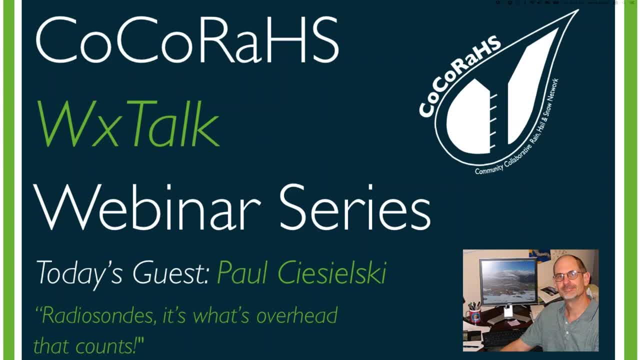 which involved launching radiosomes. So I had a rough assignment. I had to go to Australia for about a month and help to uh quality control the data that was coming in. So that was my first experience using radiosome data. but then about in 2008,- uh, our department actually has a radiosome. 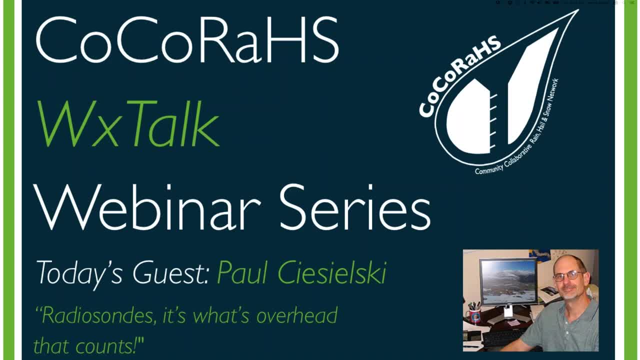 system And the fellow who was in charge of it asked me if I could take over uh the responsibilities for that system. So after that time I really was able to get a a lot of hands-on experience working with uh radiosomes and we've used uh our department system in in several 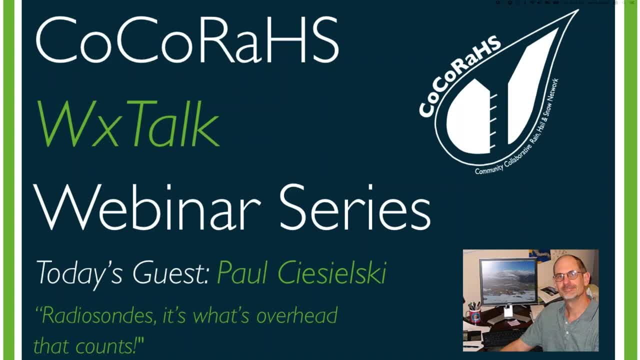 uh field campaigns in recent years. So how many radiosomes do you think you've launched in your, in your career? How many Uh? just myself, A few hundred, but I've probably looked at uh several hundreds of thousands. 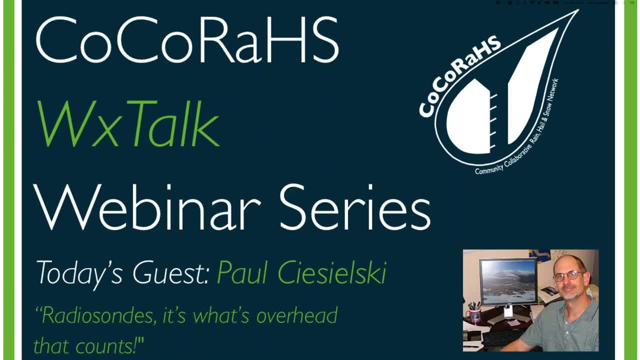 Wow, And so are you, the guy at at the birthday parties, in in charge of blowing up the balloons at home. Uh, yeah, that's one of my duties. Okay, All right, Paul Well, thanks a little. We'll let you take it away here with your. 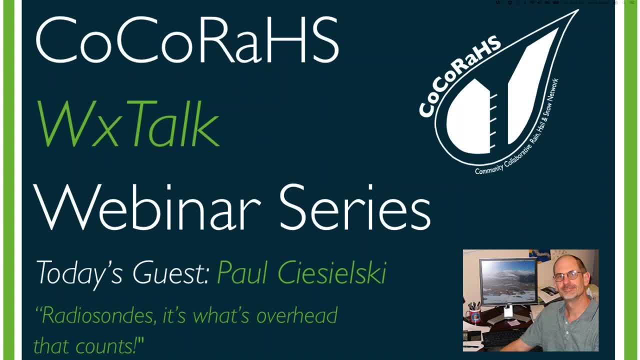 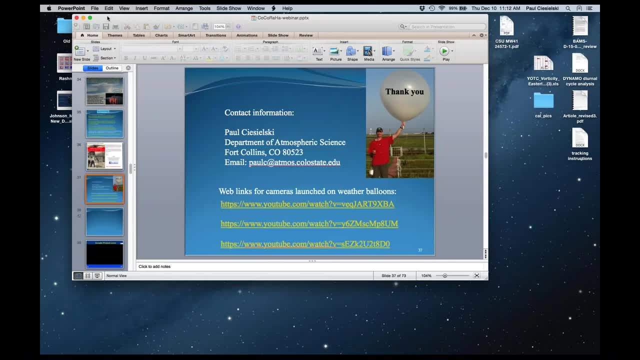 presentation. We'll be back, uh, with questions from our audience afterwards, So thank you again for being here. Okay, Thank you, Henry And Paul, as you begin to show your screen, as you are now, if you could do us a favor. 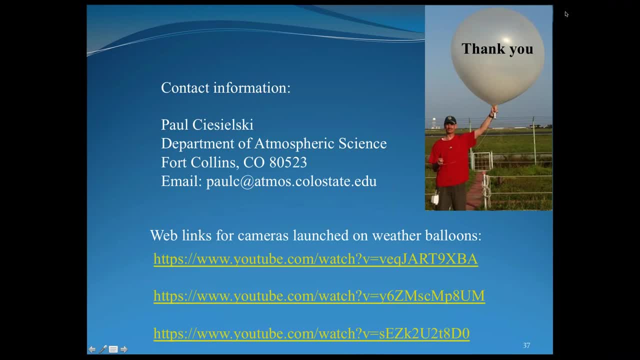 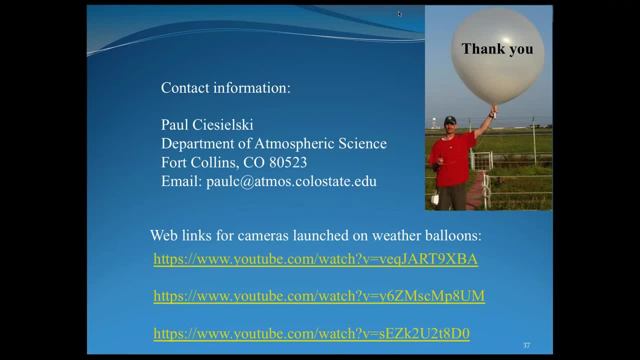 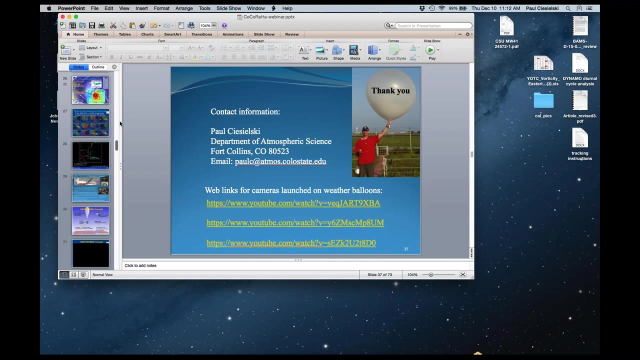 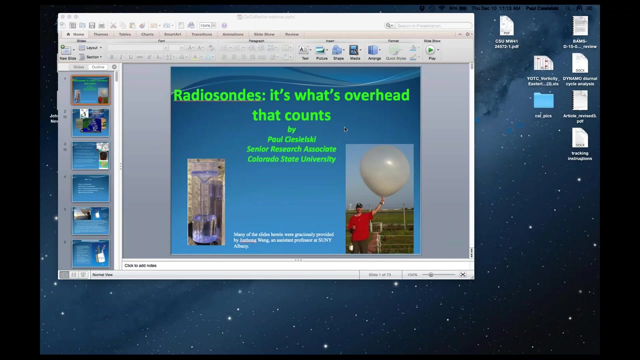 hard to hear you. so, Okay, Is that better? That is better. Thank you very much. Okay, Uh, that's my last slide, So let me go to my first slide here. Great, We're seeing it perfect. 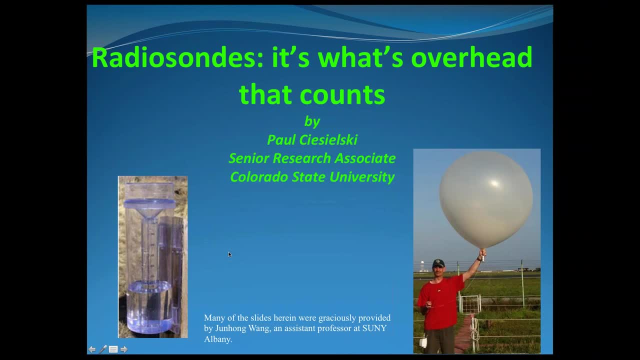 Well, there it is. There it is Okay. Well, once again, it's my great pleasure to be able to talk about radiosondes today and how they're used in the field of atmospheric science. What I'd like to convince you today in this presentation. 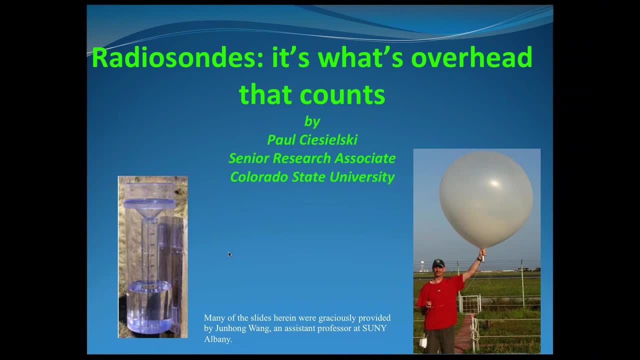 is that, of all the observations that we make of the atmosphere, radiosondes are the backbone of our observational network and the workhorse of our weather forecast. So the observations that we make for cocoa roths, of snow and rain and hail. they help us to verify weather forecasts and observe the climate. 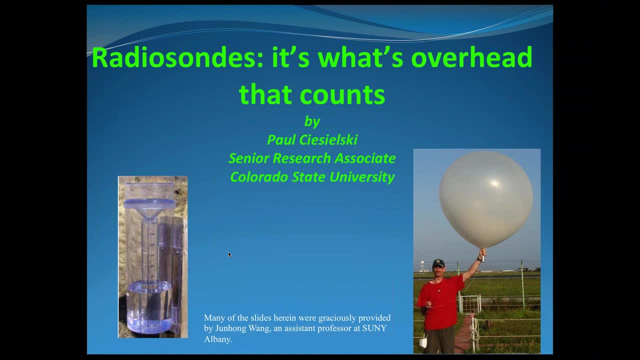 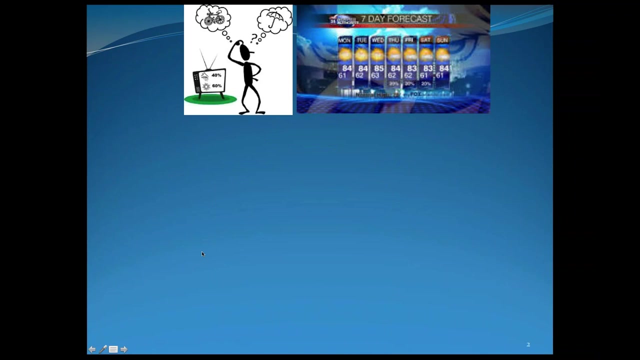 whereas radiosonde data allow us to better forecast the weather and understand our climate and its changes. So if you're anything like me- and let's see if we could advance that- you probably wake up in the morning and you turn on your favorite radio or TV station. 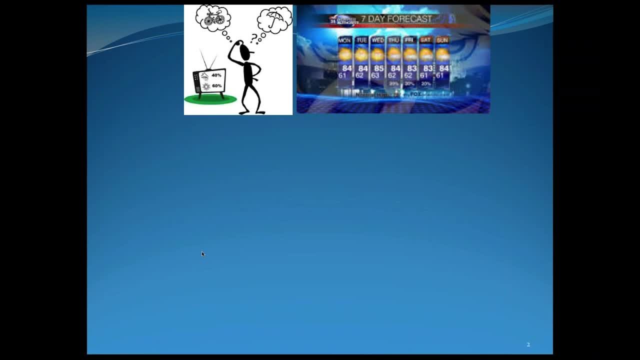 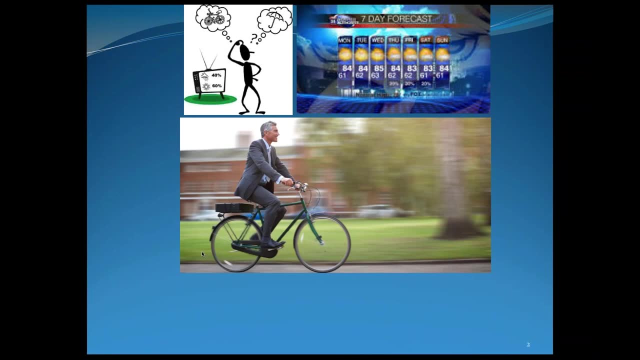 to find out what the weather forecast is for the day or for the coming week. You want to find out if you're going to be able to ride your bike without getting wet or, better yet, go fishing. You may want to know from the forecast. 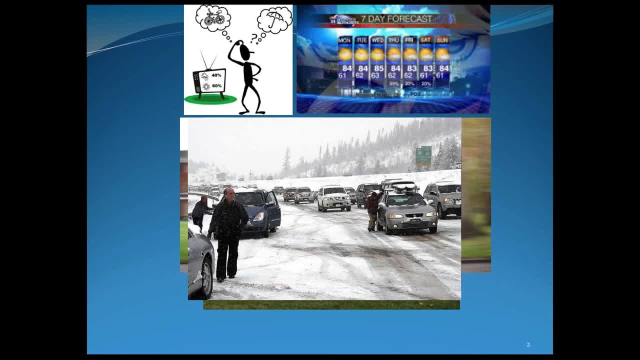 how soon do you need to blow out your sprinklers, Or what the weekend weather forecast is going to be? Is it going to mess up my travel plans So I can hit the slopes like we like to do in Colorado, although I'm not a skier? 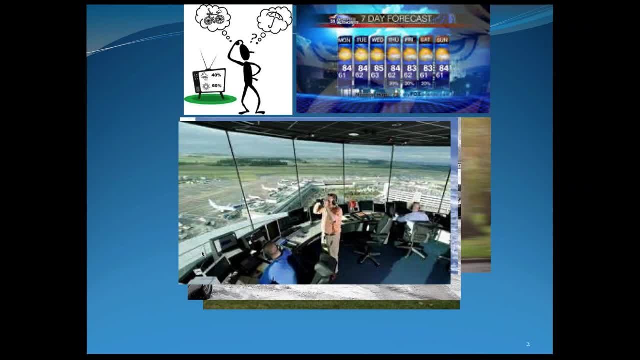 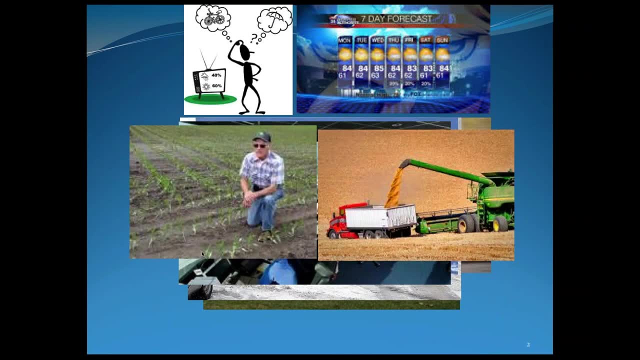 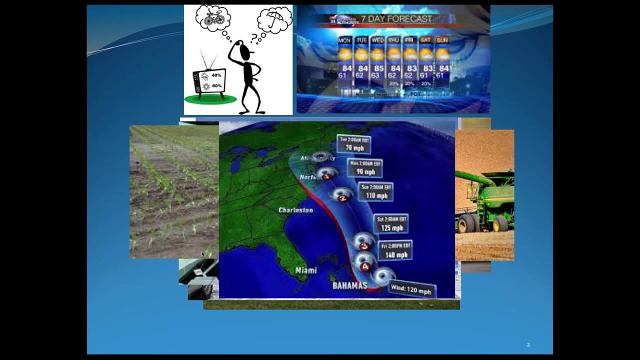 More importantly, accurate weather forecasts can help the airport control tower to know what information to give the planes that are landing or taking off, or can tell the farmer when to plant his crops and when to harvest them. And, probably most importantly, weather forecasts are used to warn residents of coastal regions. 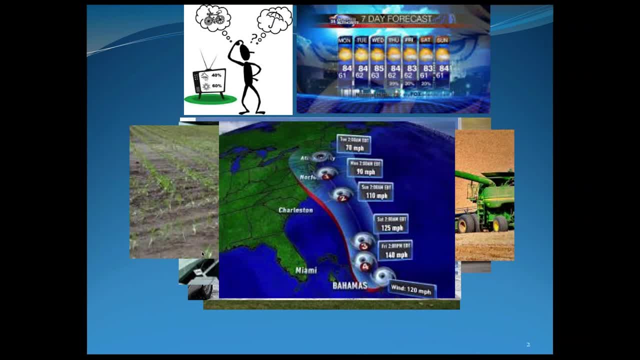 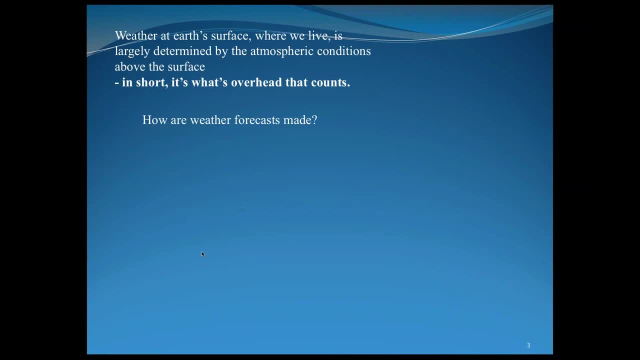 when a hurricane might strike. As it turns out, the weather on the Earth's surface, where we live, is largely determined by the atmosphere conditions above the surface. In short, it's what's overhead that counts. So how do we make weather forecasts? 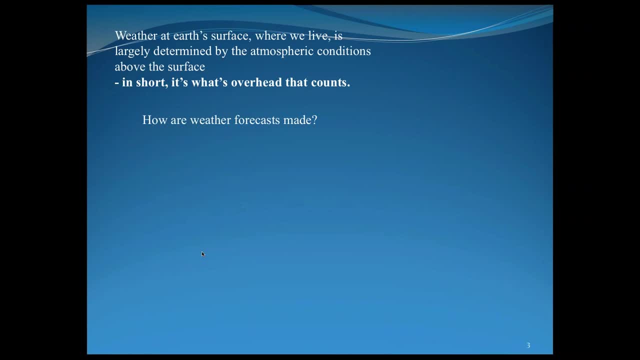 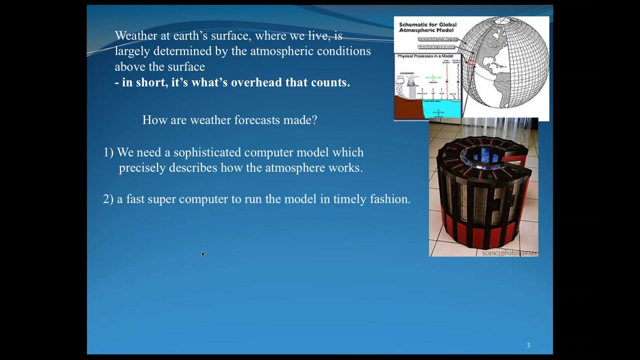 Weather forecasting is basically predicting how the present state of the atmosphere will change in time. So how is this done? First we need a sophisticated computer model which precisely describes how the atmosphere works. Then we need a fast supercomputer to run the model in a timely fashion. 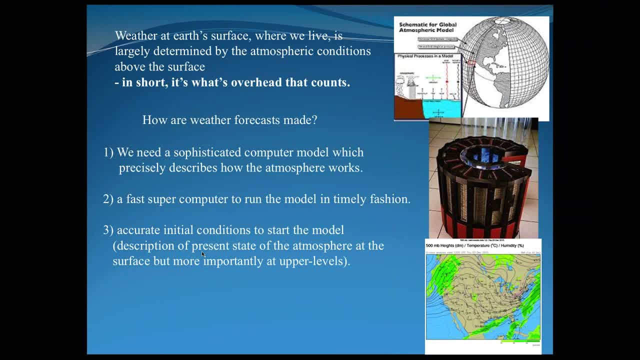 And finally, we need accurate initial conditions to start the model. And by accurate initial conditions I mean we need to be able to describe the present state of the atmosphere. I mean we need to be able to describe the present state of the atmosphere. 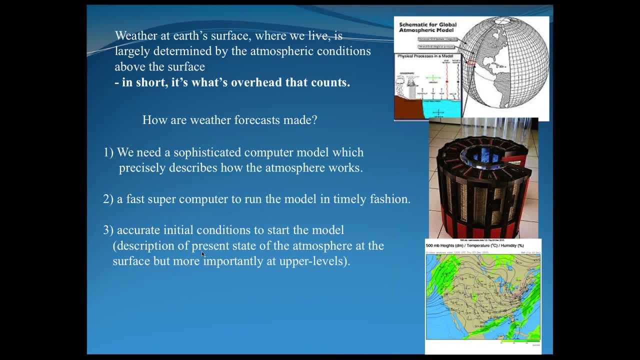 At the surface but, more importantly, at upper levels. And how do we get this accurate description of the upper level air? That's with radiosondes, And that's the focus of today's talk. So let's jump right into it. 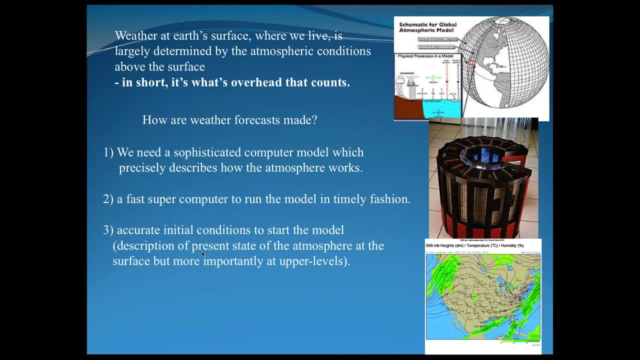 Here's an outline of today's talk. I'm going to talk about what it is a radiosonde, And I'm going to show a video of a radiosonde launch that's made at a National Weather Center. And I'm going to show a video of a radiosonde launch that's made at a National Weather Center. 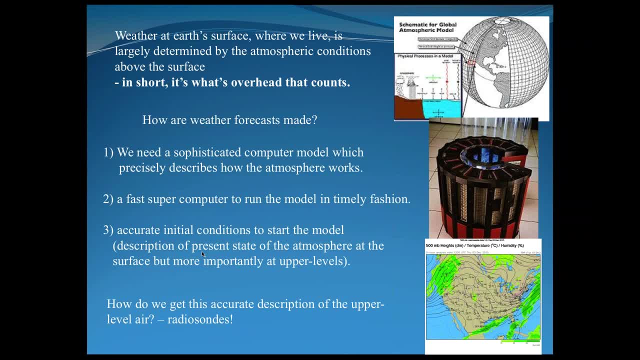 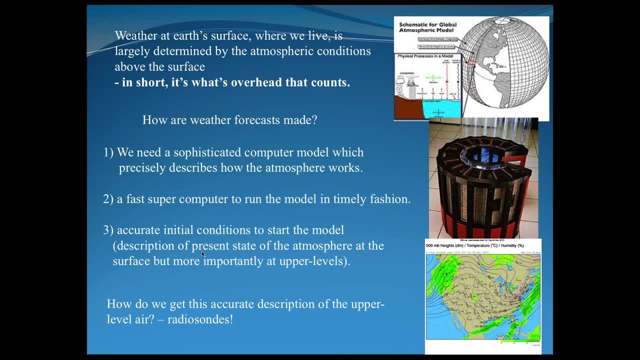 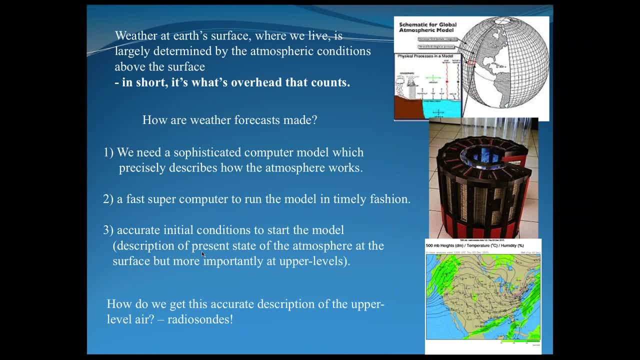 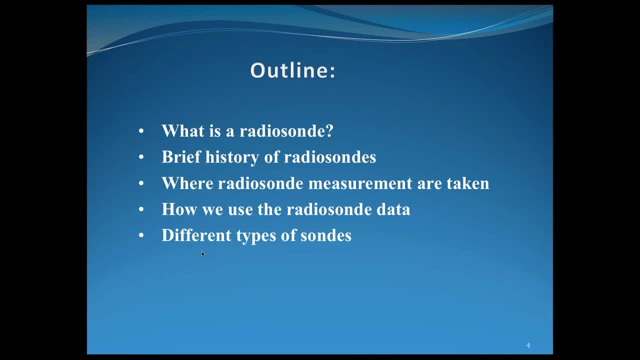 And I'm going to show a video of a radiosonde launch that's made at a National Weather Service Station. And I'm going to show a video of a radiosonde launch that's made at a National Weather Service Station. I'm going to give a brief history of radiosondes. talk about where radiosonde measurements are taken. 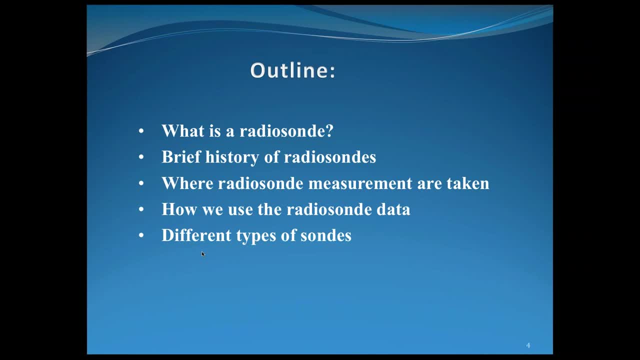 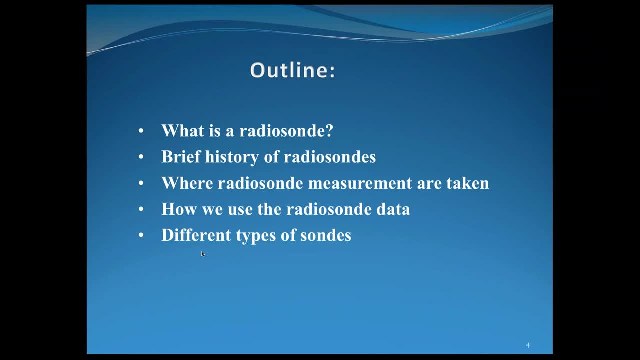 I'm going to give a brief history of radiosonde measurements are taken, how we use the radiosonde data and then look at some different types of sondes. how we use the radiosonde data and then look at some different types of sondes. 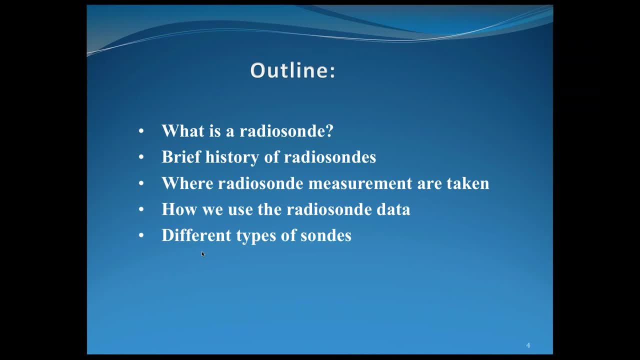 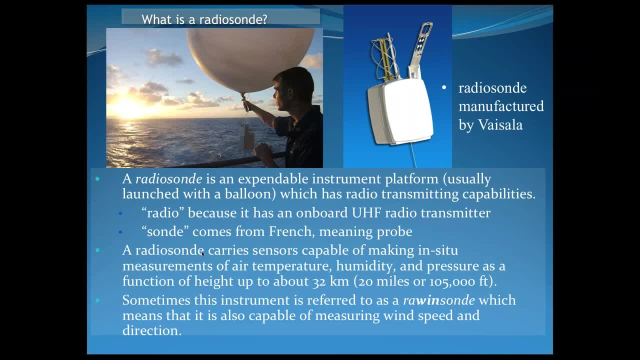 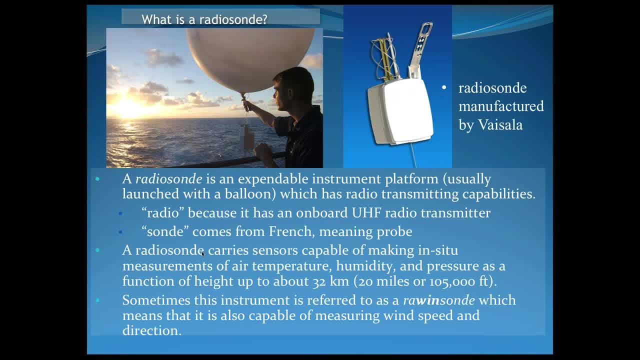 So what is a radiosonde? Radiosonde is an expendable instrument platform, and by expendable I mean we launch it and we don't get it back, and it's usually launched with the balloon. It has radio transmitting capabilities. Radio because it has an onboard UHF radio transmitter, and sonde comes from a French. 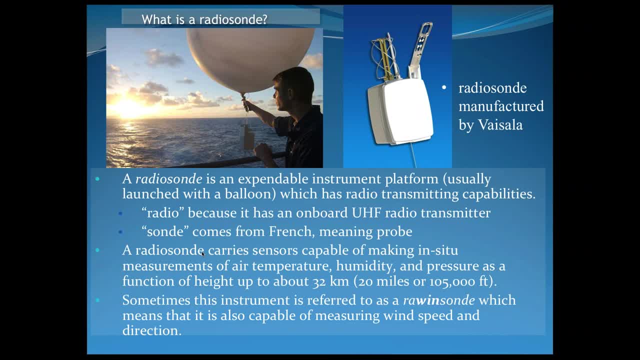 and German word meaning probe. So basically what we're doing here is we're probing the atmosphere to see what the conditions are like above our, above the ground, and it's being transmitted back to the ground with radio waves. So a radiosonde carries sensors capable of measuring in situ or in place measurements of air temperature. 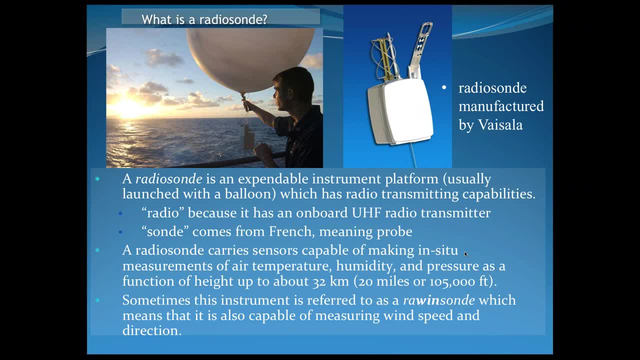 humidity and pressure, as a function of height, up to 32 kilometers, So that's about 20 miles or over a hundred thousand feet. Sometimes this instrument is referred to as a ray-wind sonde, which means that it is also capable of. 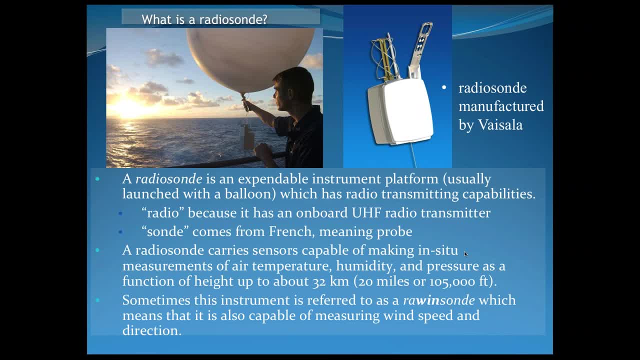 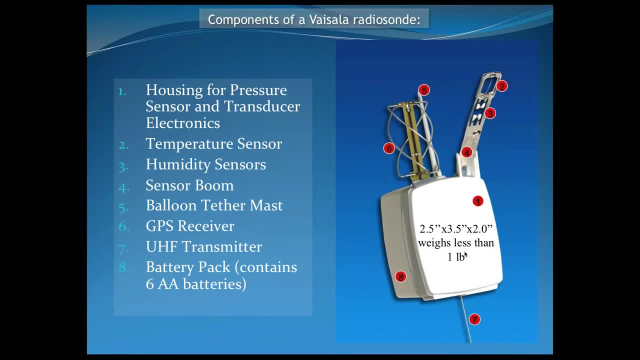 measuring wind speed and direction. In this talk I'm just going to refer to it generically as a radiosonde or sonde. So this slide looks at the components of a radiosonde, and this particular one was manufactured by Vaisala, which is a company headquartered in Finland. Now 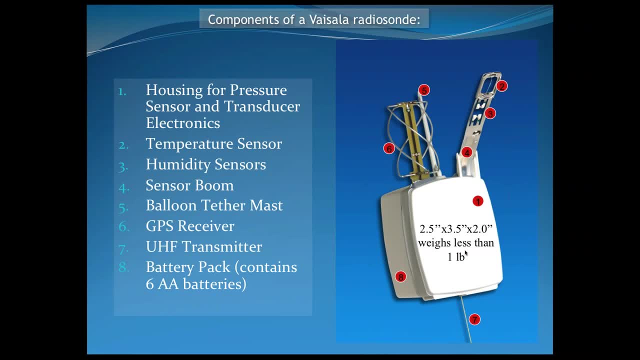 there's at least 50 radiosondes in Finland. There are 15 different types of sondes that are on the market today. This particular one happens to be one of the most accurate and most widely used, So the numbers here actually identify the various parts of this sonde. I should mention that the 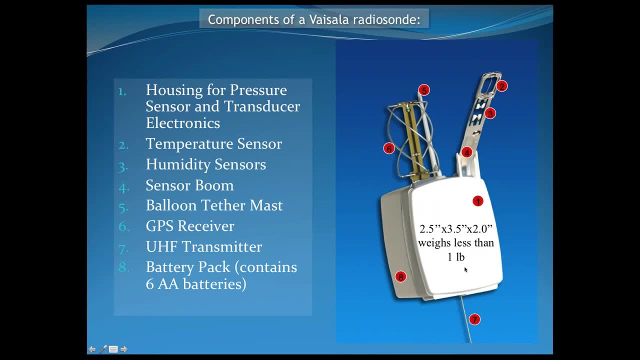 sonde is pretty small in size. It's two and a half inches by three and a half and two inches deep, and it weighs less than a pound. So that's fairly small. Now, number one here is the housing for the pressure sensor and the transducer. 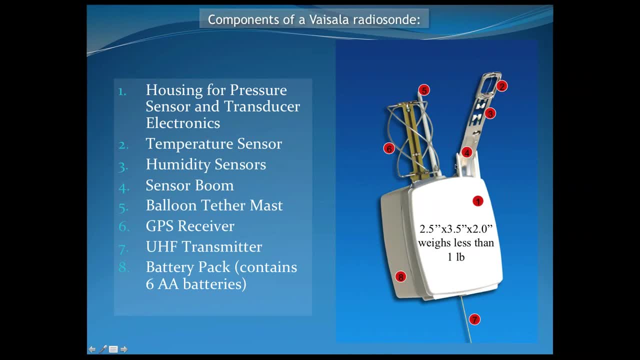 electronics. And then, if you look at number four, here, this metallic sensor boom contains instruments for measuring the temperature- number two- and the relative humidity- number three- And it does this by measuring changes in the electrical capacitance Which are caused by changes in temperature and relative humidity. Now, this cool-shaped 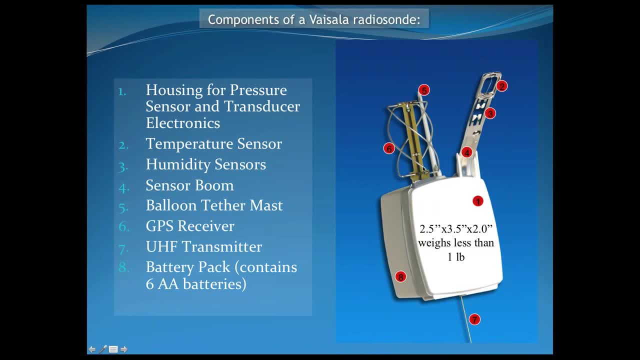 helical device. number six is actually the antenna for receiving data from the GPS satellites, which provide information about the location of the sonde from which we can compute the winds. The wire at the bottom here, number seven, is the UHF antenna, which is used for transmitting. 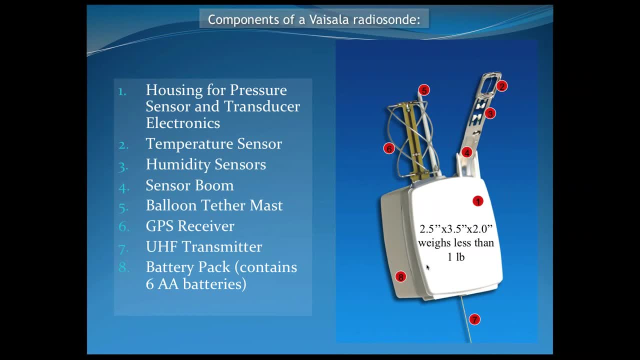 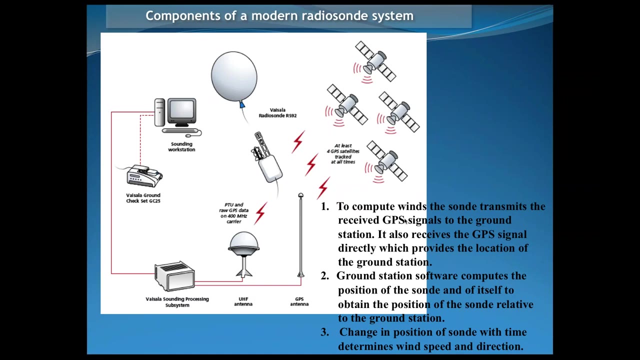 the data collected by the sonde. And number eight here contains it's the container for six AA batteries which power the sondes. So this slide shows the components of a modern radio sonde system. The radio sonde and the balloon, as I mentioned, are the expendables. We launch them, we don't get them back. So 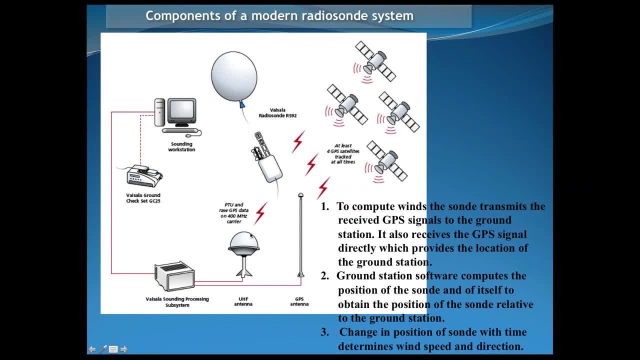 the sonde sends the data back through the UHF To the UHF antenna to the ground station. The ground station system processes all the data and displays it on the sounding workstation. The sounding workstation also has attached to it a ground check system which helps us to calibrate the sondes prior to launch. 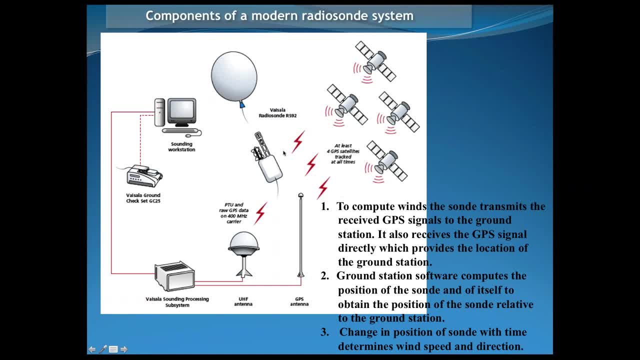 Now to compute the winds. the sonde transmits data received from GPS satellites, So here I'm showing four GPS satellites. You need at least four GPS satellites in order to track the position of the sonde. This usually isn't a problem. Usually we can track at least a dozen of the GPS satellites. 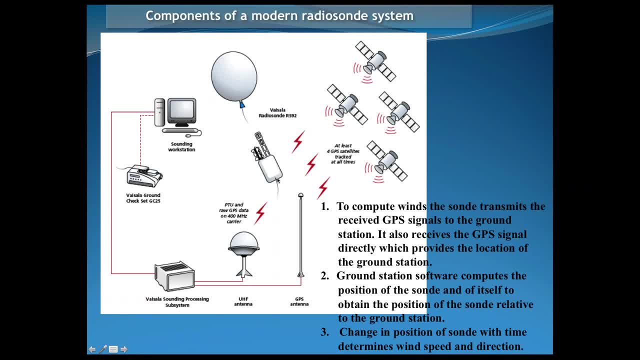 So the sonde receives this information from the GPS satellites and transmits it back to the ground. And it also connected to this ground based processing system is a GPS antenna which tells us the location of the ground station. So the ground station software, it computes the position of the sonde and of itself to 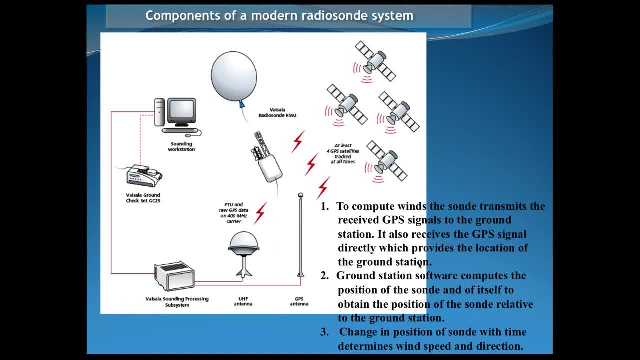 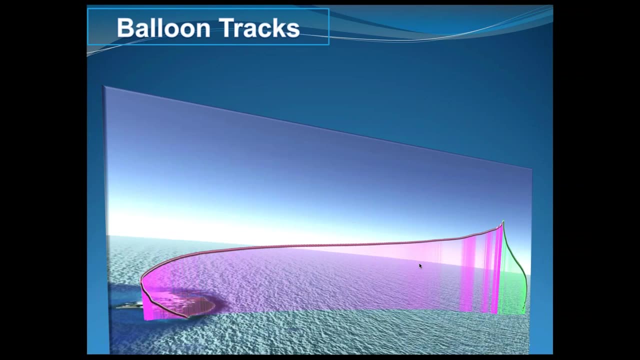 obtain the position of the sonde relative to the ground station, And then the change in the position of the sonde with time determines the wind speed and the direction. So, having the GPS information, we can graphically display the track of a sounding. Here's an. 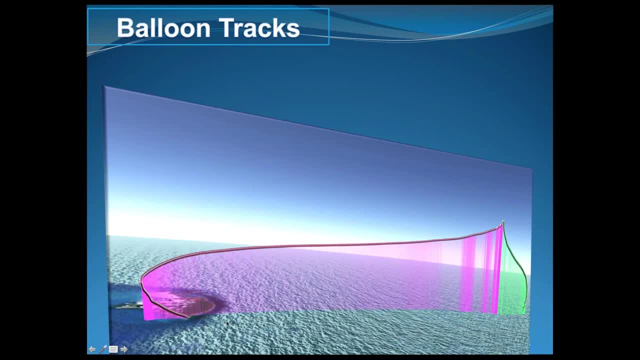 example. In this example we see that the sonde is in the direction of the ground station, So we can graphically display the track of a sounding. Here's an example. In this example the sonde is ascending through a deck of shallow clouds and it changes the direction. 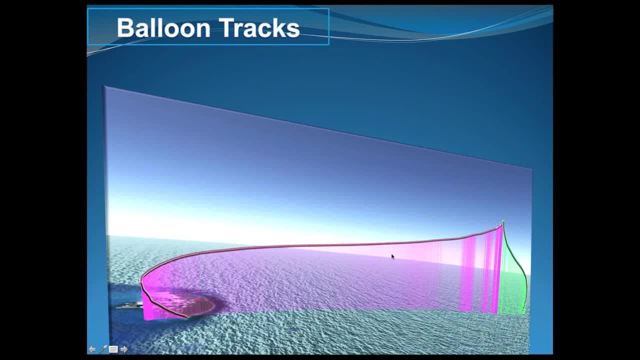 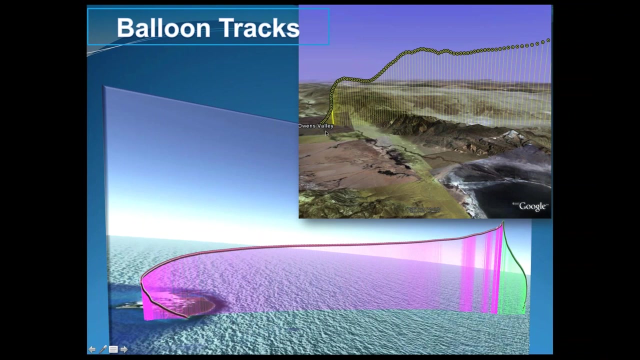 It's rising at a rate of about four to five meters per second, getting through the troposphere and into the stratosphere, And then the balloon bursts and it quickly descends. Here's a second track. This one is rather interesting and it was launched from Owens. 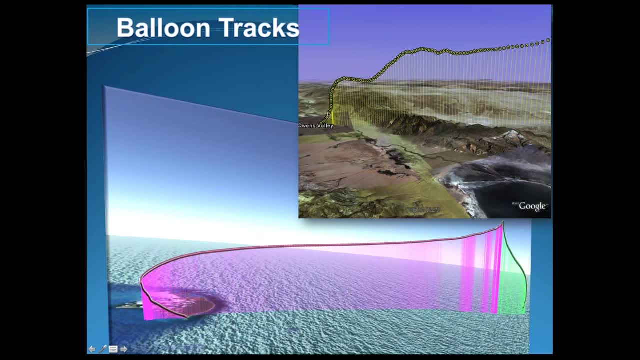 Valley in California And it shows that the balloon, after it has ascended for a while, it actually descends for a short period of time. It's actually encountering strong sinking motion that's induced by mountain waves generated by upstream flow from the Sierra Nevada mountains. 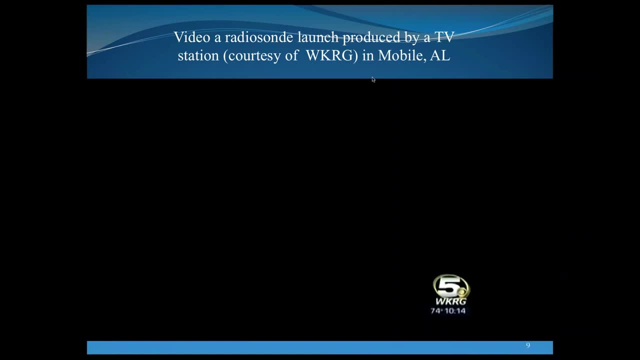 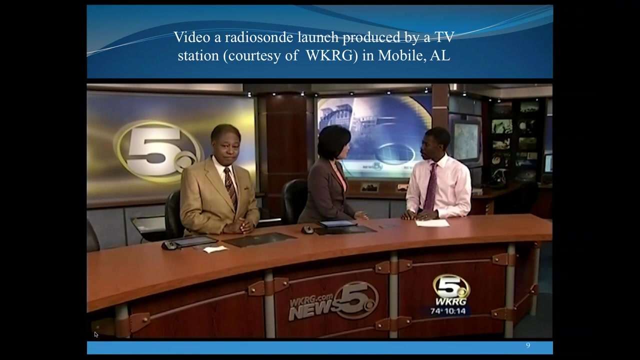 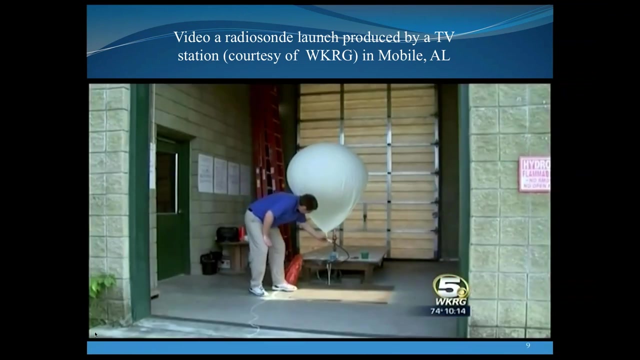 So to give you an idea of what a Radiosonde launch is like, here's a short video that's been prepared by TV station in Mobile, Alabama. This is the story of a man and a balloon. My name is Jim Salswiddle and I'm a. 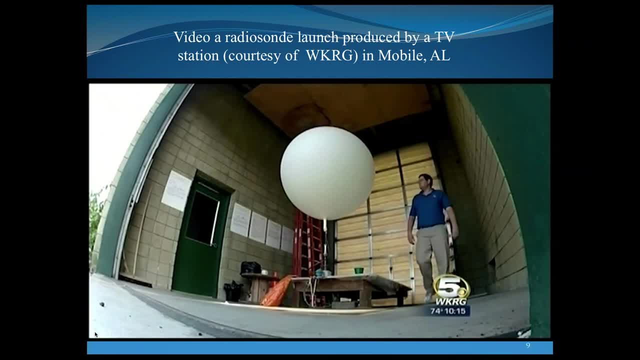 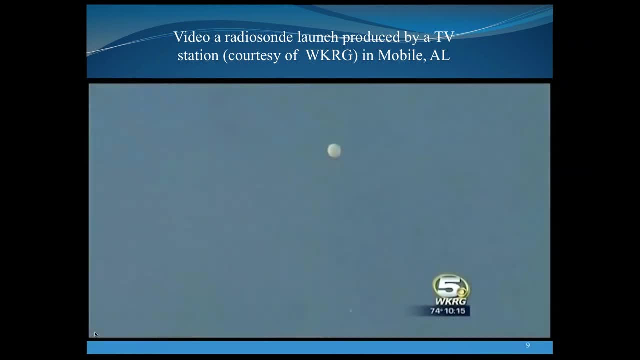 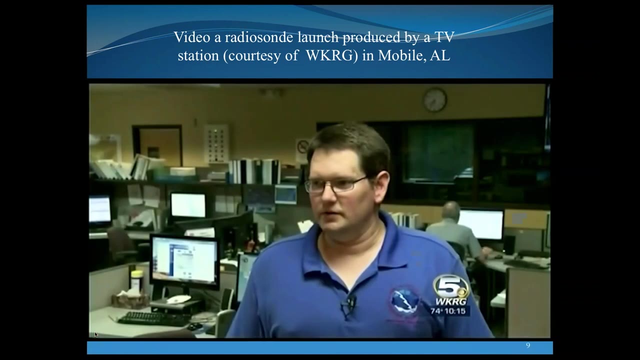 hydrometeorological technician Jim is preparing to launch a weather balloon with Radiosonde in Slidell, Louisiana. We're an official upper air site for the National Weather Service. The weather balloon carries instruments to measure weather in the upper air as it rises. The data is highly, highly critical for the 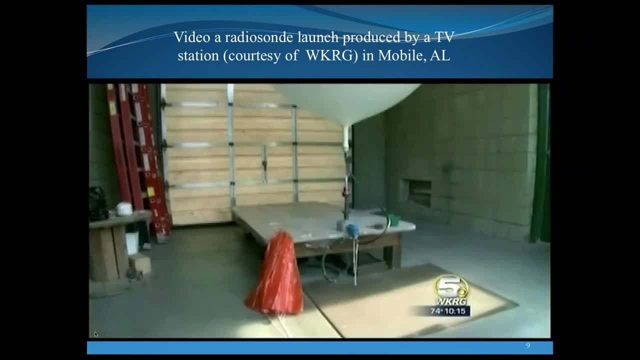 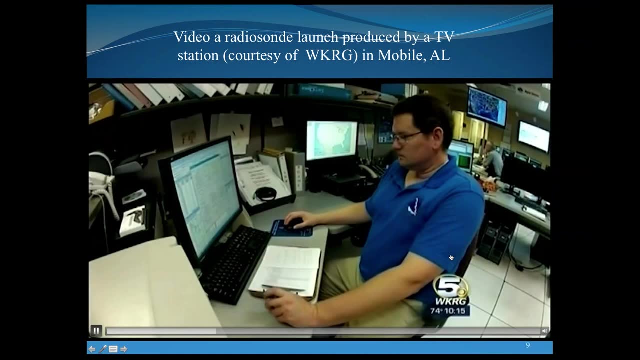 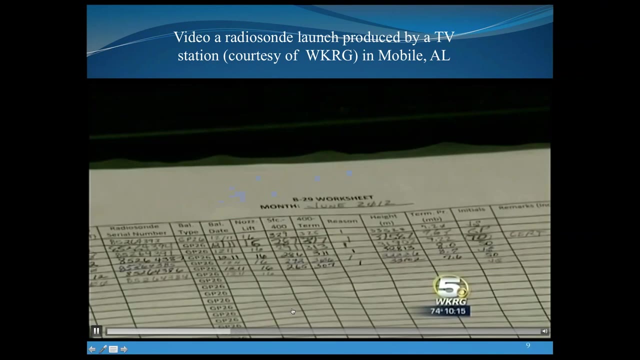 weather modeling process to get the best available forecast. This launch is choreographed twice daily, With launches at over 90 locations in the United States and another 700 worldwide, at 23Z and 11Z locally during daylight time, at 6 in the morning and 6 at night. 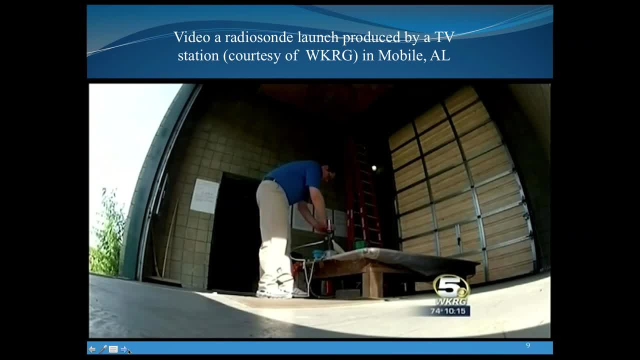 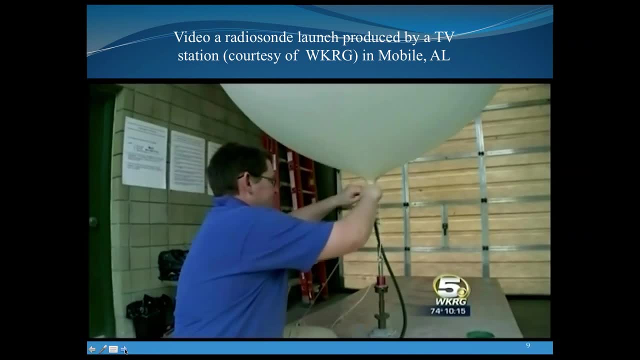 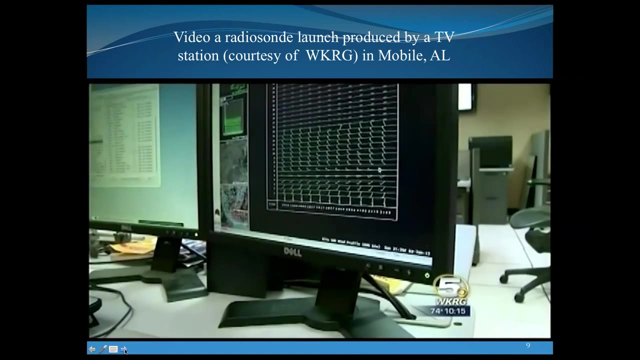 This step is pretty obvious: Filling up the weather balloon and then tying it closed. Nothing's worse than letting a balloon get out of your hands Before the launch. Jim is on a computer Looking at the upper wind flow, so we get. we have a good idea of where the 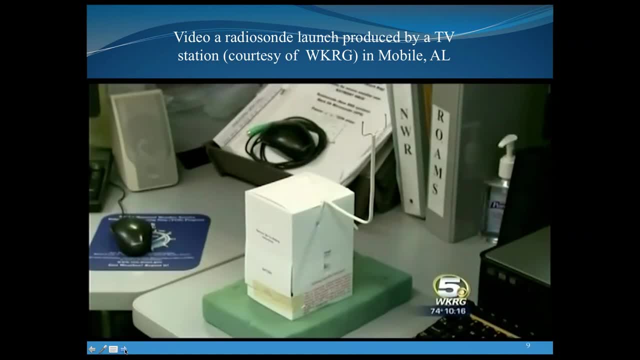 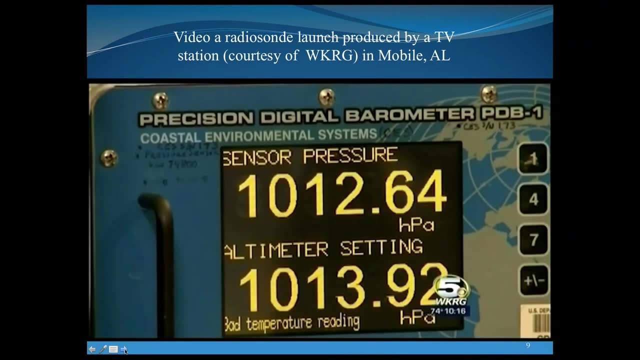 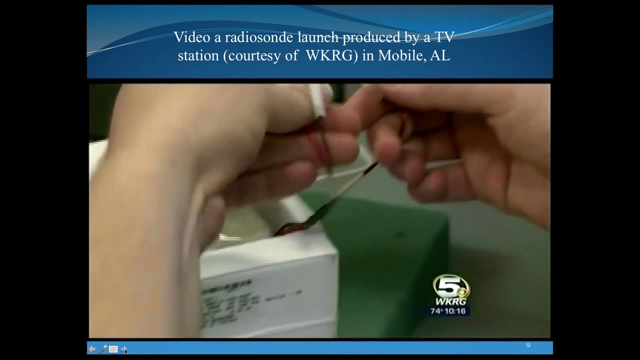 Radiosonde is going to travel. after we release, The Radiosonde is then checked for accuracy. We compare that with weather instruments that we have here at the office to make sure the Sonde is actually that the data is correct before we actually release it. A battery powers the sensors for temperature, humidity and 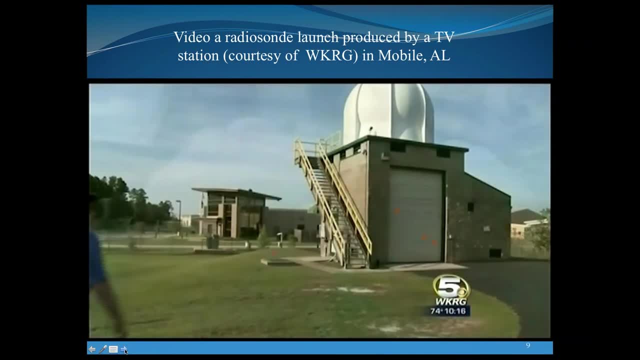 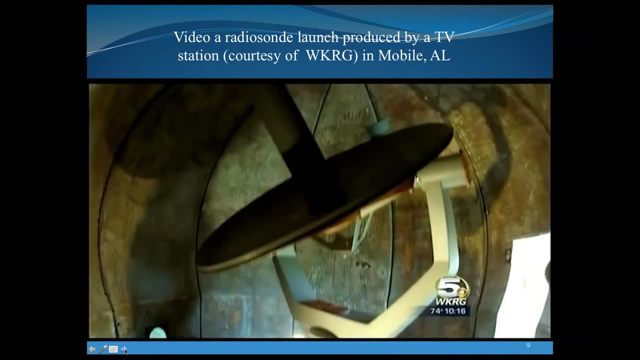 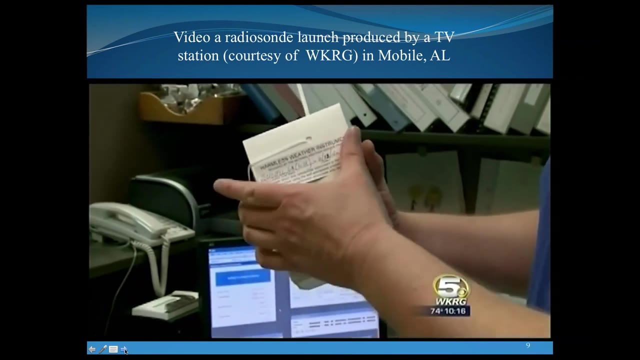 pressure, as well as a GPS unit used to help determine wind. It transmits the data back to the telemetry receiving system so that way we can get the data real time, Because the instrument may end up landing in your backyard. We put this sticker on here to let folks know it's a harmless weather instrument. 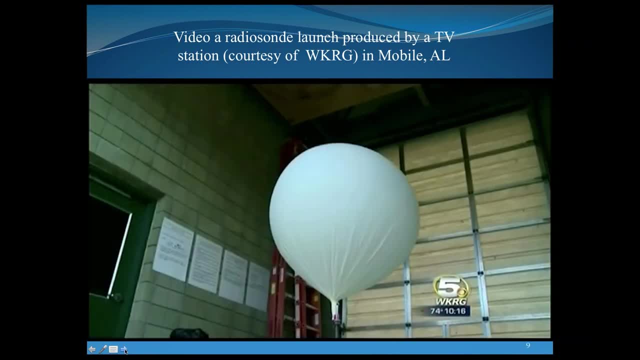 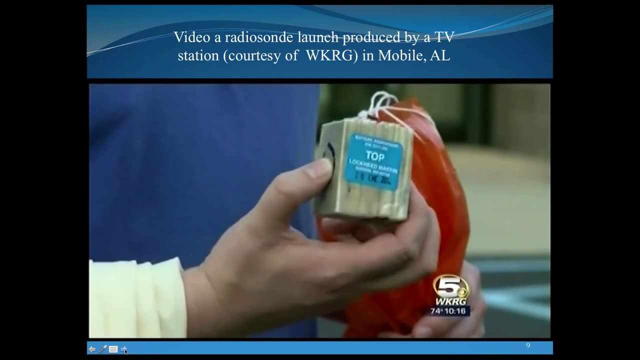 Harmless, but the balloon may contain hydrogen. You want to take great care and caution in handling that because it is a flammable gas. Also, if you find a recently used radio sonde, the batteries might be hot or hissing. 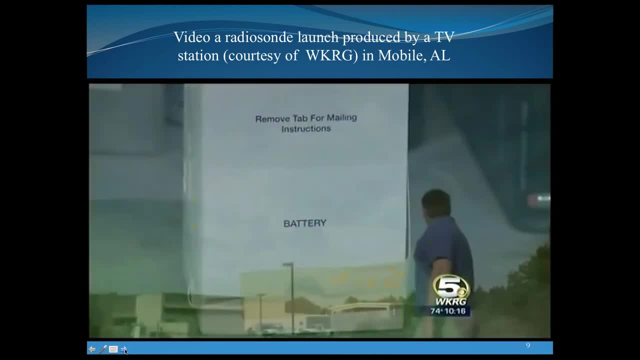 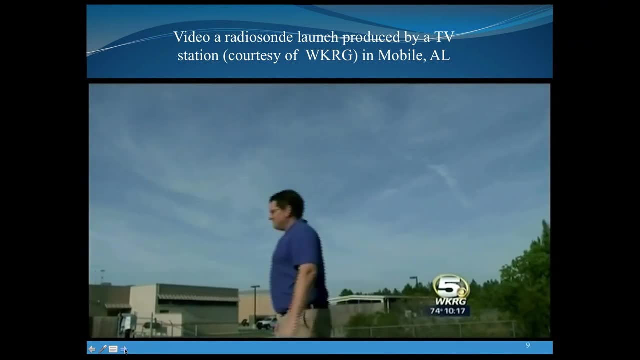 Just let them cool and quiet down before handling. It's not a hazard. And now it's launch time On a sunny day, So we watch out, for aircraft Have to really be careful of different obstacles- trees, power lines- But on a stormy day. 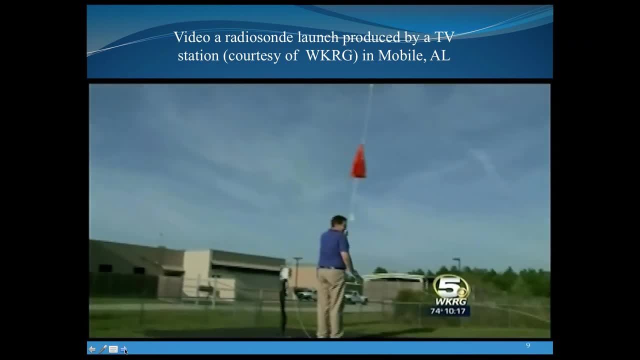 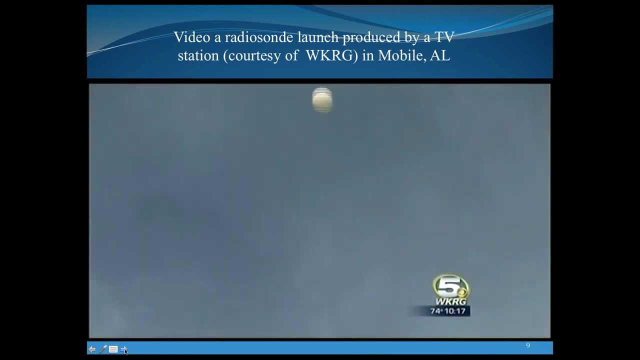 You might only have a five or ten minute window before the next line of storms. Either way, the data is valuable. Typically, when we release the balloon, it's right around five to six feet in diameter, But it's not a hazard. But as it goes through the atmosphere and expands through the higher altitudes, this actually expands to almost 20 feet or greater before it actually bursts. Usually at our office, our weather balloons burst at over 105,000 feet, That's 20 miles up. How far it travels Really depends on how strong the upper level winds are. 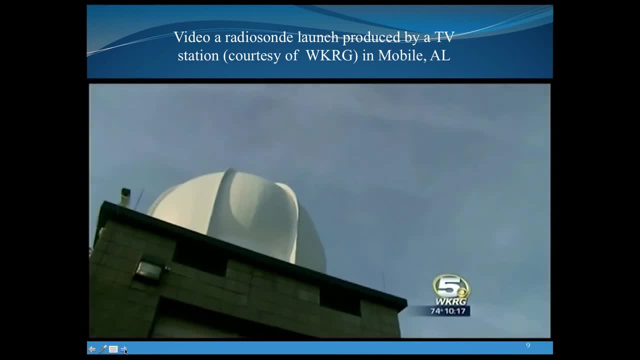 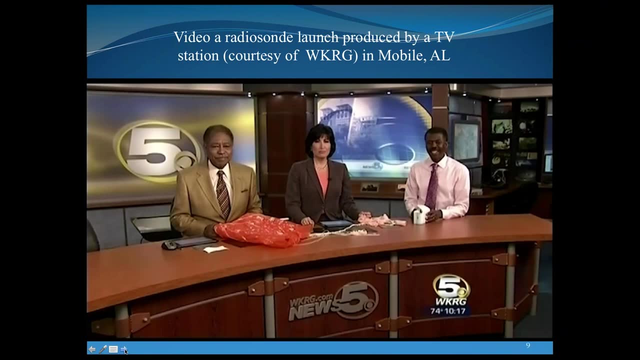 The balloon may travel a dozen miles away or a couple hundred miles away. No matter how far it travels, it's all for the data And we'll be right back. What we have in front of us is clear evidence that it can travel 100 miles land here in Mobile. 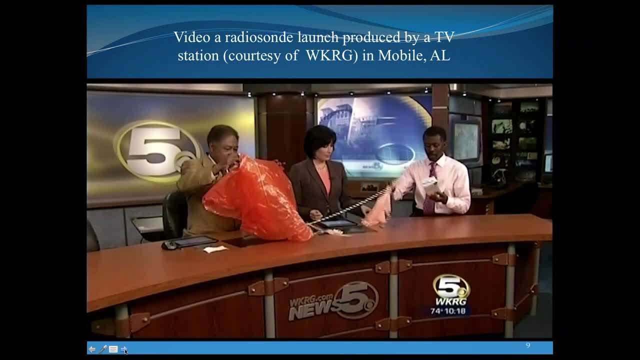 That's the parachute. This is the latex balloon, This is the radio sign. And the cool thing is, if you ever find it, you open it up. there's a self-addressed envelope from the National Weather Service. You take it to the post office, give it to the clerk, they send it back to be refurbished and they send it up again. 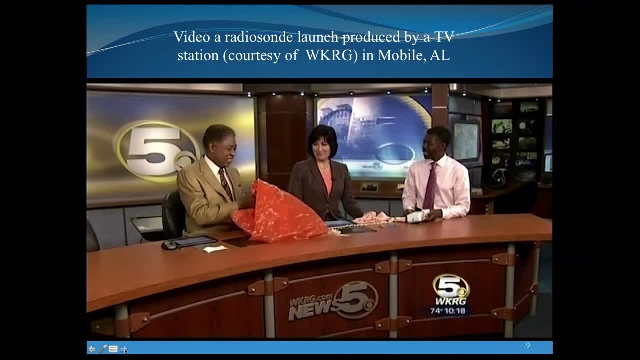 Very cool, Really interesting. Yeah, kind of fun stuff, But twice a day, day and night. that's the other fascinating part: Our weather it is So that shows how Radio signs are launched from the National Weather Service offices. 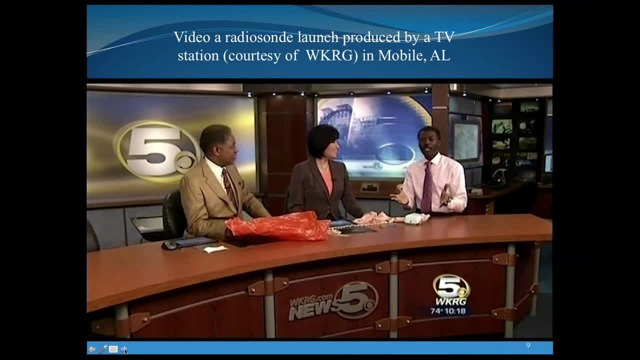 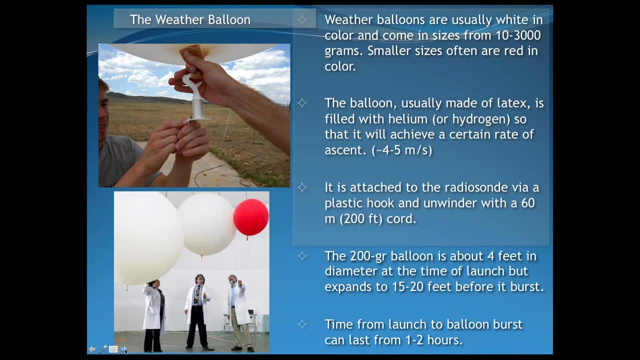 And we're going to take a look at a map of those in a few moments. One of the most asked questions, especially when I give these presentations at the school, the kids want to know about the weather balloons. So I threw in a slide here which talks a little bit about the weather balloons. 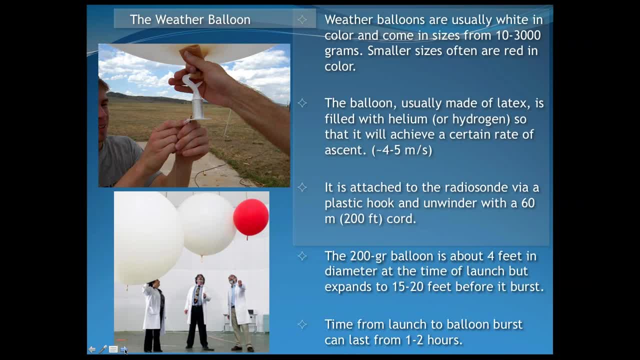 Weather balloons are usually white in color and they come in sizes from anywhere from 10, to 3,000 grams, so that's less than a pound to up to six pounds, And the smaller sizes are often red in color. The balloon is usually made of latex and it's filled with helium or hydrogen. 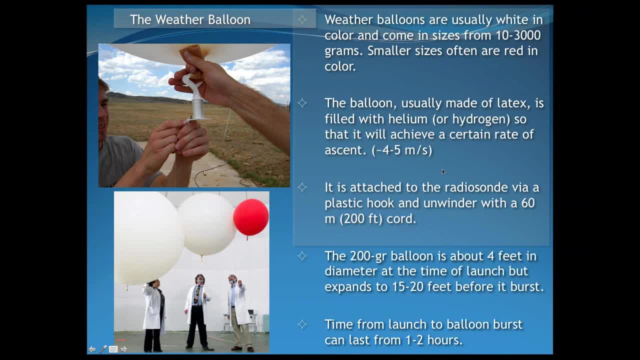 Now, helium is more expensive but hydrogen is more dangerous because it's extremely flammable. So we try, at least with our department's on system is we try to achieve a rise rate of four to five meters a second So that the sensors on the sonde will be well ventilated. 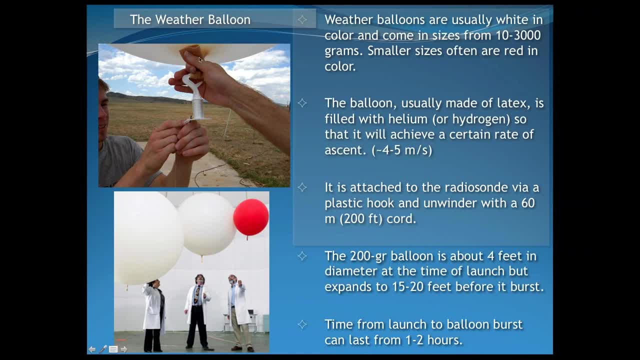 The sonde is attached to the balloon by this hook and then there's a 200 foot cord or string that attaches the sonde to the balloon And there's quite a distance between the sonde and the balloon because you don't want the balloon to interfere with any of the measurements of the radio sonde. 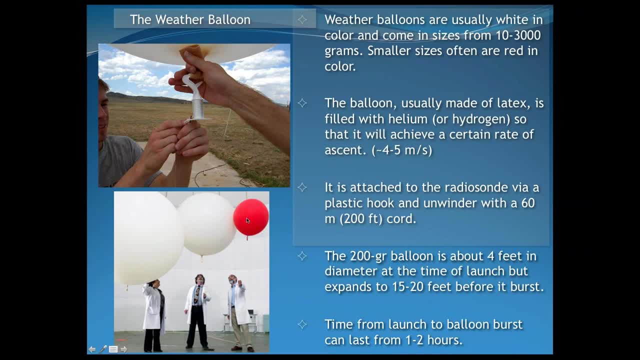 The 200 gram balloon is a very complex balloon that we use in our department. launches is about four feet in diameter at the time of launch, but it expands to 15 to 20 feet before it bursts. and here just show some different examples of different sized balloons. this is about 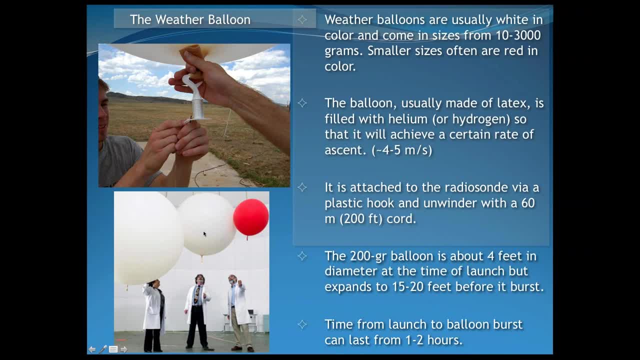 the size of the balloon- the one in the middle here that we use in our department launches. the Weather Service uses larger balloons, more like 1,200 grams, so they're larger in size when they launch and they get higher. and this is a balloon that they used on pie ball observations and we'll also talk about. 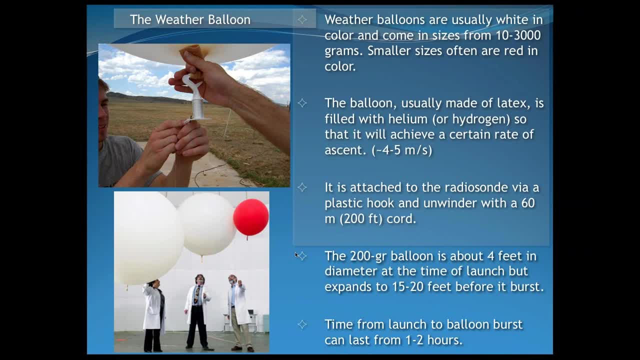 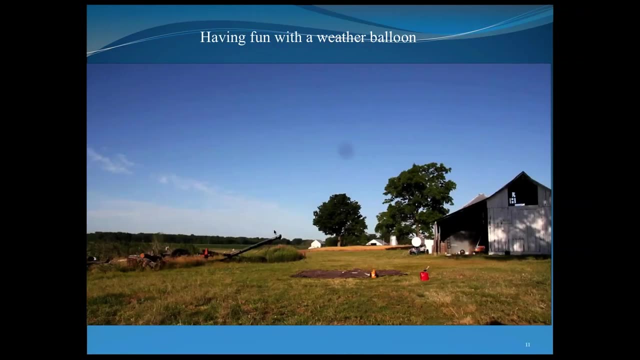 that. so the time from launch to when the balloon burst can typically be from one to two hours, depending on the size of the balloon. bigger balloons will take longer before they burst, so I wanted to show this video. it's just a fun video and it gives you some idea of just how big balloons can get before they burst. 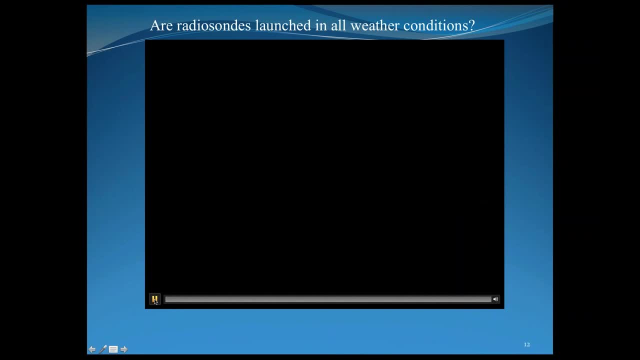 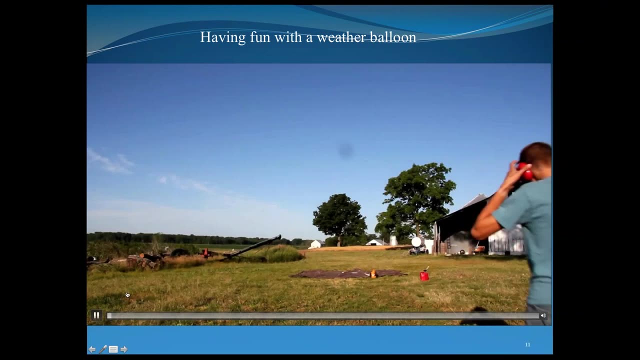 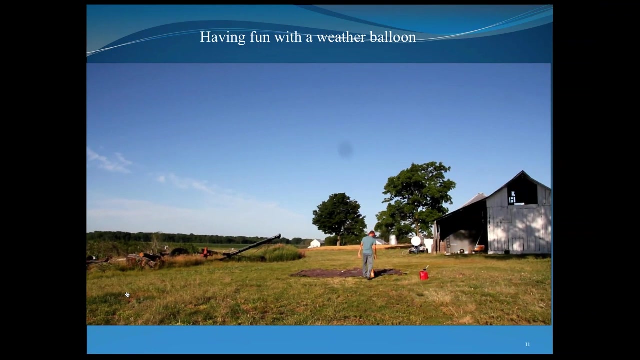 let me go back here. so this man is blowing up the balloon with the gas powered leaf blower. if he can get it started, there he goes. I'm going to blow up the balloon with the gas powered leaf blower now in slow motion. stop that. so, folks, if you see a 20-foot diameter white object out the window of your next 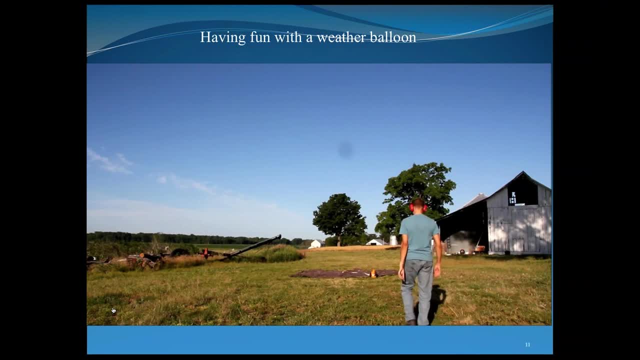 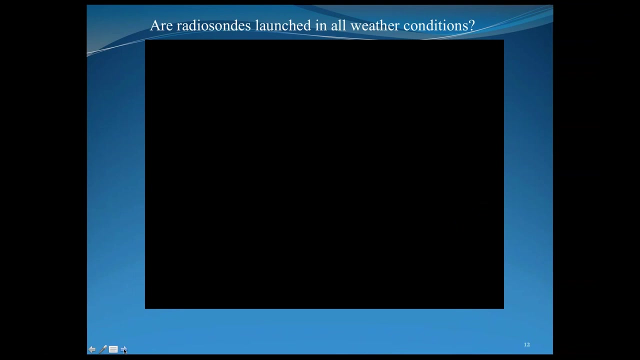 flight to visit grandma. it's probably not a UFO, it's just a weather balloon. now you may wonder our radio songs launched in all weather conditions. to give you an appreciation of what weather observers have to deal with the times, I just want you to consider the short video clip of a song that was played in the weather balloon. 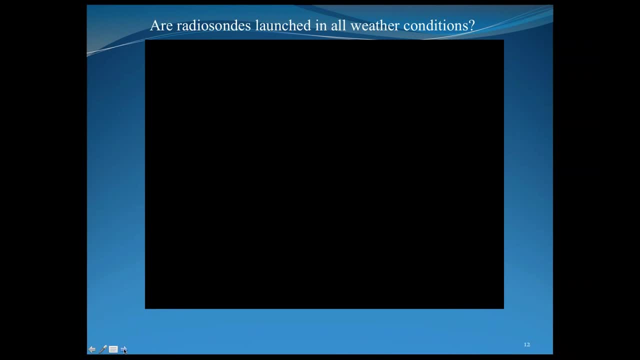 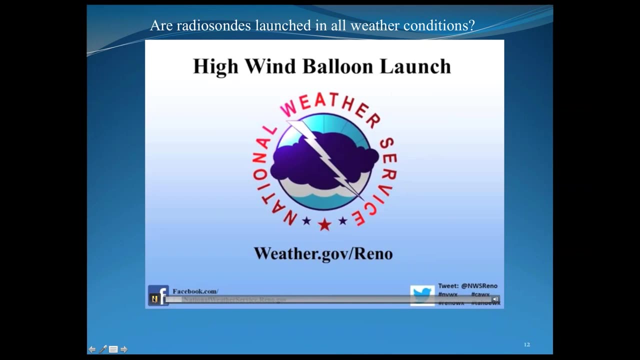 I just want you to consider the short video clip of a song that was played in the weather balloon. I just want you to consider the short video clip of a song that was played in the weather balloon, launched in windy conditions. one of the meteorologists with the National Weather Service forecast office. 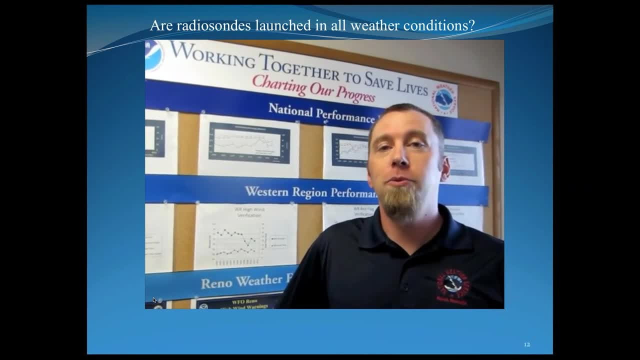 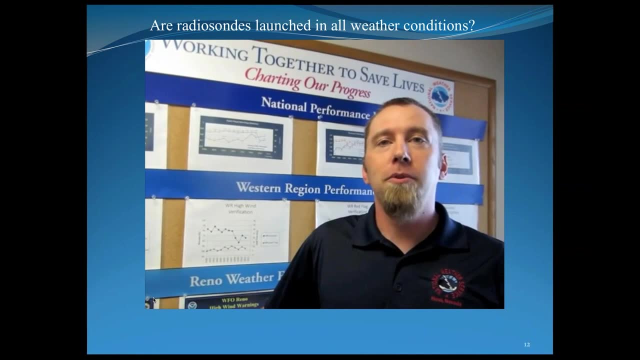 here in Reno, Nevada, every day, we launched two weather balloons, one at 3 am and 1 at 3 pm, as a part of the National atmospheric sounding program. weather balloons are launched all over the globe at the same time to create a 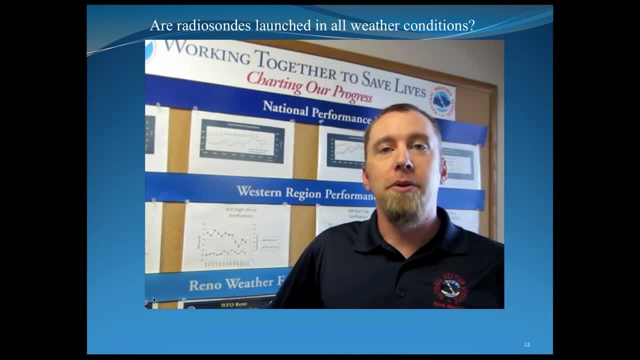 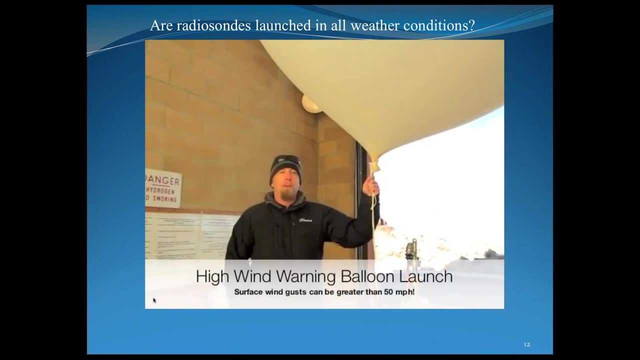 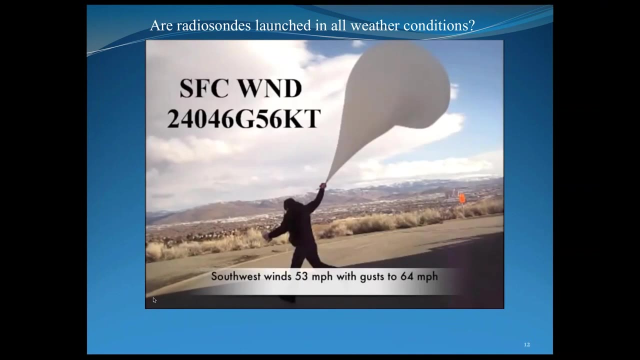 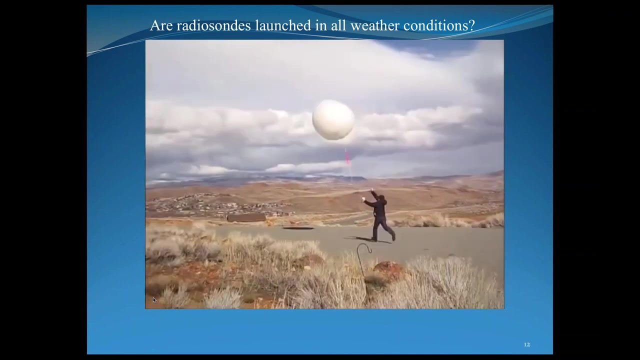 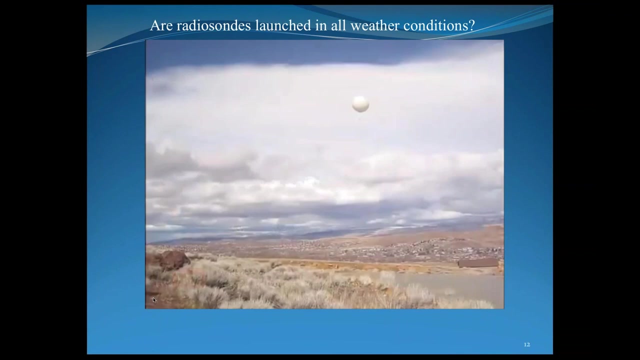 snapshot of the atmosphere. the data that we obtained is used directly by our forecasters and used to create new weather forecast models: launching the balloon during a high-wind warning, where gusts up to 50 miles an hour are possible. so fun stuff. in fact. radio songs are launched. 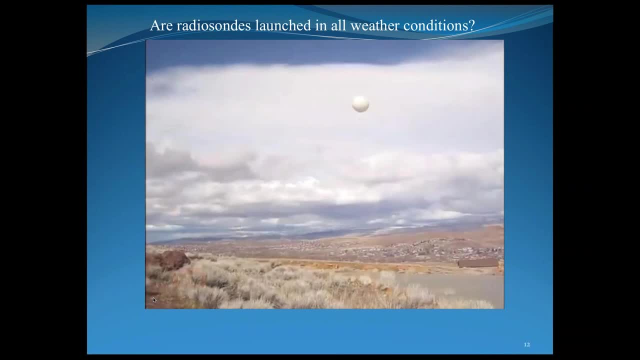 in the weather forecast models. so fun stuff, in fact. radio songs are launched in the weather forecast models. so fun stuff, in fact. radio songs are launched in all weather conditions: rain, snow, blizzards, hurricanes. there is only one in all weather conditions: rain, snow, blizzards, hurricanes. there is only one. 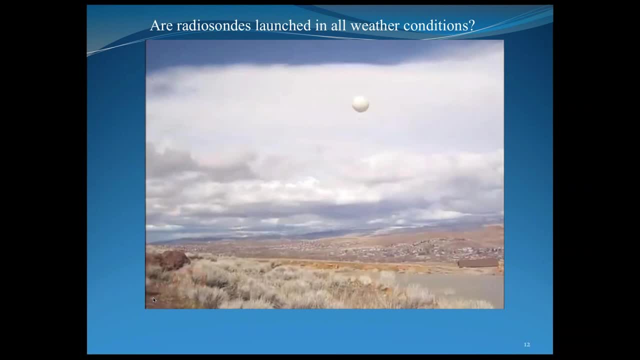 exception: if thunder is heard within 15 minutes of the launch time by the observer, the observer must wait until the threat of lightning has passed. I was visiting a weather station in Taiwan which was located on its east coast. now Taiwan is a magnet for hurricanes and on the average, 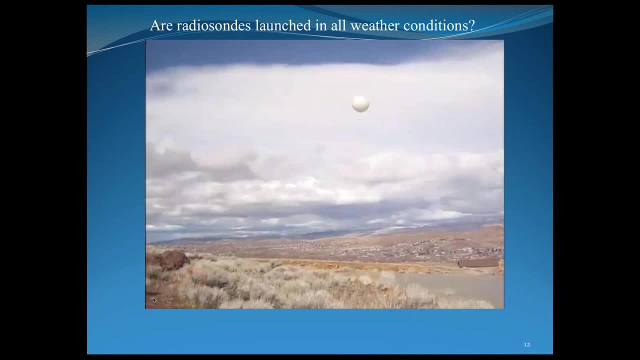 Taiwan is a magnet for hurricanes and, on the average, Taiwan is hit with three hurricanes. Taiwan is hit with three hurricanes each year. now, keep in mind that hurricanes in this part of the world, in the Far East, are called typhoons, so I asked the weather observers at this site. 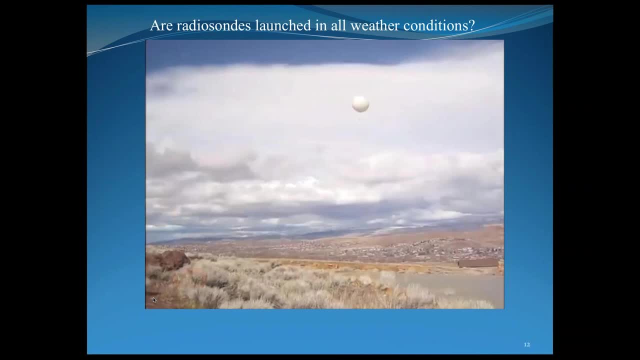 if they stopped doing their song launches when the typhoon is approaching, because In fact they increase their sound launches to four times per day. But to ensure the safety of the observer, they tie a rope around their waist In case the observer starts to get picked up by the typhoon strength winds. 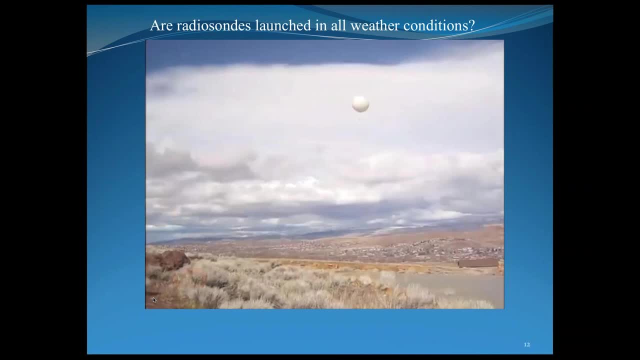 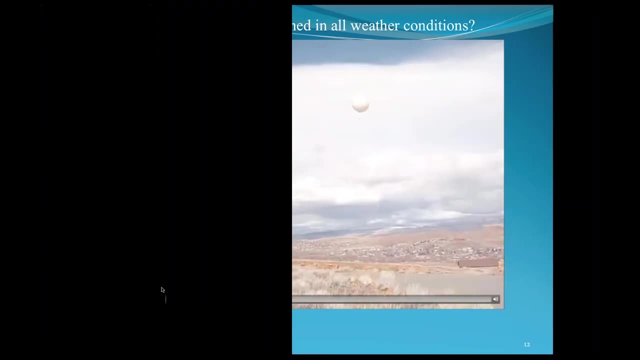 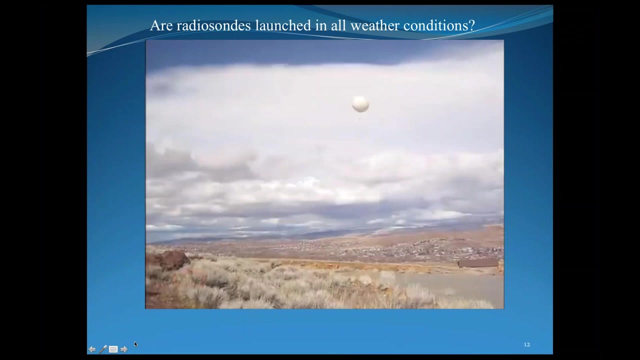 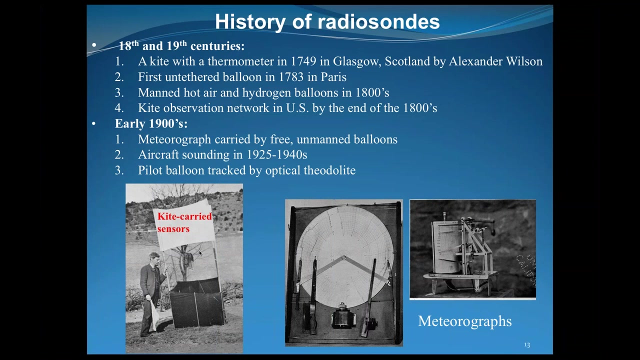 the other crew members, simply reel them back in. Now, folks, that's dedication. So I'd like to share with you now a little bit on the history of radio signs. Upper air observations began as early as 1749 in Europe with the use of a kite to carry a thermometer aloft. 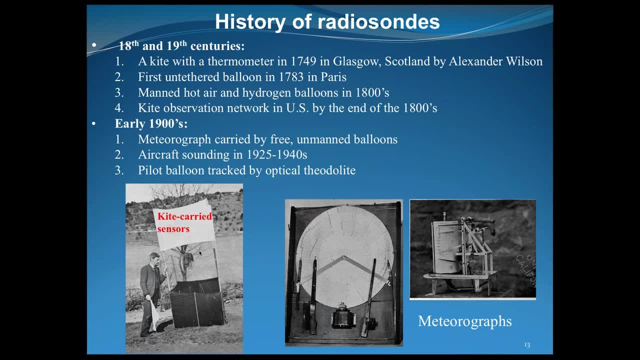 With the invention of hot air and hydrogen balloons in France in the early 1780s, scientists ascended in these balloons carrying with them barometers, thermometers and other instruments to investigate the structure of the upper atmosphere. But these manned flights? they continued through the 1800s. 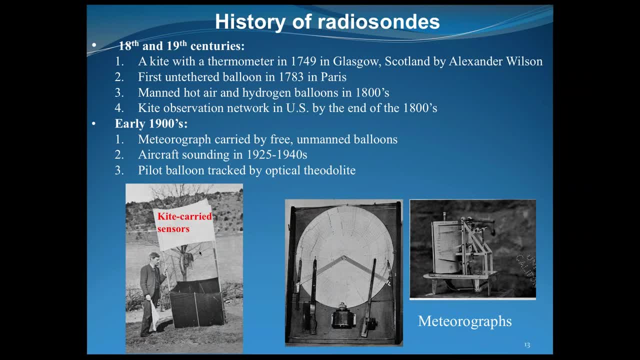 but there were some troubles that the observers ran into because of the extreme cold and lack of oxygen they experienced at the higher altitudes. In fact, in a flight taken over Europe in 1875, two Frenchmen died as a result of the high altitudes. 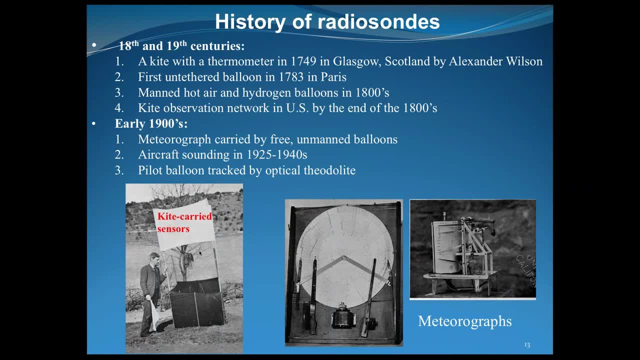 This was the result of inadequate breathing equipment. Meanwhile, the use of kites for observing the upper atmosphere continued, And by the end of the 1800s, kite observation stations were established across the US. These kites carried meteor graphs. 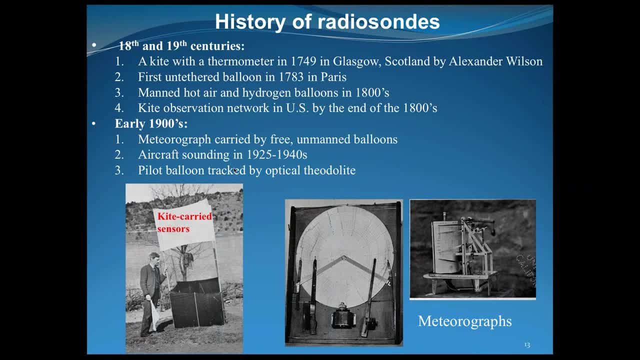 These are basically instruments that record pressure, temperature and relative humidity on a clockwork-driven chart recorder, And I have a few pictures of some of these earlier meteor graphs that were carried on balloons in these kites In the early 1900s. 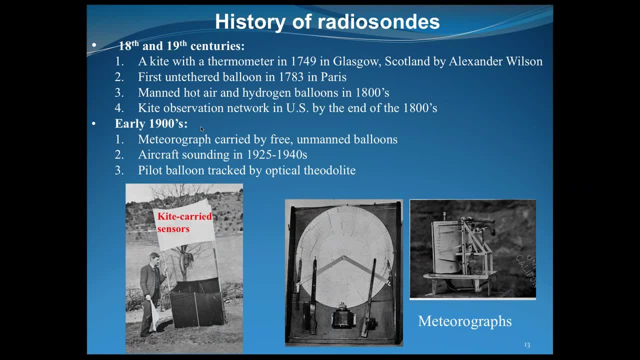 meteor graphs had developed to the point where they could be carried aloft by unmanned balloons, which reached greater heights than the manned balloons or the kites. After the balloon burst, the meteor graph returned to the Earth and it preserved the data until the meteor graph was found. 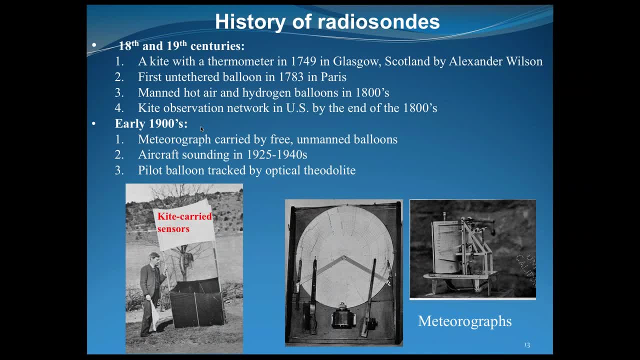 A major drawback to this approach was that the data was not readily available to the weather forecaster until the meteor graph was found, And in many cases, the meteor graphs were never found. From about 1925 through the 1940s, the Weather Bureau operated a network of up to 30 stations across the country. 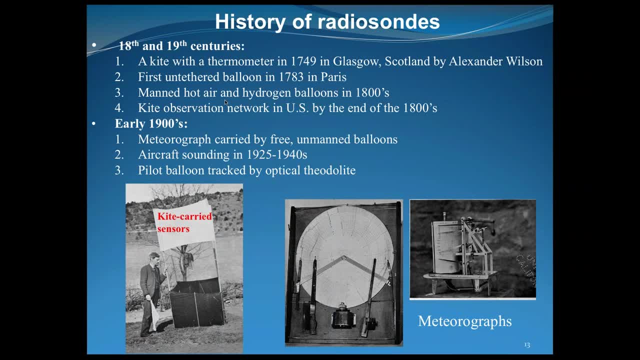 that collected weather observations taken by aircrafts. The limitations to this approach, like the kite, was that the aircraft could not be flown in poor weather and that the data could not be analyzed until the plane landed. Also, the maximum altitude of these early flights was only about 5 kilometers. 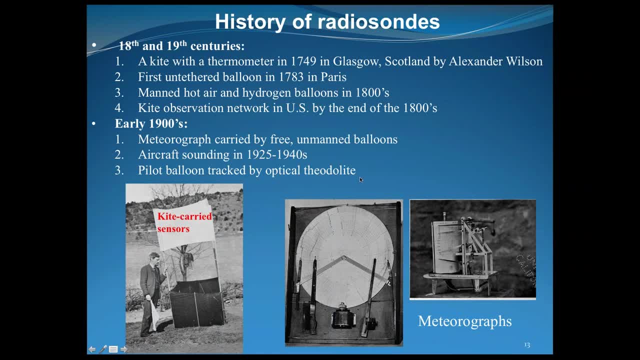 To supplement the kite and aircraft observations, the US Weather Bureau stations in 1909 began to track small balloons, called pilot balloons, by optical theodolites to obtain information about winds above the surface. I'm going to talk more about that in the next slide. 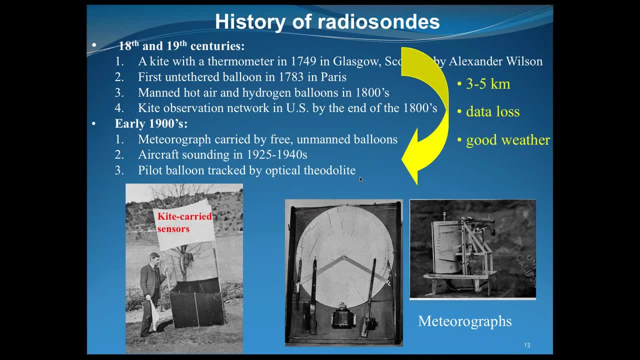 But basically the early years had several shortcomings. The data was only at the lowest levels, only up to 3 to 5 kilometers. There was a lot of data loss and the data was only in good weather conditions. When you want to make a forecast, you'd like to know the weather. 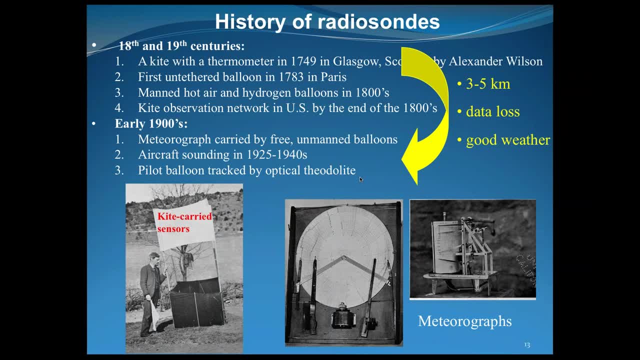 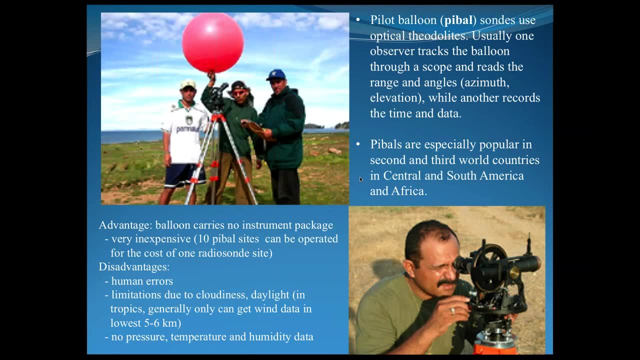 when the weather is changing and the weather is getting bad. So I mentioned in the last slide about pieball observations and I wanted to follow up on this because this type of observation is still quite popular today in second and third world countries. 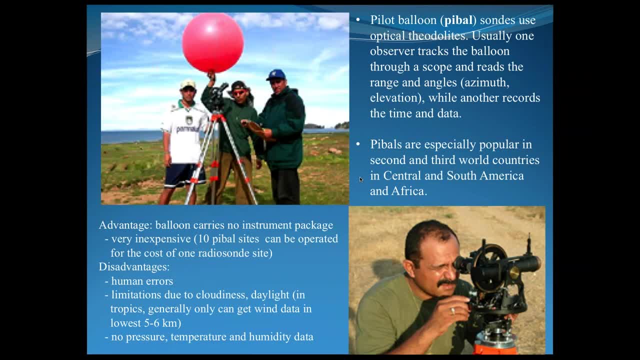 especially in Central and South America and in Africa. So I wanted to take a minute to explain them better. Pilot balloons, or pieballs for short. these observations are taken with a radial theodolite, So in the lower right-hand corner. 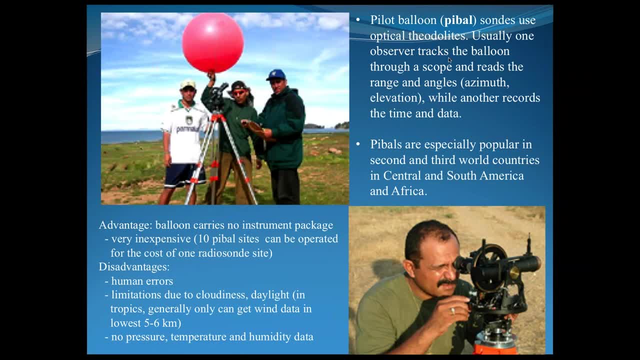 you could see someone looking through one of these theodolites And they're keeping this balloon and they usually use these small red balloons. he's keeping that balloon in the scope of this theodolite And he reads on this instrument: the angles. 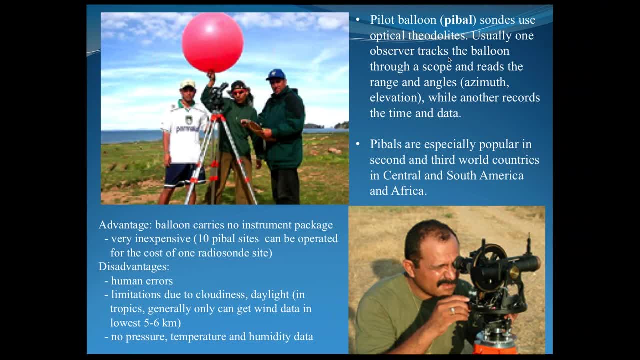 the azimuth and elevation angles, And another person then records this information and records the time, And with this information you can actually back out the winds, because it tells you the location of the balloon, how it changes in time. So the advantage of these type of soundings: 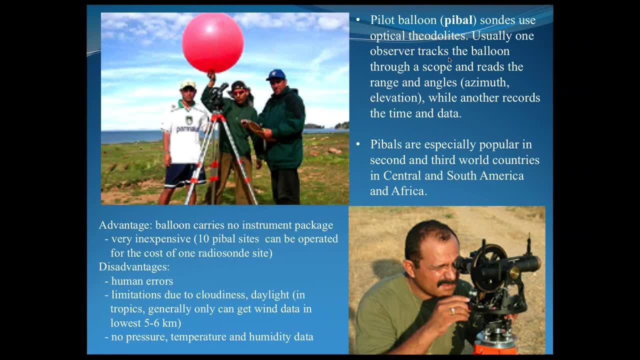 is that the balloon. it carries no instrument package, so it's very inexpensive. Ten pieball sites can be operated for the cost of one radius on site. So that's why second and third world countries- this is a popular way to take observations. 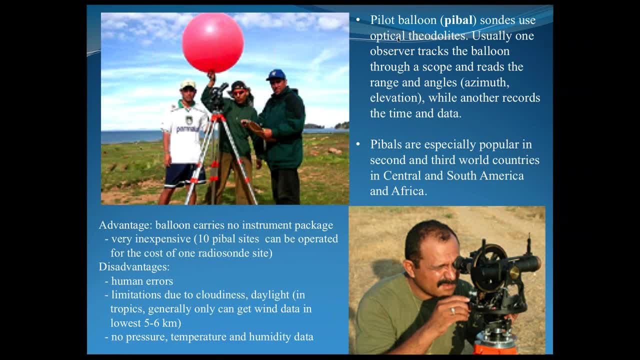 The disadvantages of this are: there are human errors trying to keep the balloon in the site. If it goes behind a cloud, you can no longer take any observations And generally it can only be done in daylight, But some observers do do it at night. 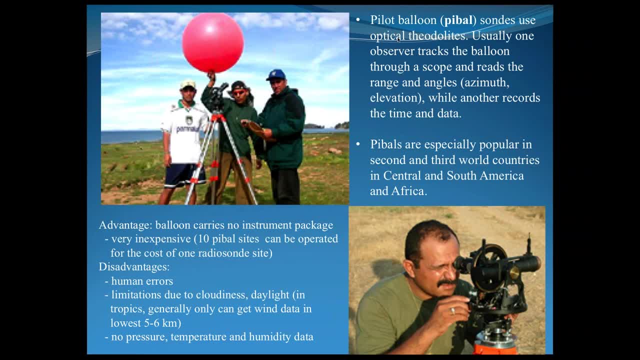 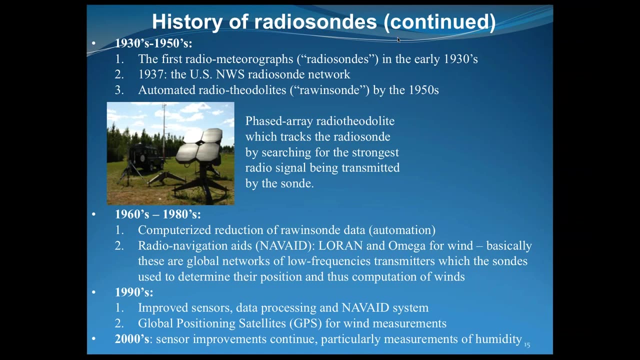 they attach a small flashlight to the balloon. So any other disadvantages. it has no temperature, pressure or humidity information. So continuing on with the history of radio sounds. because of the limitations of the earlier sounds, scientists began suspending crude radio transmitters. 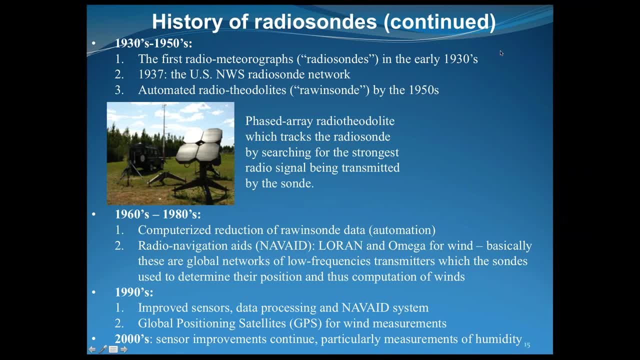 from balloons in the early 1930s, And these became the first radio meteor graphs or radio sounds that were flown. In 1937, the US Weather Bureau established a network of radio sound stations that has continued until the present day. 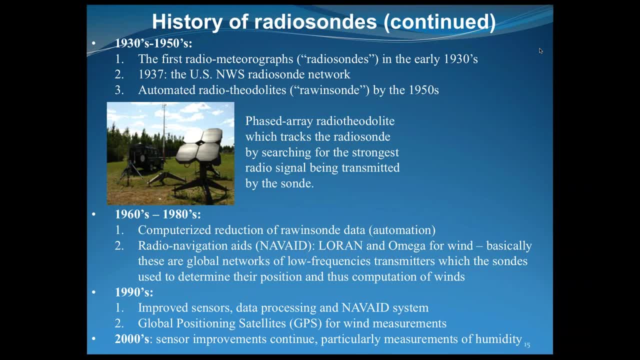 But up until now sounds only measured, basically the upper level, pressure, temperature and humidity. But during World War II advances were made in radio detection technology that allowed the radio sound to be tracked in flight so that winds aloft could be measured. 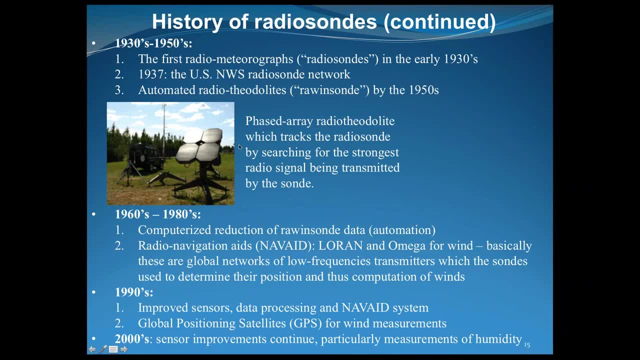 This here is a picture of a phased array, theodolite, which tracks the radio sound by searching for the strongest radio signal, and it then just transmits that information from the sound back to the ground station. So, using these types of devices, 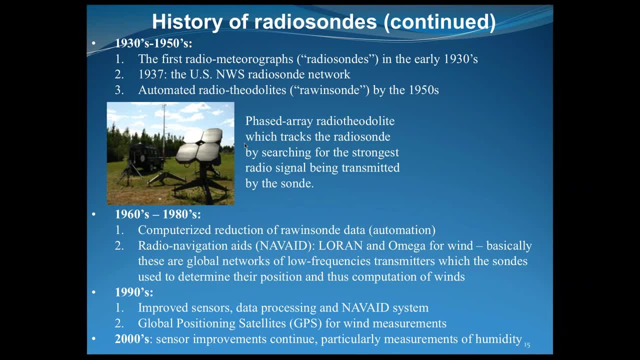 we could actually measure the upper level winds, And these devices are still used today at some stations. In the interest of time, I'll sum up the advances from the 60s to the present by saying that increased use of computers, continued refinements and improvements of the sensors. 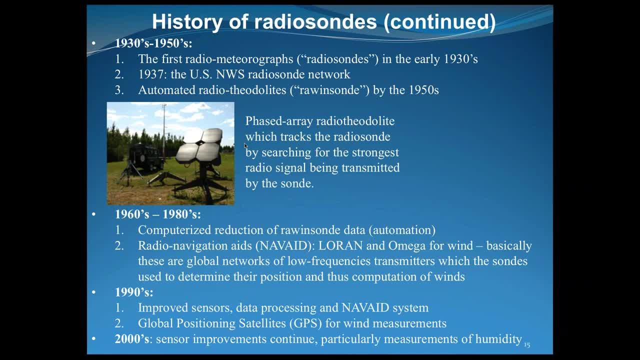 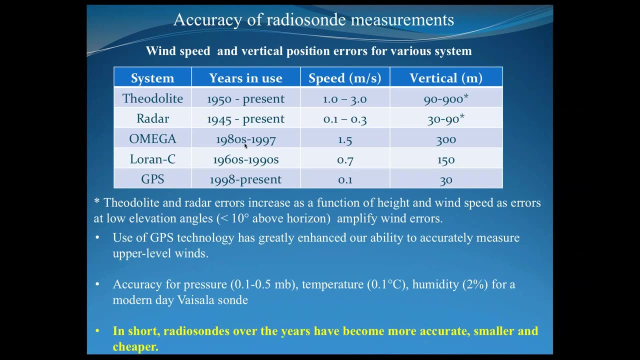 and more sophisticated navigational tracking aids, in particular the use of GPS technology, have resulted in extremely accurate instruments for measuring the characteristics of the air at upper levels. This slide shows the accuracy of radio sound measurements. This table shows the wind speed and the vertical position errors for these winds. 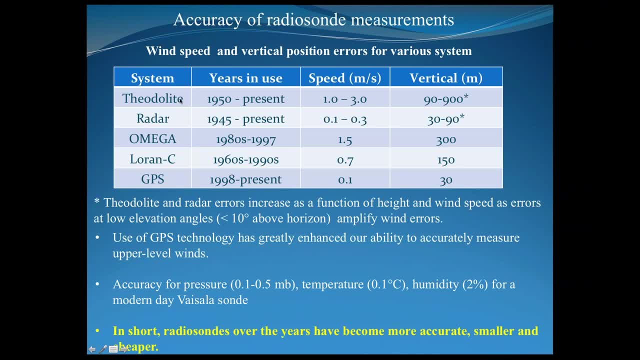 from various systems through the years. So the theodolite radar, Omega and Loran-C are different navigational systems And finally the GPS, the geostationary positioning satellites. So you can see how the errors or the accuracy 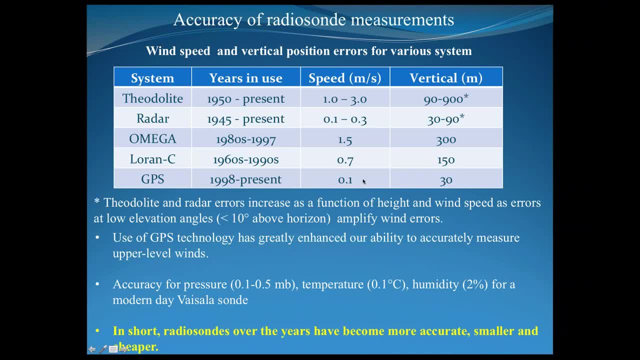 the errors have gone down and the accuracy has gone up. So now, with GPS technology, we can actually measure the winds within a tenth of a meter per second- much better than the early days- And we can estimate where that wind observation is from. 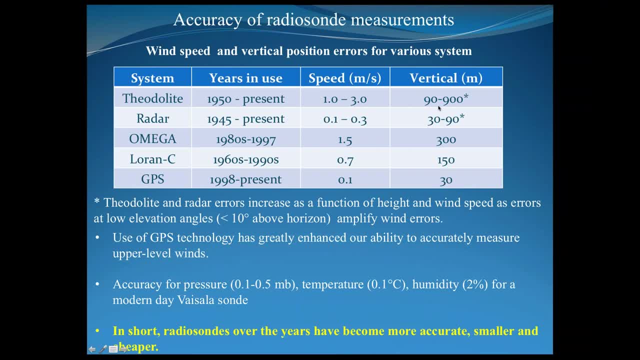 within 30 meters, where within the early days, 900 meters or a kilometer was the best we could do. So the use of GPS technology has greatly enhanced our ability to accurately measure upper level winds. Now the accuracy for pressure is from a tenth to half a millibar. 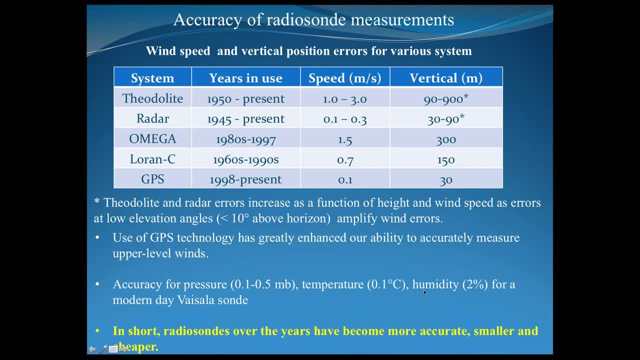 Temperature is within a tenth of a degree and humidity is two percent, And these are accuracies reported from a modern day by Solaceon. So, in short, radio sounds over the years have become much more accurate, smaller and cheaper. So how cheap are they? 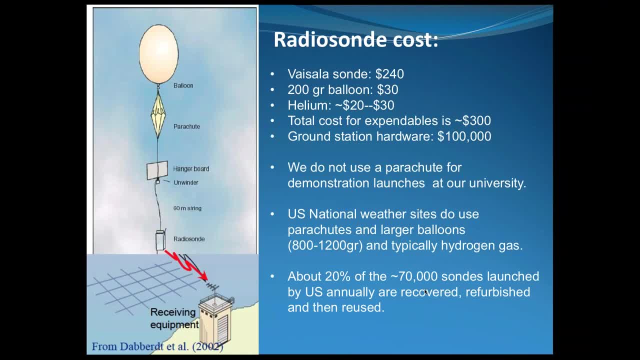 Not all that cheap. This slide summarizes what the cost of the expendables are. So this is for the system that we use in the department. These are the costs. The radio sound itself costs about $240.. The balloon: a 200 gram balloon. 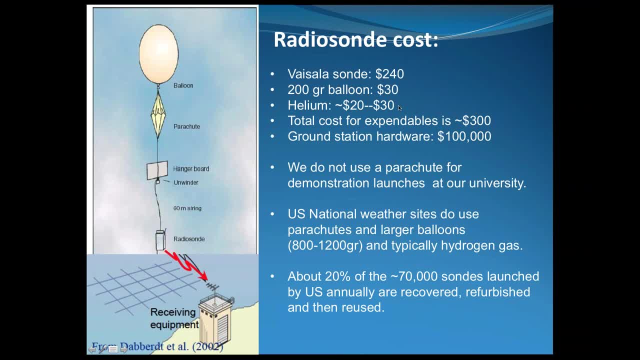 that we use is $30.. And the helium that we use per launch is $20 to $30.. So the total cost for the expendables in one launch is about $300.. The ground station software is $100,000.. So this diagram 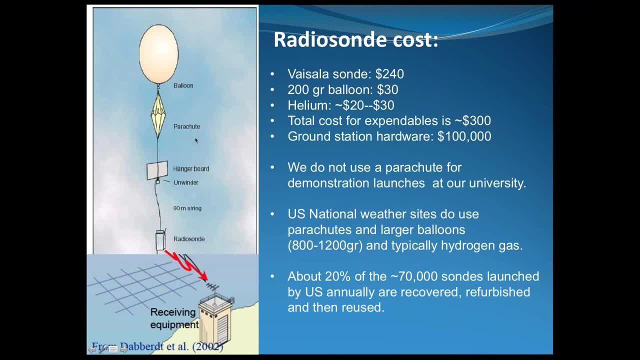 here shows a typical setup In our department: launches. we do not use a parachute. However, the National Weather Service does use a parachute. They also use larger balloons, So that's probably more expensive for them, But typically the National Weather Service 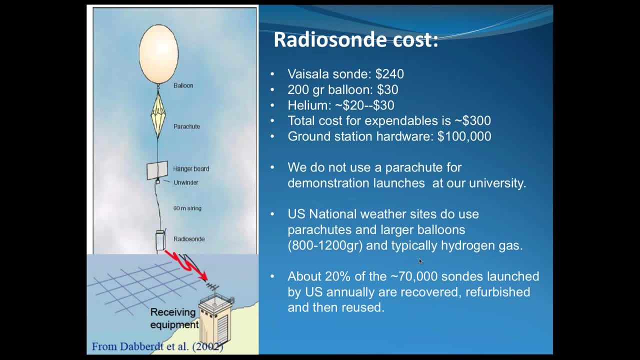 uses hydrogen gas. About 20 percent of the 70,000 sans that are launched annually by the US are recovered, refurbished and then reused. So you can see that the US- You could do the math here- The US spends about. 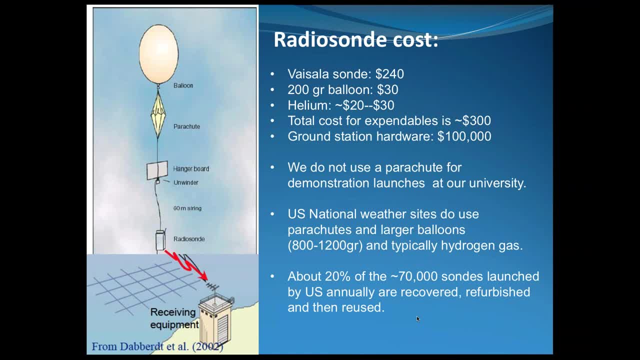 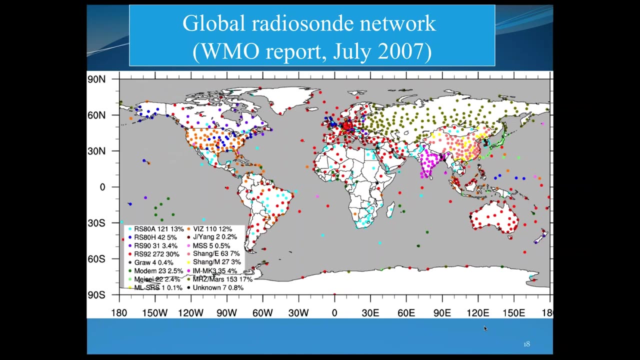 $20 million a year in expendables, But that does not include the labor cost for doing these launches. So where are these observations made? The colored dots on this map show all the locations around the globe which take radiosonde observations. The color coding: 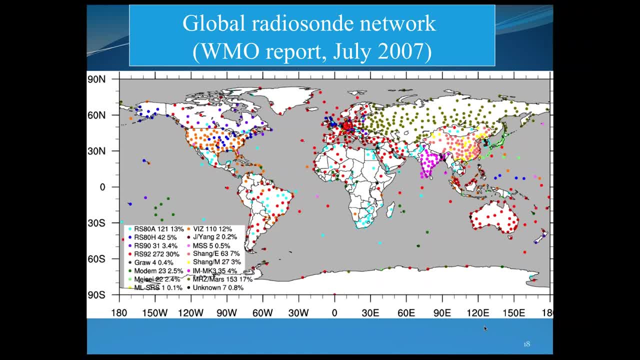 of these dots indicate the type of radiosonde that is used at each of these sites. So in total there are over 900 stations globally that take radiosonde observations daily. There's over 15 different types of radiosondes used And two. 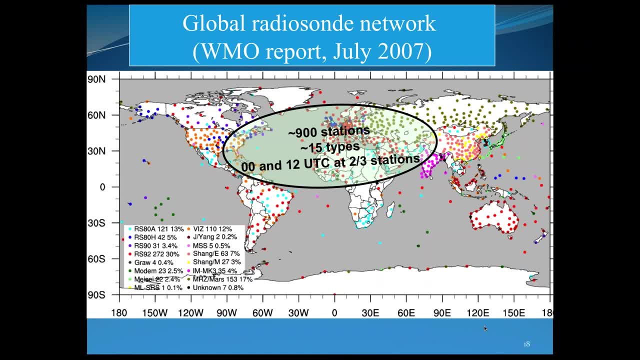 thirds of the stations take observations at 0 and 12 UTC every day. The remaining sites, because of financial considerations, take only observations once a day at 0 or 12 UTC. Also bisalisondes, which tend to be the most reliable type. 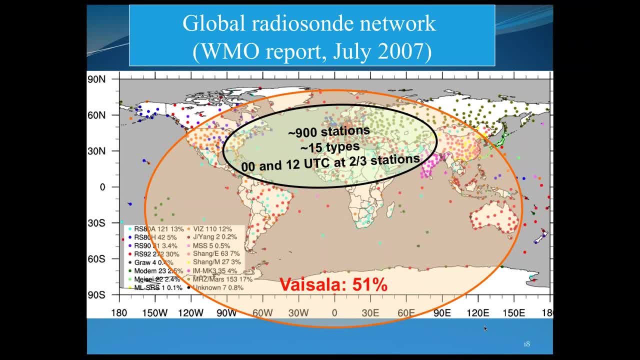 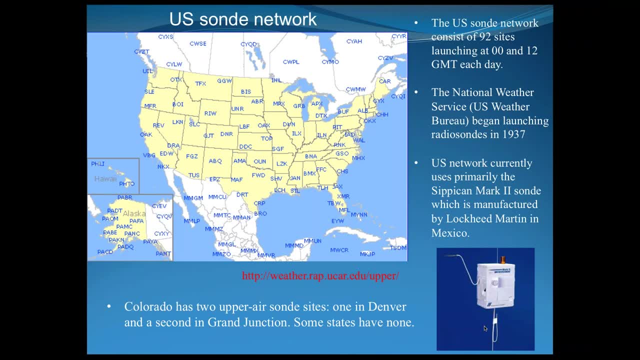 are used at 51% of the sites around the globe. This map shows the US sounding network. The US network consists of 92 sites launching sondes, again at 0 and 12 UTC. However, if there's a high-packed weather, 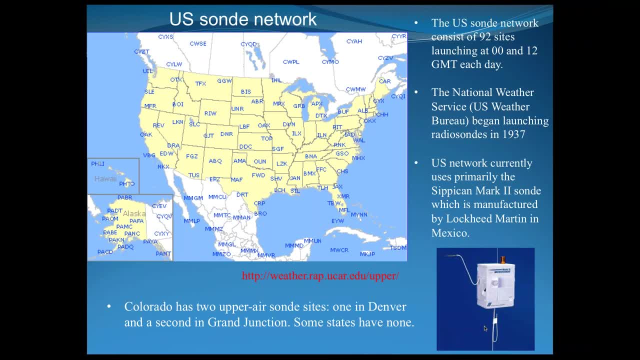 event occurring like a hurricane approaching the east coast of the US or maybe a huge winter storm that's forming that will impact holiday weather plans. the weather service can request additional observations be made. These are typically made at 06 and 18. 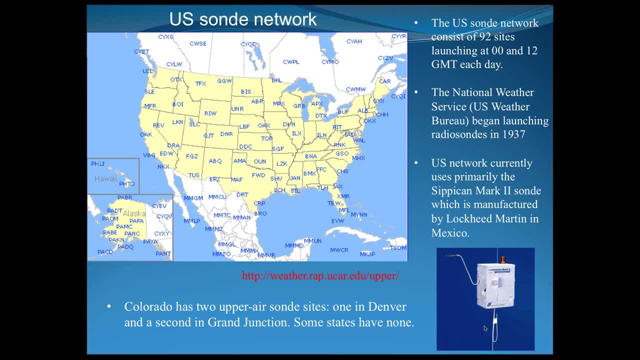 UTC. This additional data can help reduce the uncertainty in the forecast for these high-impact weather events. So currently, the US network primarily uses the Sipicant Mark II sonde, which is manufactured by Lockheed Martin in Mexico. This map: 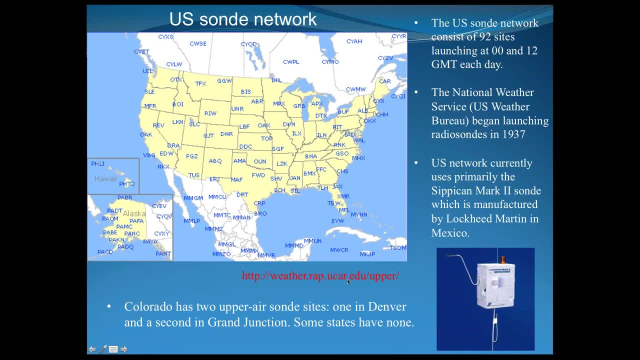 comes from this website. I show the link here And if you go to this map, you can click on any one of these hot links, any one of these sites, and you could see what the current radio sound observations are for that site Now, Colorado. 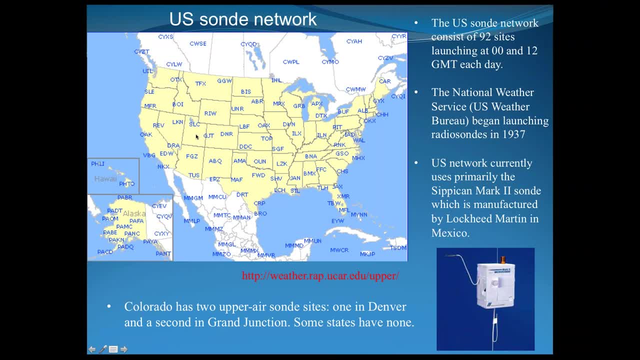 has, where we're located, has two upper air sound sites, one in Denver and one in Grand Junction. Some states have none. For example, Indiana, Kentucky and a number of sites in the northeast have no upper air sites. So now I'd like to try to answer. 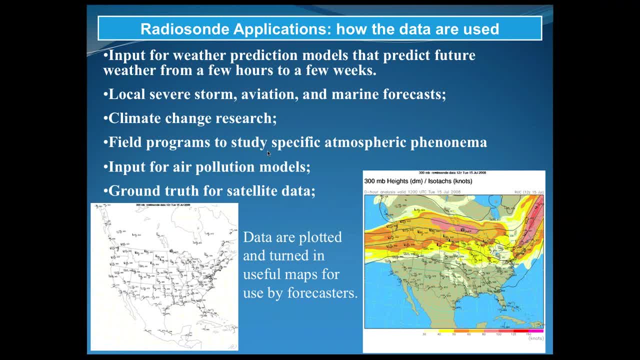 the question: how are the radio sound data used? As I mentioned earlier, one of the primary uses of these data are input for weather prediction models that predict the weather anywhere from a few hours to a few weeks into the future. Radio sound data is also used to 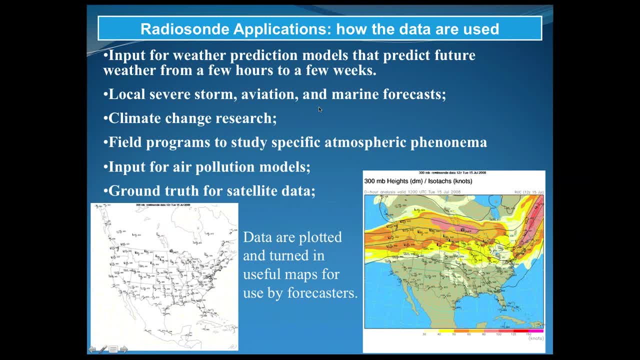 for local, severe storm, aviation and marine forecasts. It's used in climate change research Field programs use radio sound data to study specific atmospheric phenomenon, For example, if we want to better understand how tornadoes form in the Great Plains or we want to investigate the disturbance. 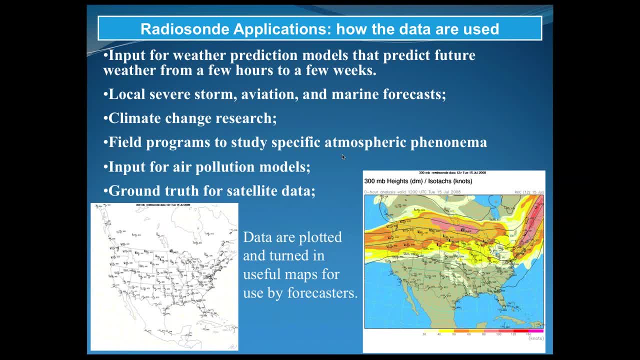 that comes off the coast of Africa which develop into hurricanes. we'll plan an experiment which uses a radio sound network to try to investigate those atmospheric phenomena. Radio sound data is also used for air pollution models and ground truth. for satellite data It's probably 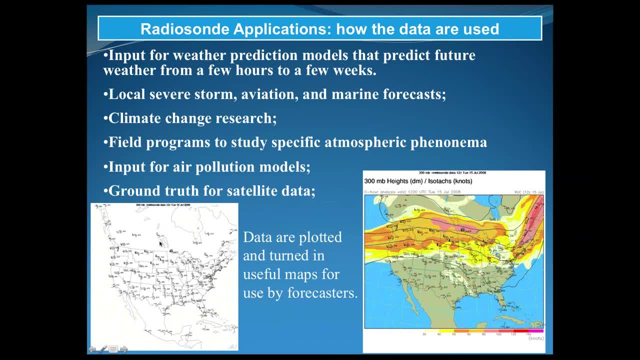 hard to see, but here at the bottom is a map of upper level winds and other data plotted over the US which shows where the jet stream is located. The map on the left shows the raw data. This is again at 300 millibars or about 9 kilometers. 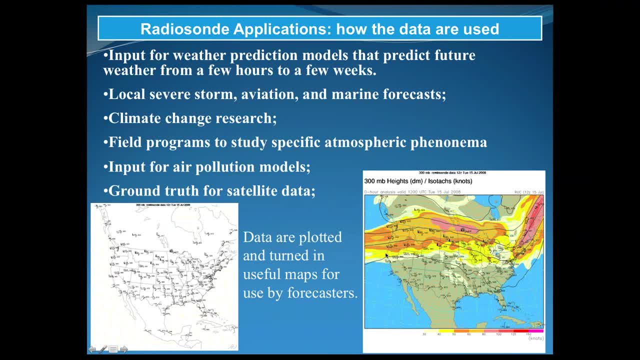 The map on the right shows this data analyzed Where we see these warm colors? this is actually an analysis of the jet stream. Maps like this are invaluable to forecasters, as wind patterns aloft often determine and steer the weather systems at the surface. 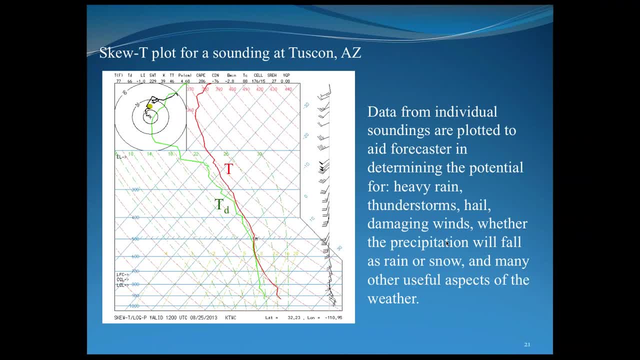 Forecasters often like to display a radio sound data. this is just for one radio sound launch in a format that's called a SQT plot. I'm showing here a SQT sounding for Tucson. I think this is sometime in the summer of 2013.. 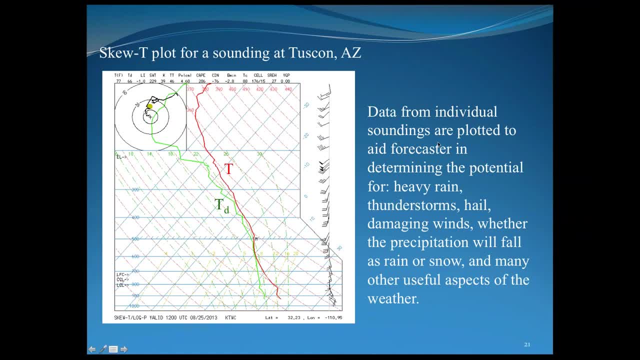 Here. the red curve on this plot shows the temperature and the green curve shows the dewpoint, And where these two lines come together, the relative humidity is 100% and that's where you'll find cloud layers. Now plotting the data in this format. 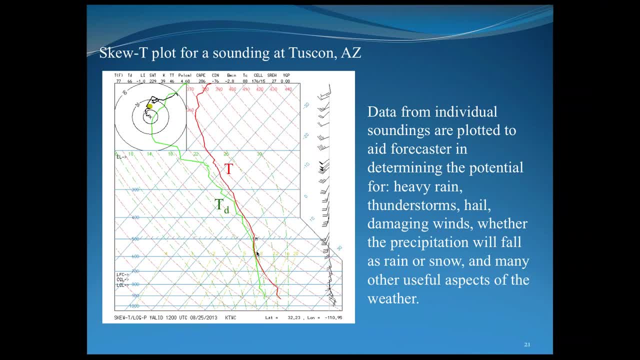 it allows the forecaster to determine the potential for many things like heavy rain- how much rain potential is there- thunderstorms, whether it be hail, damaging winds, whether precipitation will fall as rain or snow, and many other useful aspects of the weather. 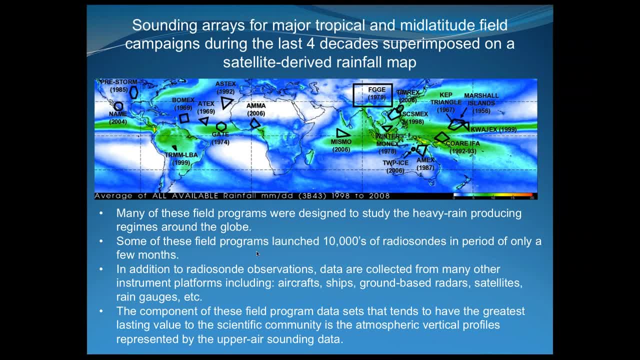 As I mentioned earlier, radio sounds are used in field programs and this slide shows the sounding are raised for major tropical and mid-latitude field campaigns during the last four decades, And I've superimposed this on a map of satellite-derived rainfall map. 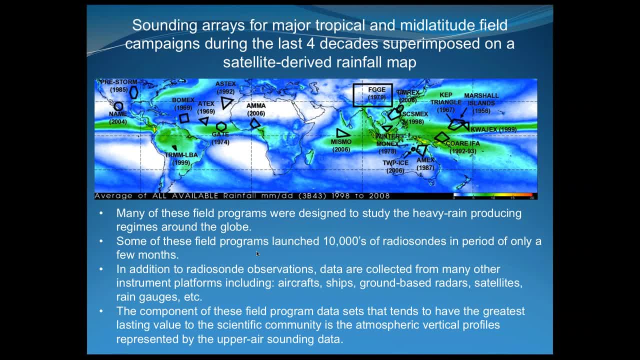 So the areas in this map that are shaded in green are experienced on the mean. This is a mean map of where rainfall is the heaviest, So you can see it's typically in the tropics, in areas like the Amazon. So the vertices. 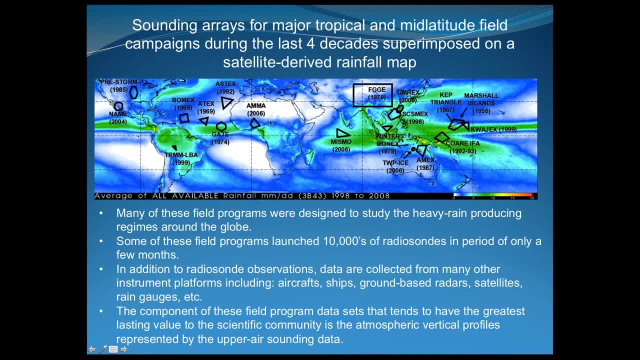 of all these polygons. each of these polygons represents a sounding array for an experiment, But the vertices of these polygons show where radio sound launches were made during these experiments. Many of the sites were from ships or tiny islands. So many of these field. 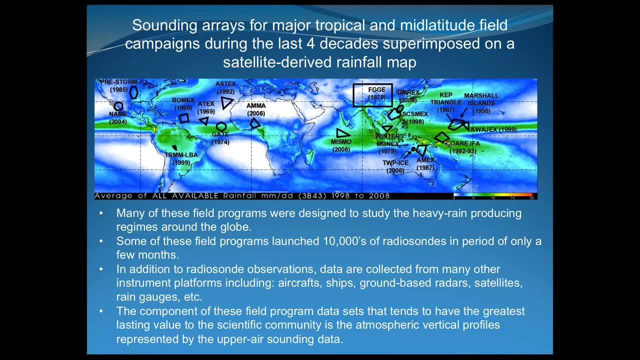 programs were designed to study the heavy rain producing regimes around the globe, And I like the way one scientist put it. He said these observational networks are intended to capture, to study and to understand the invisible atmospheric creatures that exist in that region of the world. 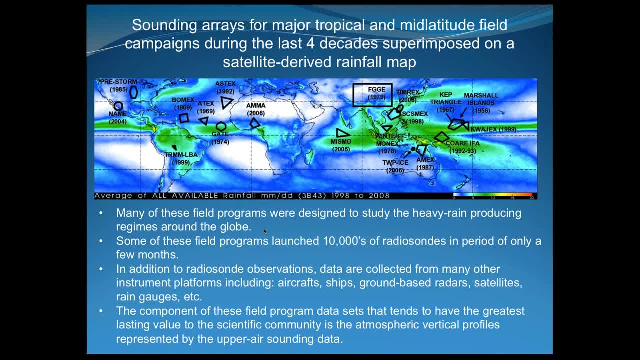 And with these experiments we have been able to capture many interesting of these invisible atmospheric creatures. So some of these field programs that I've been involved with- for example Toga Core here in 1992 and 93, they've launched over 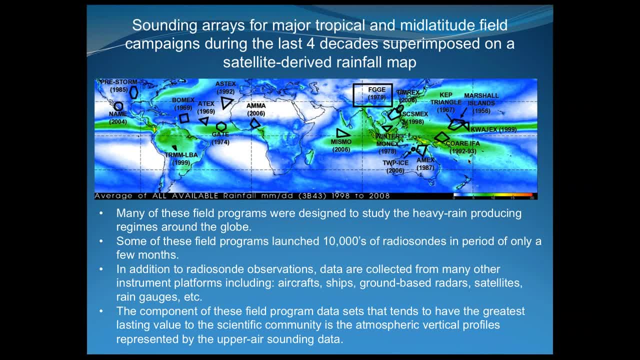 tens of thousands of soundings in a period of only a few months. So some of the sites may be launching four to eight soundings per day. In addition to the radio sound observations, data are collected from many other platforms during these experiments: Aircrafts, ships. 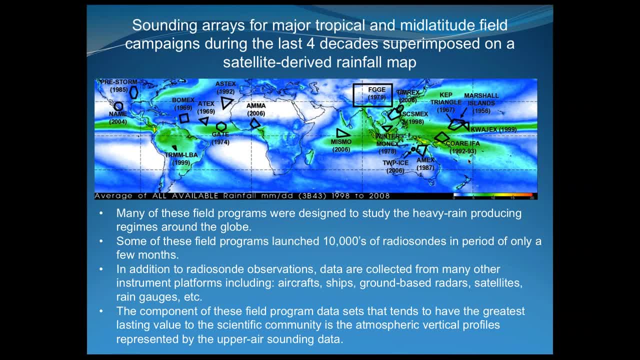 ground-based radars, satellite rain gauges, So they're all taking observations. But the component of these field program data sets that tends to have the greatest lasting value to the scientific community. it is the vertical profiles of the atmosphere represented by the 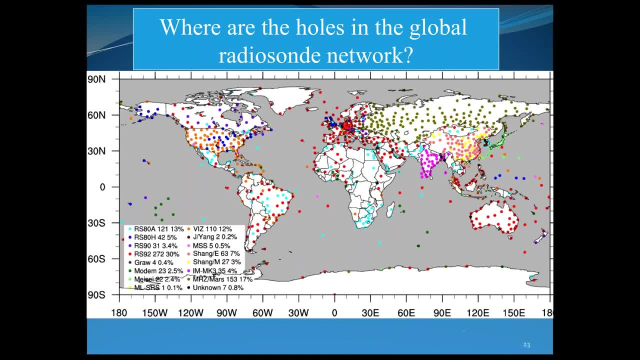 upper air sounding data set. So look at this map here. I've shown this map before. This is the map of where radio sound launches take place over the whole globe, But I want you now to look at it and see where are the holes in this. 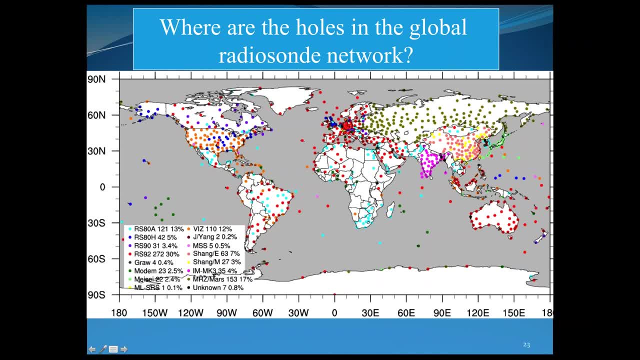 global network, Your eyes might be drawn to places like Greenland, the Arctic, the Antarctic, but also over the oceans. So what do we do? How do we fill in these data gaps? These data gaps are important, For example, right now. 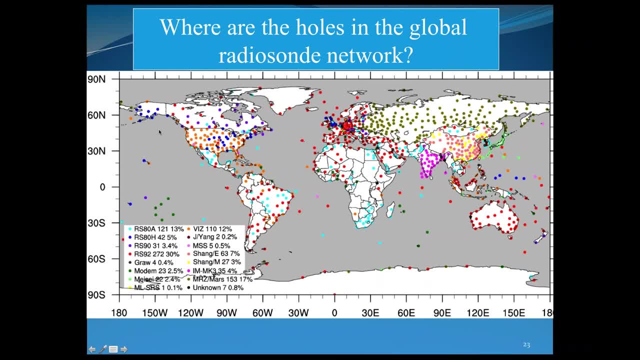 there's a big, major storm which is coming off the west coast of the United States And, if you remember, at mid-latitudes storm systems tend to move from west to east, So we have almost no radio sound data in this region. So how do 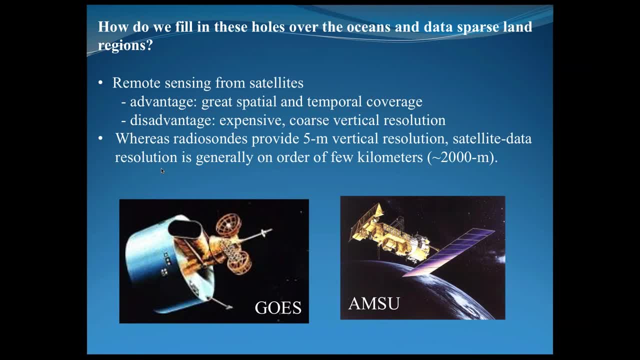 we fill in these data gaps. Well, remote sensing from satellite helps us to fill in these data gaps. The advantage of this is they have great spatial and temporal coverage. They cover the whole globe And we get data every half an hour to hour from these. 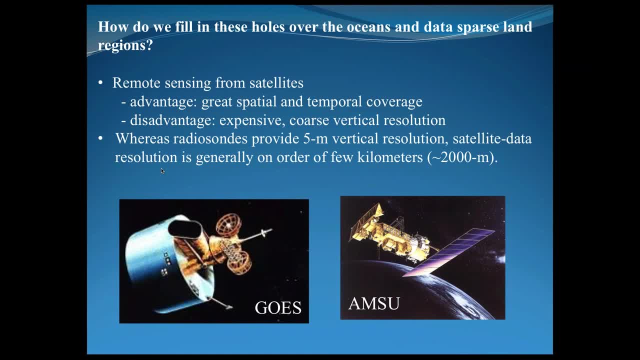 satellites. The disadvantage is they're expensive. Satellites cost an order of billions of dollars, Whereas radio sound networks on the order of millions. Also, satellites have coarse vertical resolution of the atmosphere. Radio sounds provide resolution on the order of five meters, Whereas satellite the resolution. 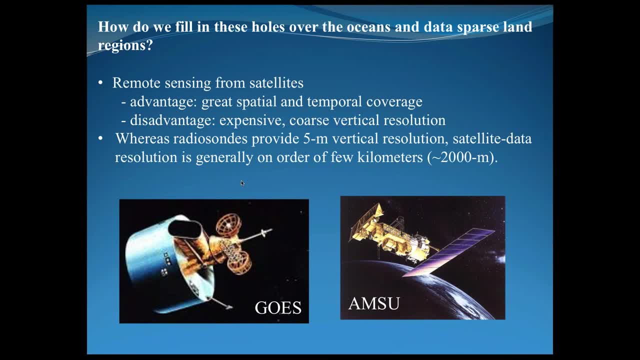 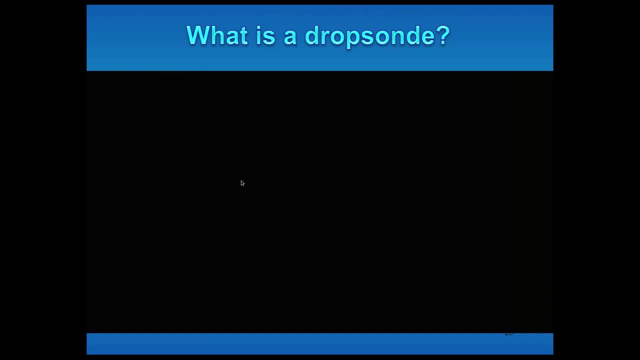 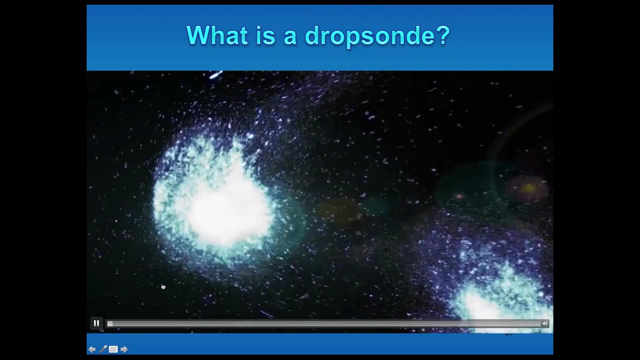 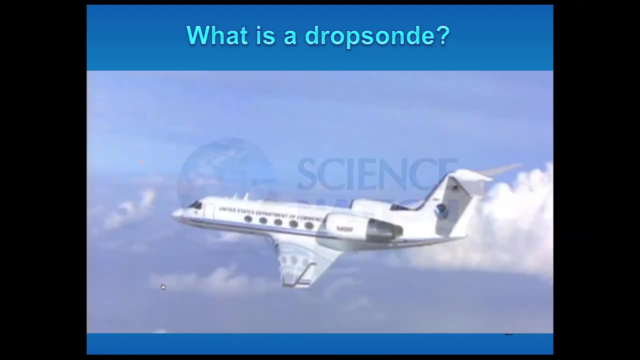 is generally on the order of a few kilometers, So we need to plug in these data gaps in other ways. One of these ways is with drop sounds, And the concept of drop sounds is explained nicely in this video. This small cylinder is called a drop. 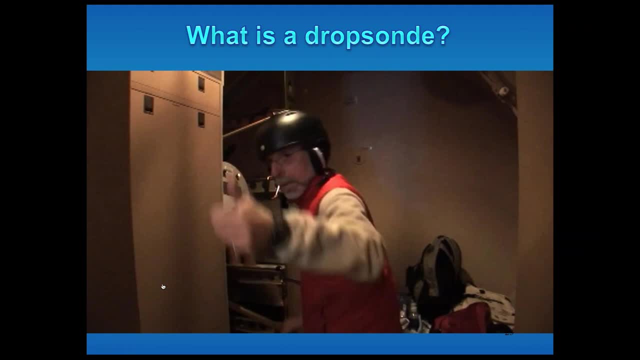 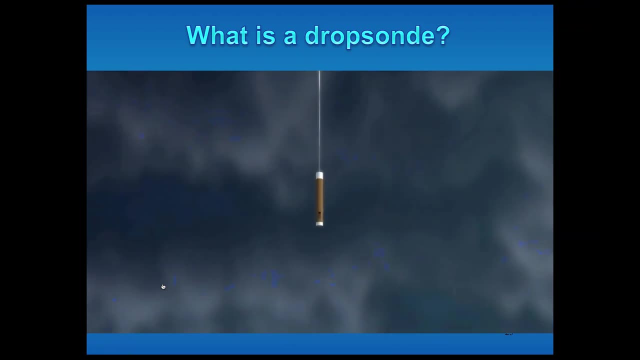 sound, or sound for short, And what a story it tells. It launches from an aircraft and falls through the air, gathering data about the atmosphere as it descends. It's a workhorse of hurricane forecasting, dropping out of hurricane hunter airplanes right into a 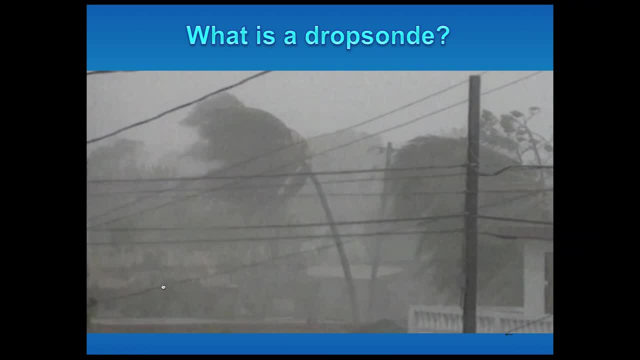 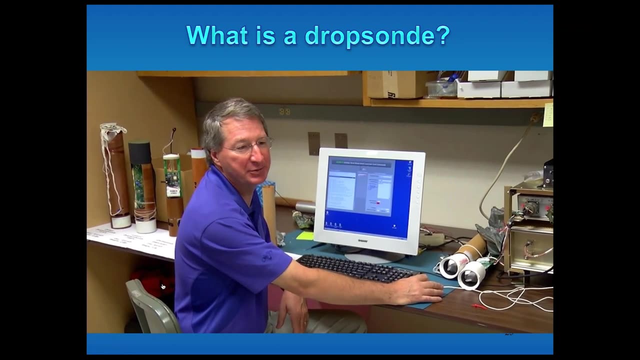 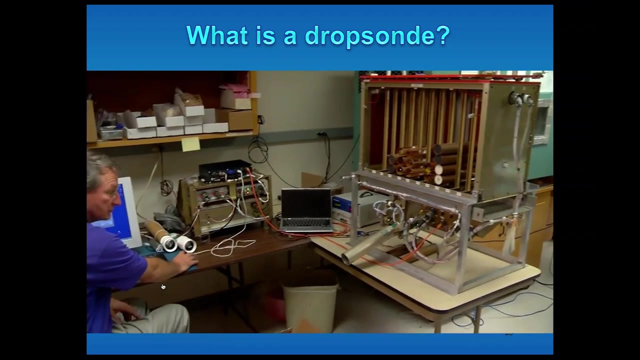 raging storm. Drop sounds have a huge impact on understanding hurricanes and predicting hurricanes. Electrical engineer Terry Hoke and colleagues at NCAR, the National Center for Atmospheric Research, have been designing, building and improving drop sound technology for more than 30 years for a wide range. 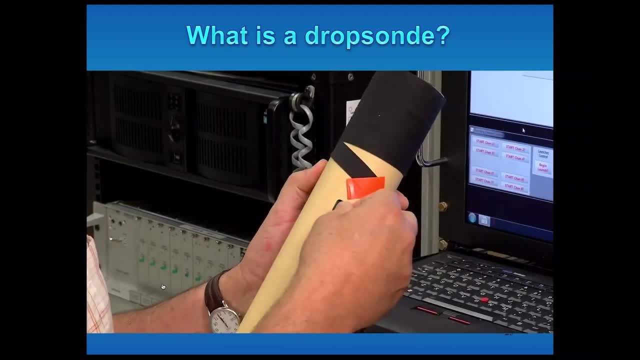 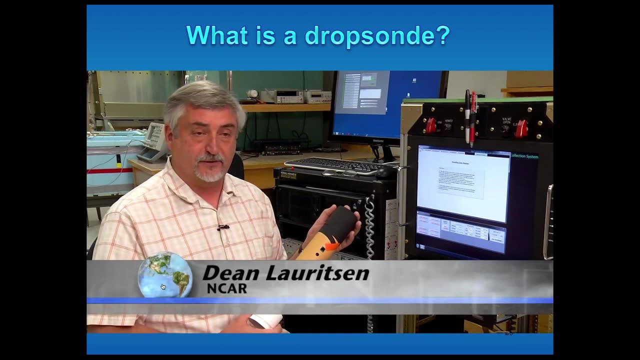 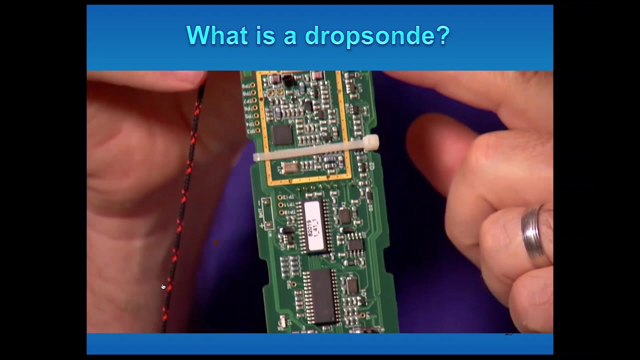 of applications. This is the drop sound that the NSF aircraft used for our scientific research purposes, and it's also sensibly used by the hurricane research people. Compared to earlier models, today's sounds are lighter weight, relatively inexpensive and loaded with sensors. 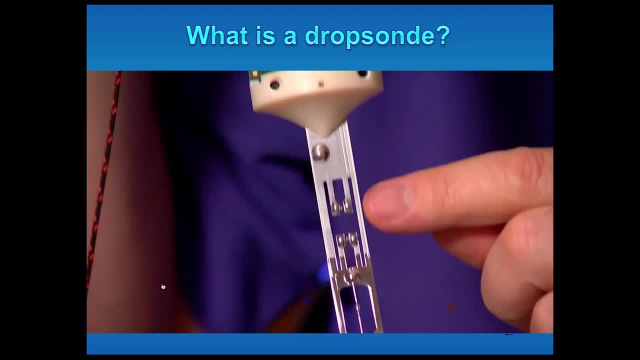 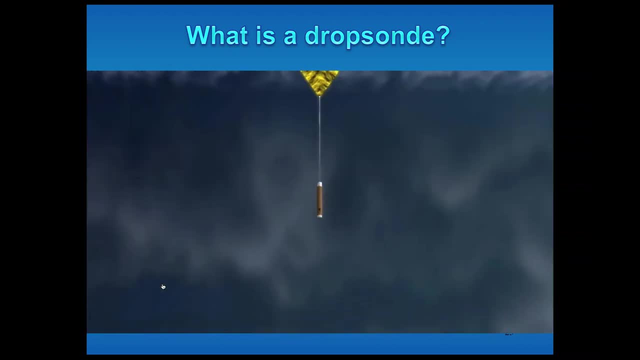 We actually have a temperature and humidity sensors down here at the bottom and we also have a parachute here at the top end of it. As it falls, the drop sound checks the pulse of its surroundings two times a second, including pressure, temperature, humidity. 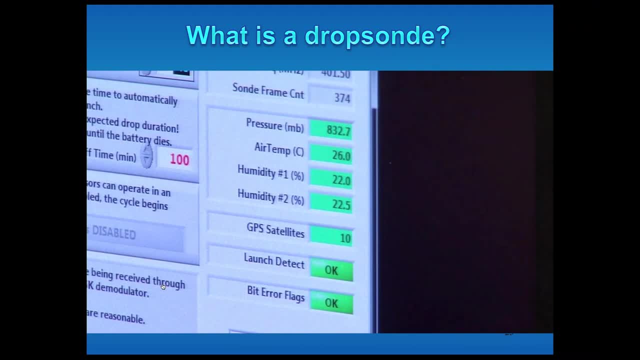 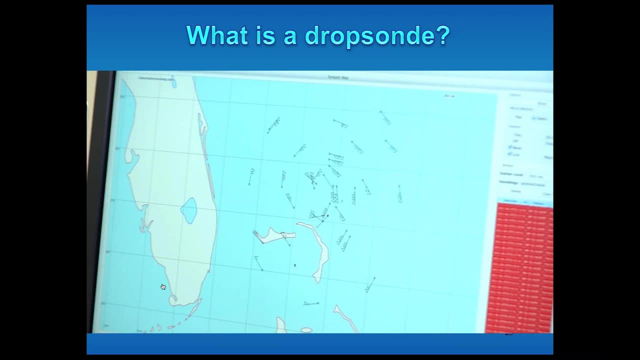 wind speed and wind direction. We're just taking these vertical slices of the atmosphere constantly as the sound falls, You can see how the winds are in a circular pattern going around the hurricane, so the center of the hurricane is going to be in here. 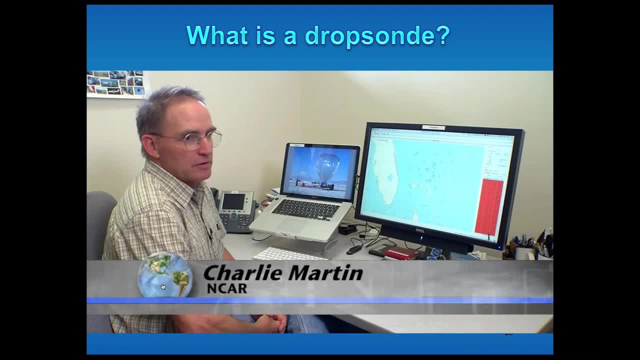 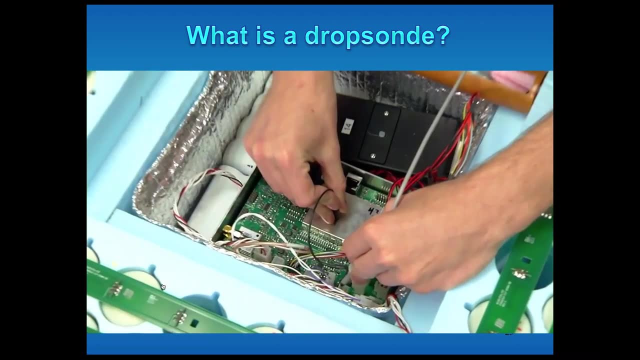 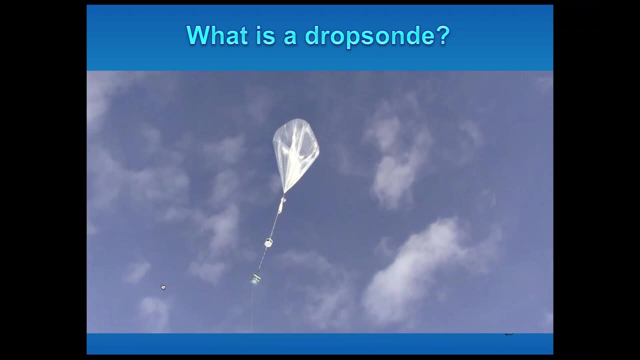 And they use this data, along with other data, to classify the. hurricane Hoke and his team custom-fit aircraft with sound launchers, including this one for helium-filled balloons. In 2010,, American and French researchers deployed balloons over Antarctica that dropped. 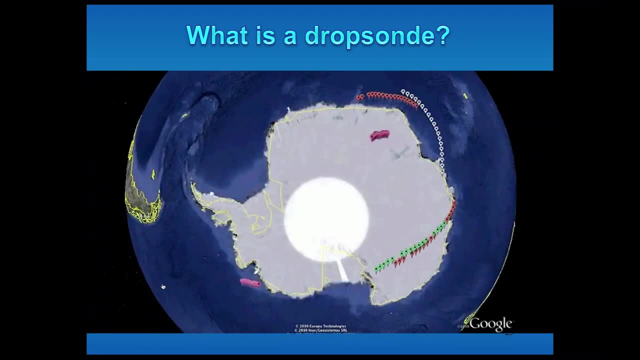 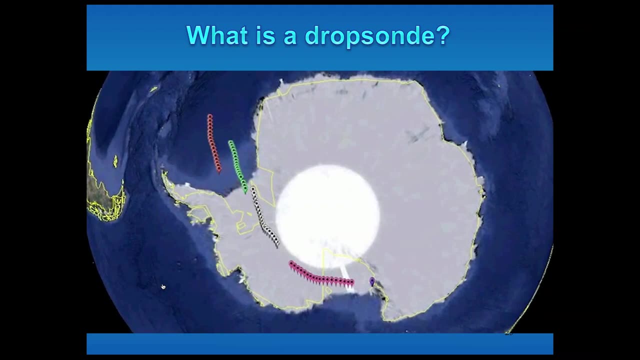 300 sondes to study atmospheric conditions and the shifting ozone layer over a four-month period. That has mapped the Antarctic atmosphere like it's never been done before. As the sonde is falling, we're seeing every single little measurement show up immediately on the computer screen. 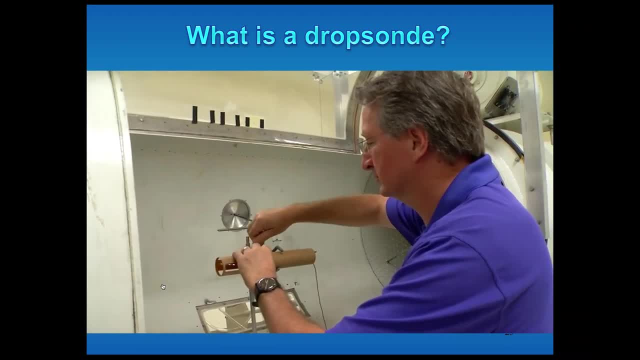 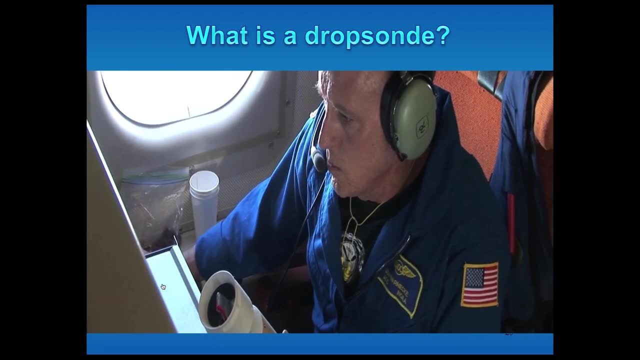 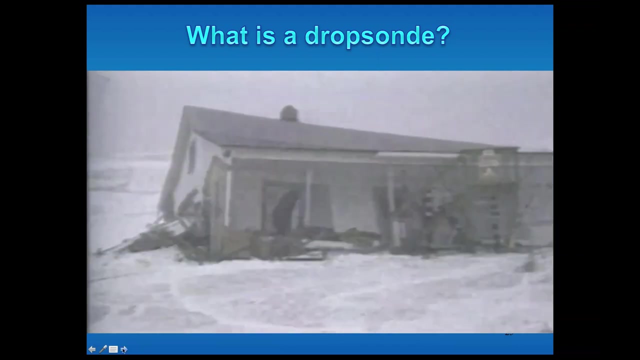 Such inside information is helping scientists learn more about the atmospheric conditions that spawn hurricanes. Hoke expects this will help forecasters make earlier and more precise predictions, giving people in the path of a killer storm more time to evacuate out of harm's way. For Science Nation, I'm Miles O'Brien. 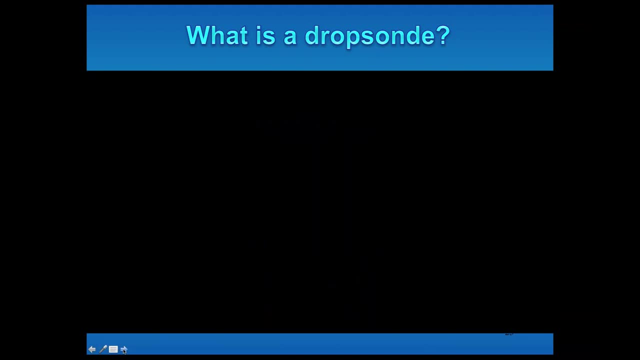 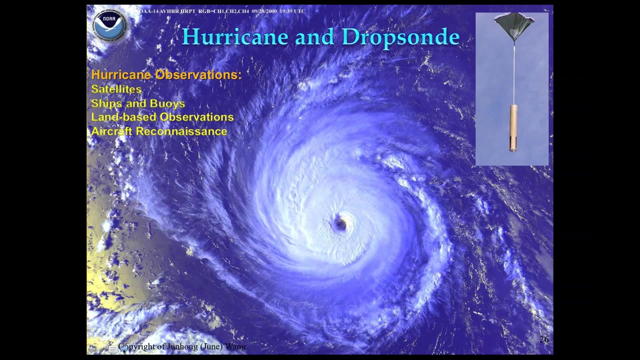 So drop sondes are a very important way that are being used to fill data gaps in regions that are difficult to get data. This slide shows a picture of Hurricane Katrina on August 28, 2005.. Now, hurricanes are one of the most powerful natural hazards known. 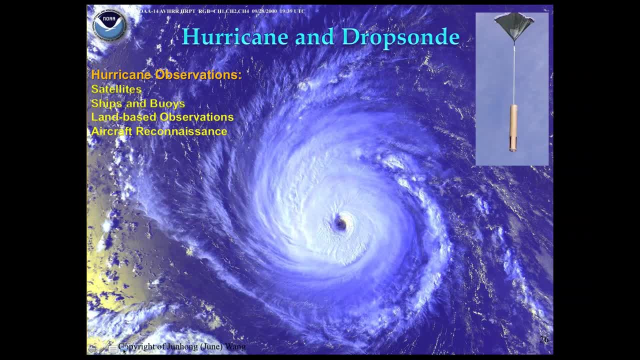 to humankind. We don't have the ability to control them, but we can do a better job to prepare for them. One way is to improve hurricane forecasting Now. hurricane forecasts need observations to initialize and constrain them. These observations can come from several sources. 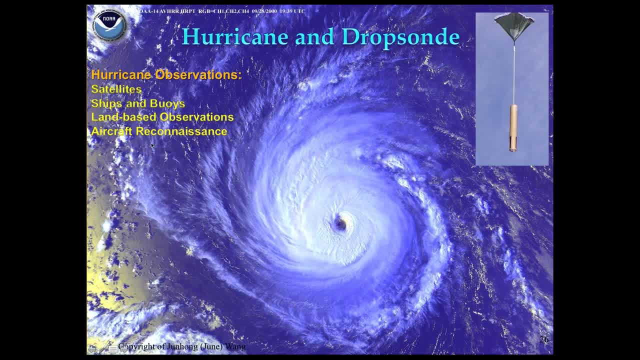 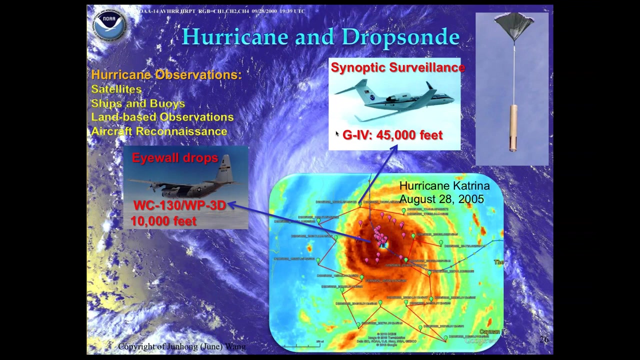 Satellites, ships and buoys, land-based observation and aircraft reconnaissance, But one of the most important instruments for hurricane reconnaissance is drop sondes from aircraft. This actually shows a picture of what a drop sonde looks like here. So in Hurricane Katrina, 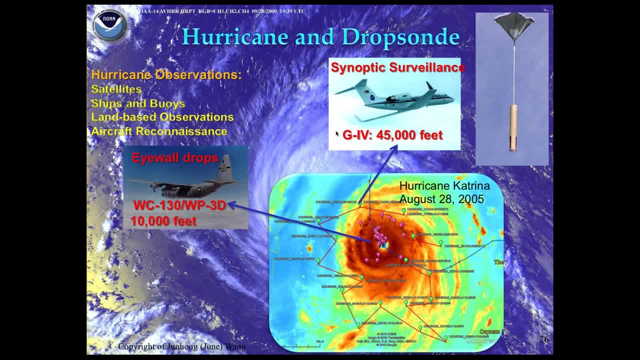 two aircrafts made drop sonde observations and this shows actually what their flight tracks were. So one of the aircrafts was flying at 45,000 feet. that's shown by this red track here and these little balloons show where the drop sondes. 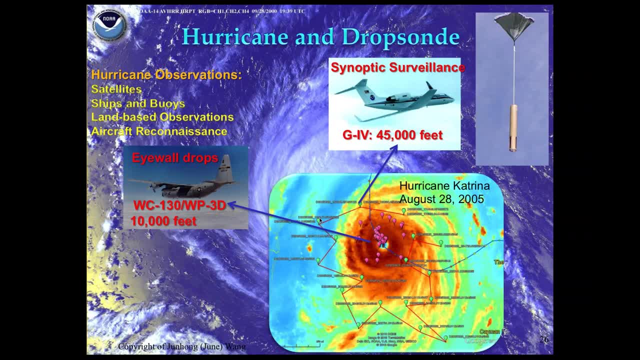 were made. Now, the mission of this aircraft, of these drops, were to better sample the large-scale environment of the storm, to determine the steering current for this hurricane. Now a second plane was flying at a much lower altitude: 10,000 feet. 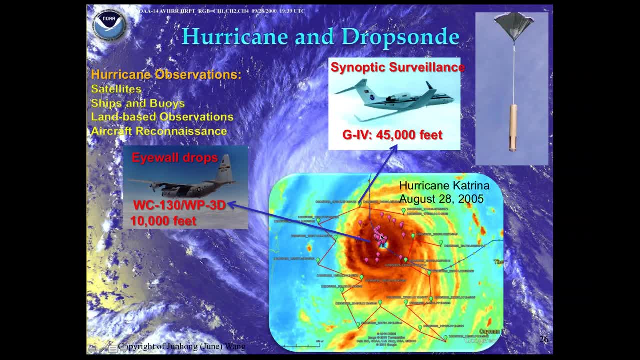 and its drops were primarily seen by these purple-colored balloons, were primarily in the eye wall of the storm, to allow the forecasters to better estimate the intensity of the storm and the wind speeds in the eye wall region. So during the last 17 years. 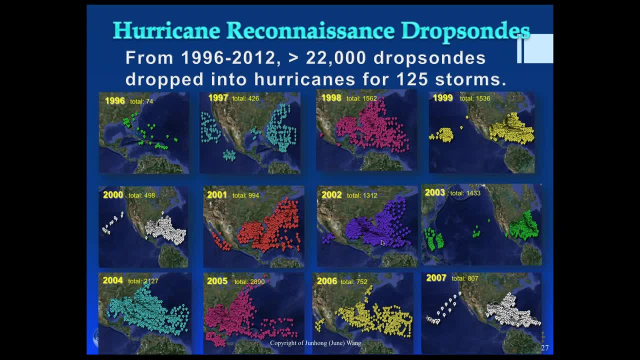 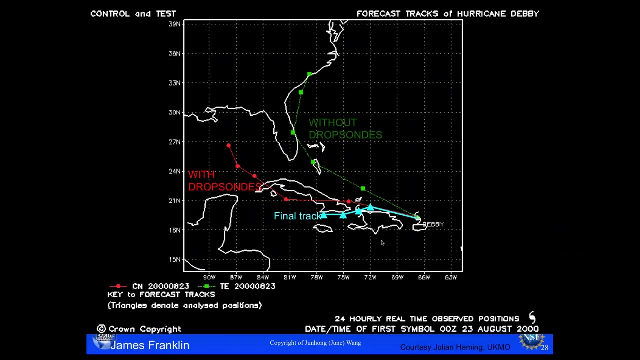 NOAA and the Air Force have dropped over 22,000 sondes into hurricanes And this shows what the pattern for these drops for many of these years. So this slide actually shows the track of Hurricane Debbie that's shown in this cyan line here, But it also 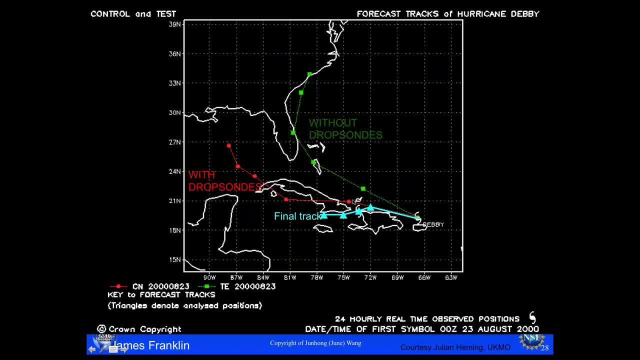 shows the track for Hurricane Debbie, which was in the year 2000,. made with a numerical model that did not include any drops on information And you could see that forecast takes the hurricane track up the east coast in Hennig Florida. 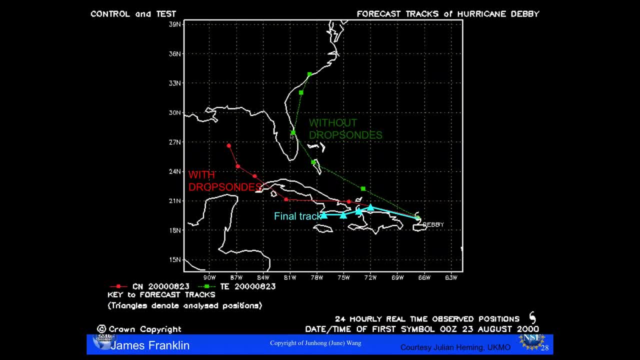 In which case, if we went by this track, we would be issuing forecasts to evacuate much of the east coast in Florida. But when they put the drops on information into these numerical models, you can see that it did a much better job. The forecast track is much. 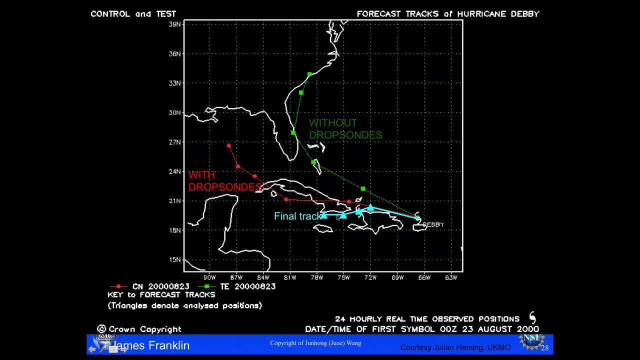 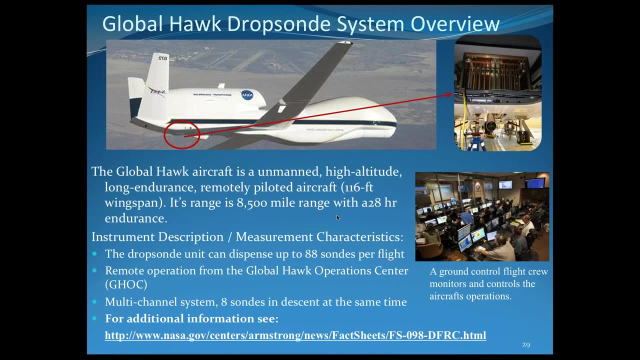 farther to the south and much closer to the final track of the storm. So this drops on information has been crucial in helping us improve the track forecast. So another way that drops ons have been deployed is with the Global Hawk drops on system And that's summarized in this. 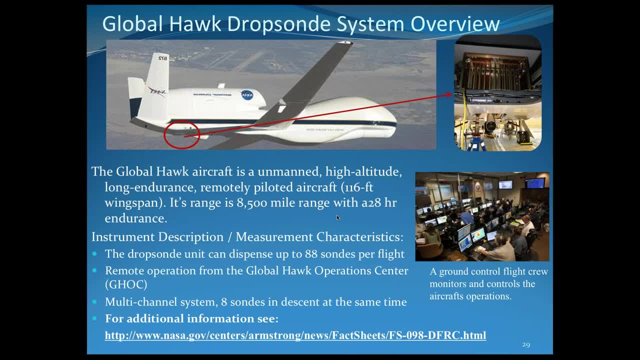 slide. The Global Hawk aircraft is an unmanned, high altitude, long endurance, remotely piloted aircraft. It has a wingspan of 116 feet, Its range is over 8,000 miles And it has an endurance that can stay in the air for up to 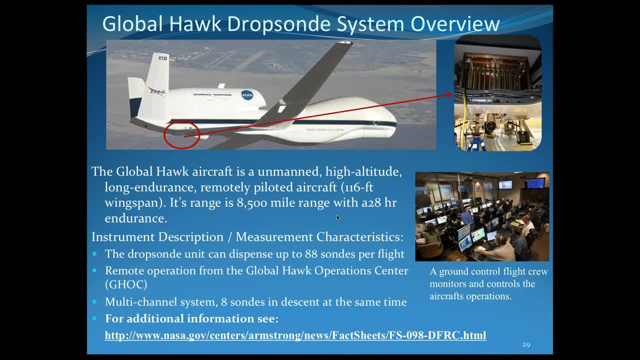 28 hours. So it's actually controlled by a ground crew And this actually shows with that ground crew. here they're monitoring the aircraft and the observations that are coming in. The aircraft actually has 8 channels, so 8 soundings can be in the air at the same time. 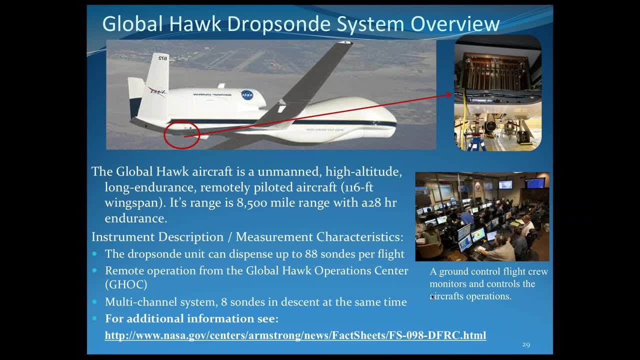 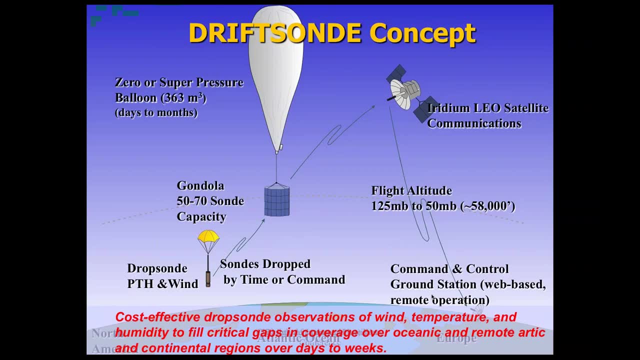 So more information if you want to find out. there's a link included here about the Global Hawk drops on system. So now I'd just like to briefly talk about the Drifts On concept, which was mentioned in the video. Now, Drifts On. 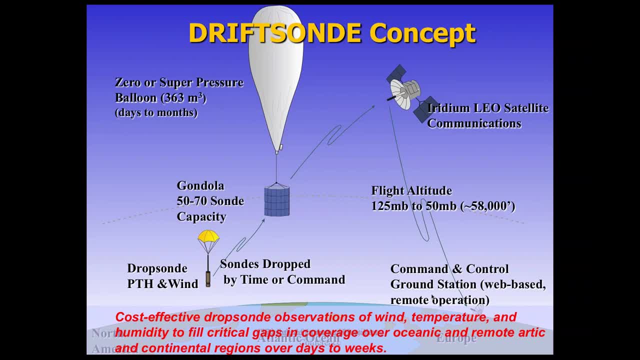 deployments actually started in 2003.. Now Drifts On is nothing more than a huge balloon which is launched from the ground and it carries a gondola up to the stratosphere And it stays there for up to several days, up to 10 weeks. 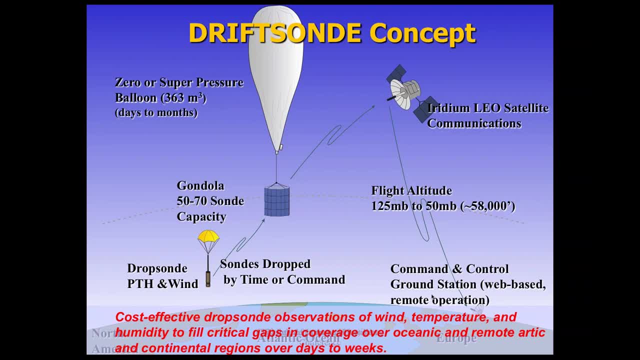 So the winds in the stratosphere carry the balloon along and it just drifts along with the stratospheric winds, And then the sands are actually released by a command that's given, sent to this gondola from the surface, or either they're time released 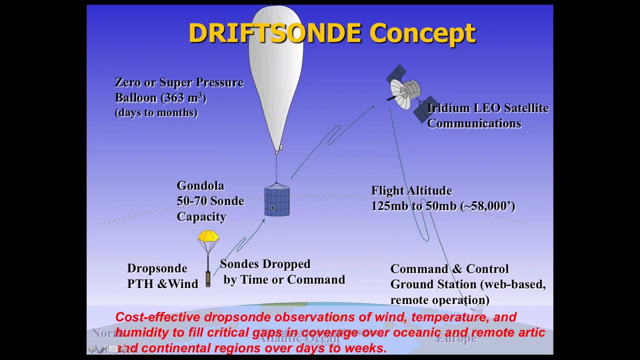 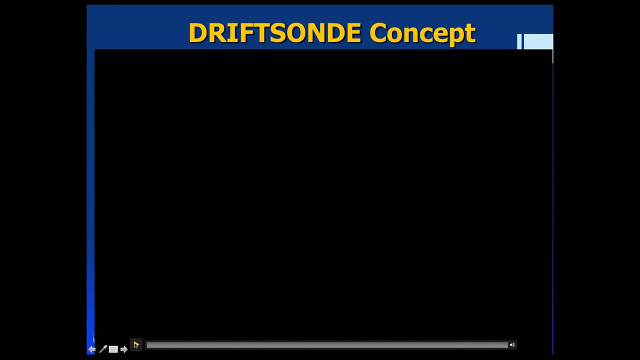 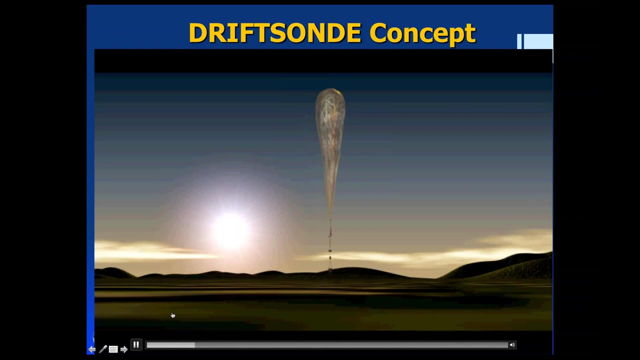 So the drops on send the information back to gondola, which sends it to the satellite which then relays the information back to the ground station. So I have just a very short video which discusses, illustrates this, Drifts On concept. So again it's a very large. 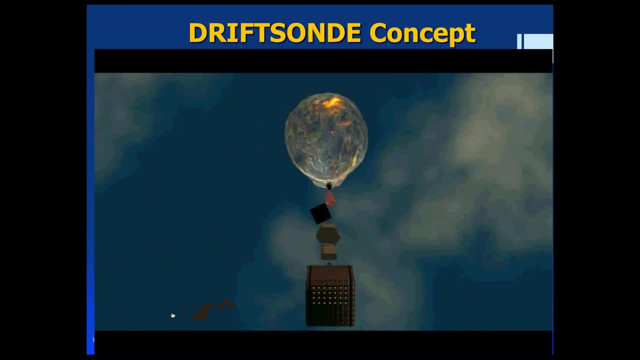 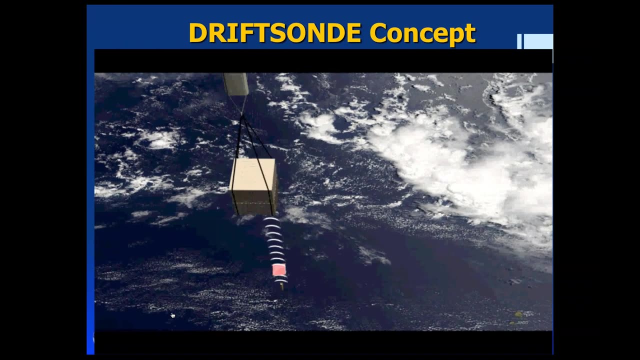 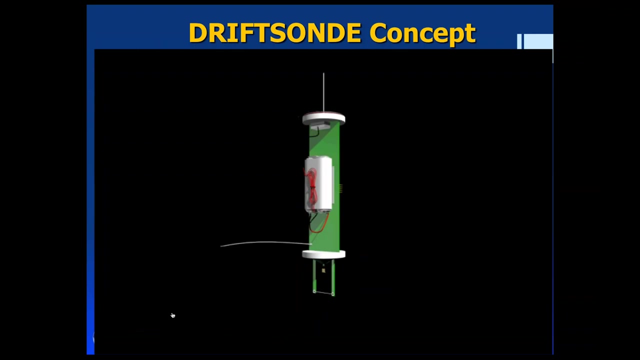 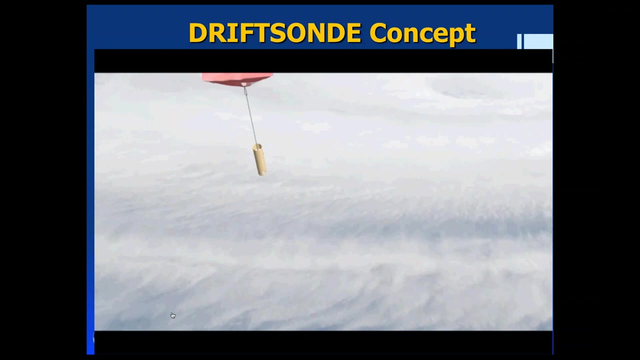 helium filled balloon. It carries this gondola up into the stratosphere. Stratosphere is anywhere from 10 to 18 kilometers, depending on where you are in the globe. This is from 6 to 12 miles up And it shows some of the instrumentation. 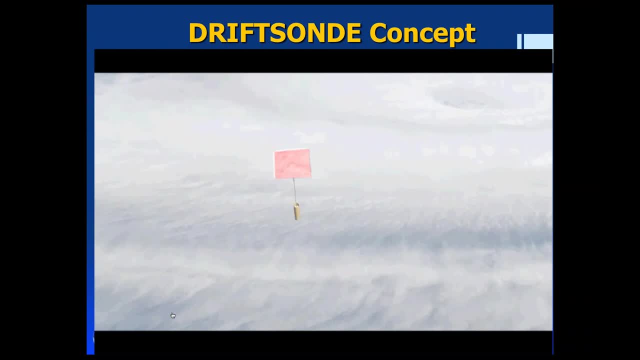 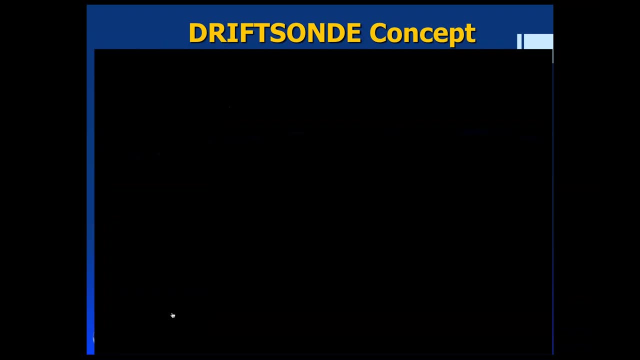 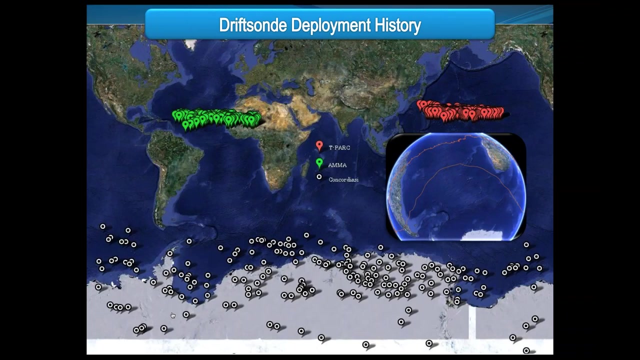 on the Drifts On, And Drifts On has a parachute as it comes down slowly, So this is a great way to launch radio sands in remote regions. So again, the Drifts On have been deployed, starting in 2003.. 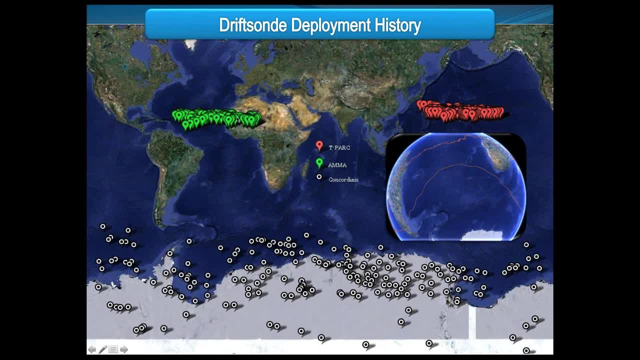 We've used them in three major field campaigns. One is in Africa and over the eastern Atlantic to study the origin of easterly waves that develop into hurricanes. They've been launched over the west pacific to study the strong typhoons that form there. 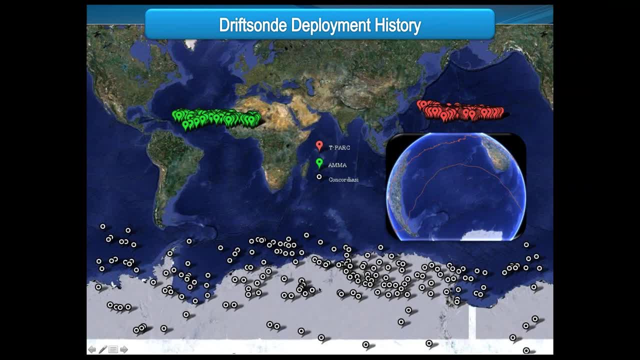 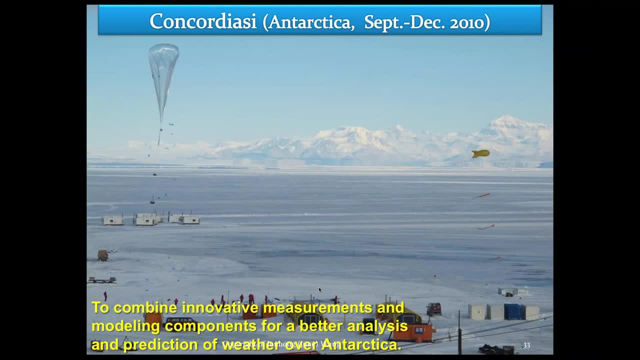 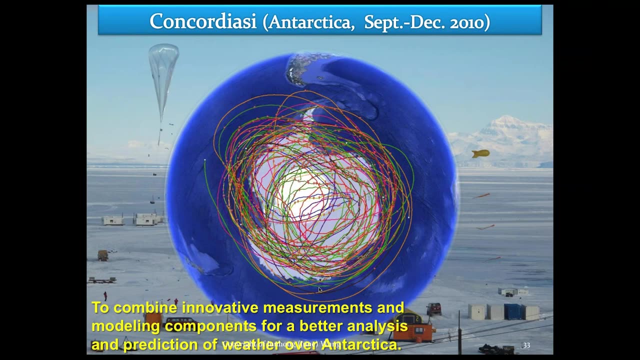 And then also over the Antarctic. This slide actually talks about the Antarctic experiment in which Drifts On were used. So in this experiment this shows the actual course of these Drifts Ons. There's actually 13 Drifts Ons that were. 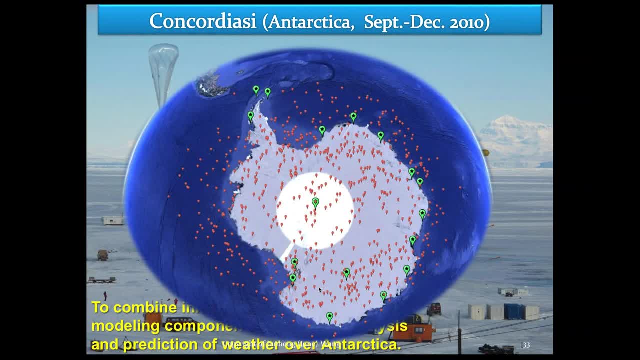 released. These are where all the soundings were taken. The green little balloons here show radio sound sites that were used during this experiment on the ground. But look at all the soundings over the ocean and inland, over the Antarctic We were able to sample. 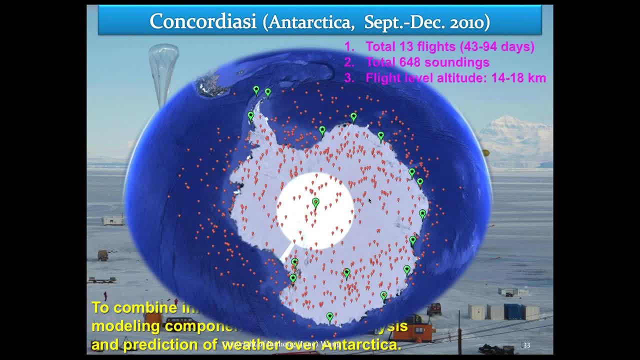 observed regions that had never before been observed. So there were 13 Drifts Ons that were sent up. They were up there anywhere from 43 to 94 days. They took over 600 soundings from altitudes from 14 to 18. 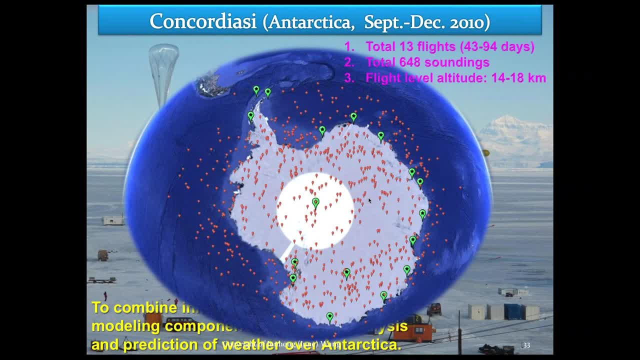 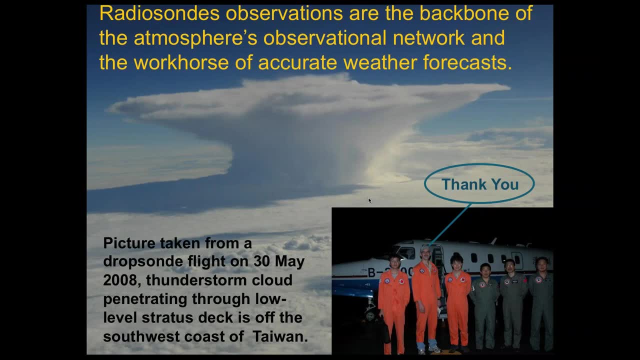 kilometers. So this provides again observations in regions that have never been observed before. So, to conclude this talk, I hope you've gained an appreciation of the importance of radio sound observations, That they truly are the backbone of our atmosphere's observational network and the workhorse of 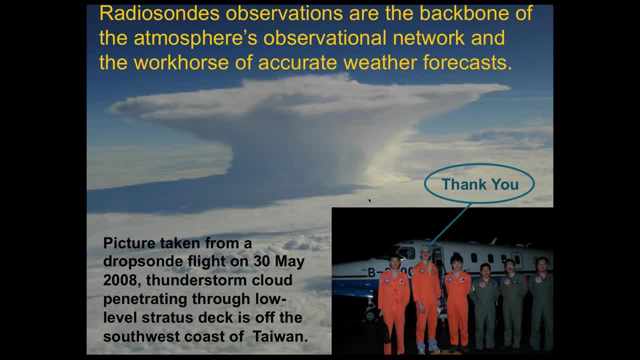 accurate weather forecast. This picture I actually took from a Drifts On flight that I was invited on. This was from May 30, 2008, and I was looking out the window of the plane that was making the drops ons, And this shows a thunderstorm with this. 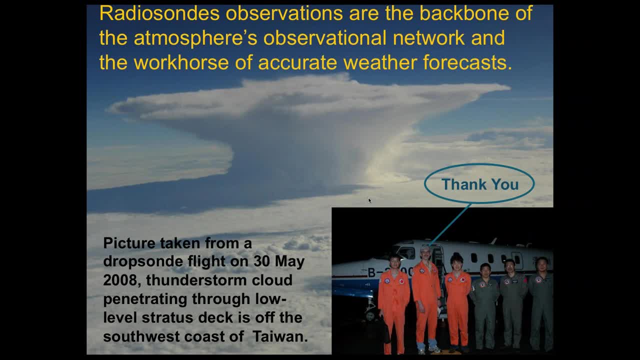 beautiful Andal cloud And this thunderstorm is penetrating through a low stratus deck off the coast of Taiwan And they asked me when I was in this flight that I needed to wear this outfit in case the plane crashed- They'd be able to find me. 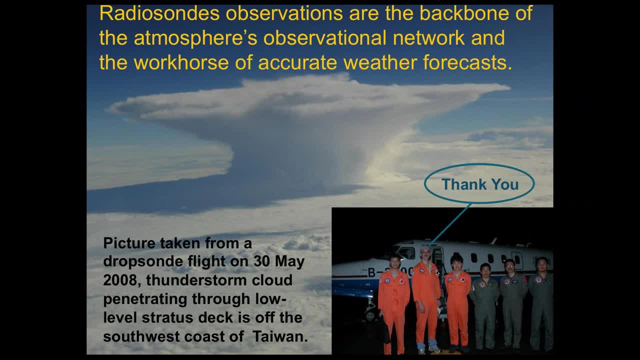 easier. I can't swim with a lick, so that wouldn't have made any difference. But I asked for the largest outfit they had because I'm six feet four and you could see that it does come a little short. It was a little tight on me. 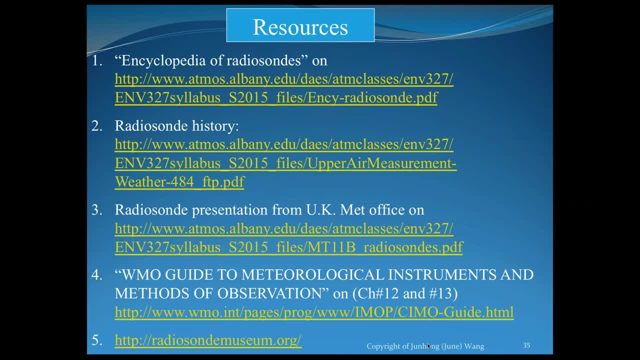 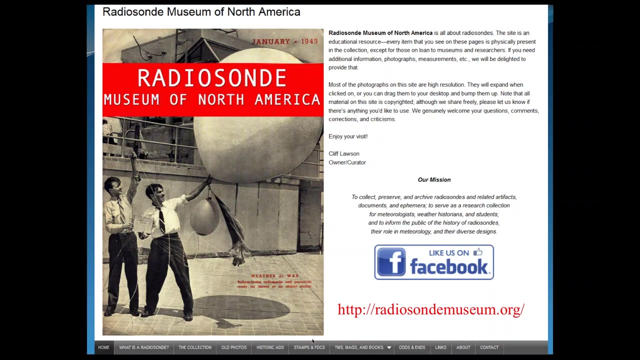 So here are some additional resources. if you're interested in additional information on radio sounds, I'd like to call your attention to this bottom link here, which is about a radio sound museum. This museum is actually located in Mississippi and it was started by a civilian. 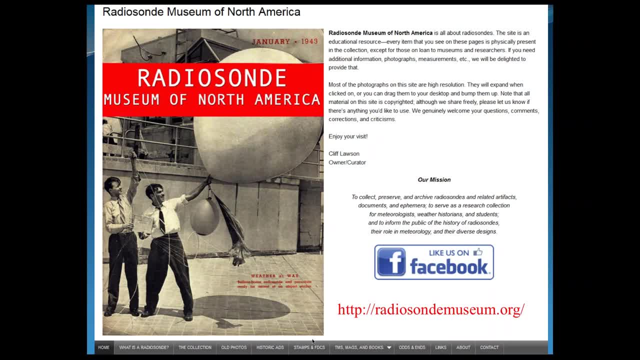 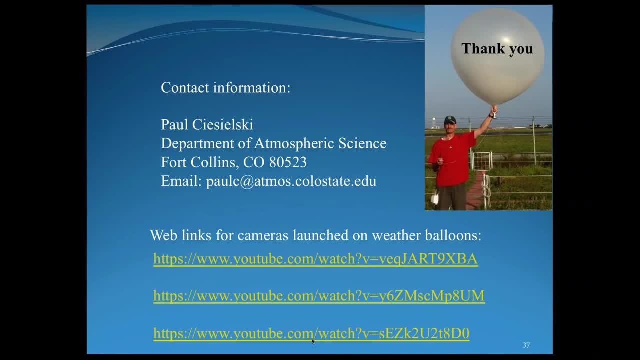 who has been collecting radio sounds for the last 40 years. And finally, here are some links to cameras that have been launched on weather balloons, And these videos are really fun to watch. It'll give you some idea of the varying conditions that a sound would experience. 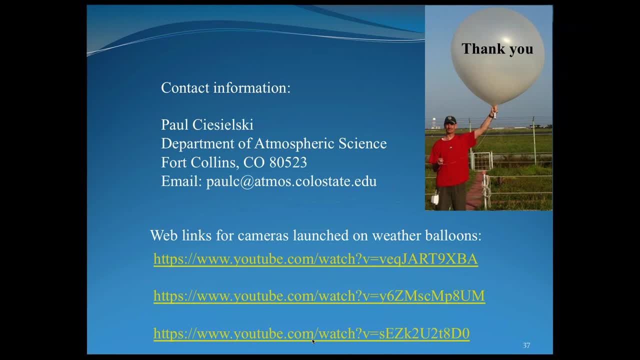 as it goes from the surface into outer space. So thank you very much for your time and I'll be happy to entertain any questions. Paul, thanks so much. Great presentation there. All these links that Paul has just shown on his screen we have on our. 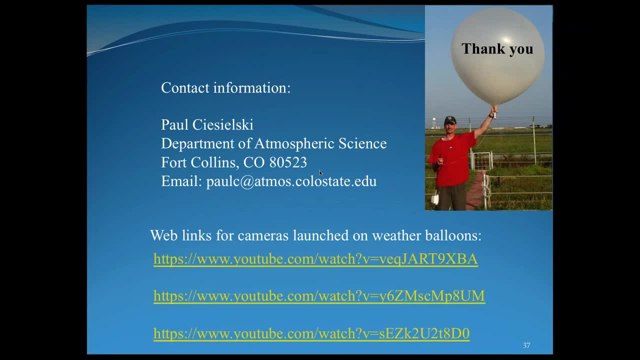 page, our WeatherTalk page. If you'll go and you'll click down at the bottom of the page, it'll show the talk from today. We'll have that up later on today along with this presentation. So again, thank you so much for giving this. We're getting a couple. 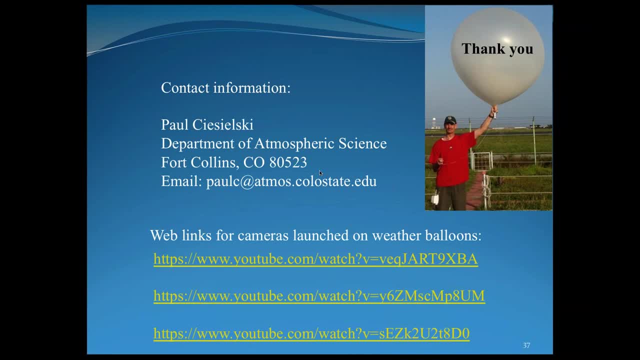 of questions starting to come in now. Are you ready to take a couple? I'm ready, Okay, well, this is an interesting one. and Beth writes in. excuse me, Jeffrey writes in and Jeffrey wants to know how do we keep aircraft from crashing into them? 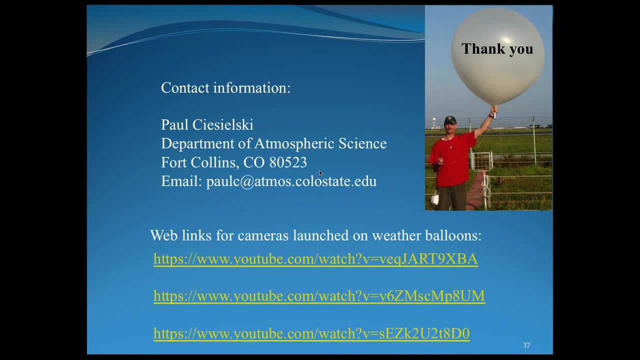 Most are launched near airports and major metropolitan flight factors. He's a pilot and thinks this is a great topic. So there you go. Well, that's a really good question because, you're right, Many of them are launched near major airports And I don't have a good answer. 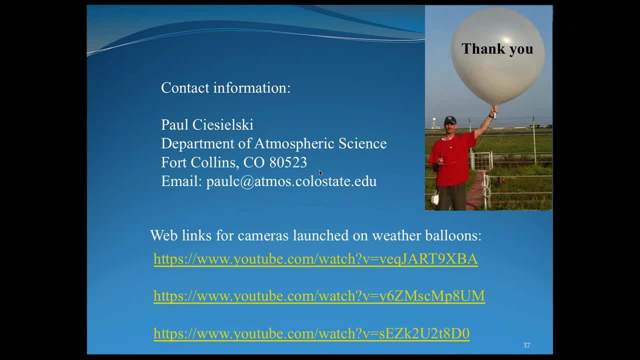 for that, except to say that these soundings have been designed so that if they get sucked in to the engine of a jet, it doesn't do any damage to the jet. Of course the radio sign is toast, And when we do our launches in field experiments, 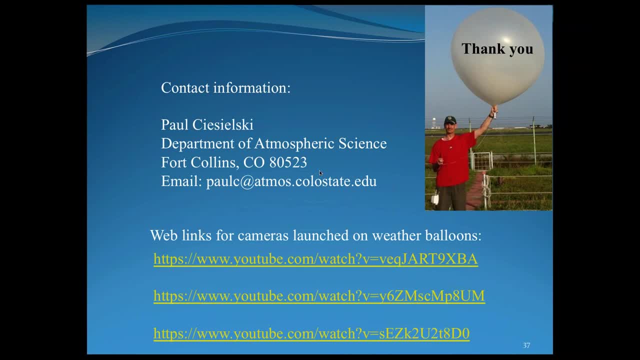 we usually need to call an airport if it's nearby and ask for permission to launch And they'll say: go for it or don't go. So we have to abide by what they say. As far as I can tell, the aircraft have very few. 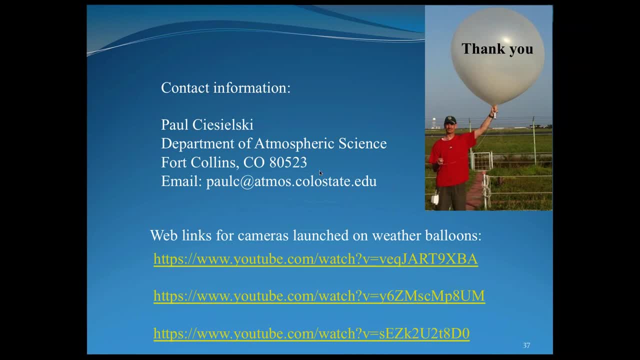 issues running into these radio signs. Henry, I think you're still muted. There we go. Sorry about that. Robert writes in: wants to know the cost, weight and accuracy of the Sipicam MK2.. If you have any information on that, 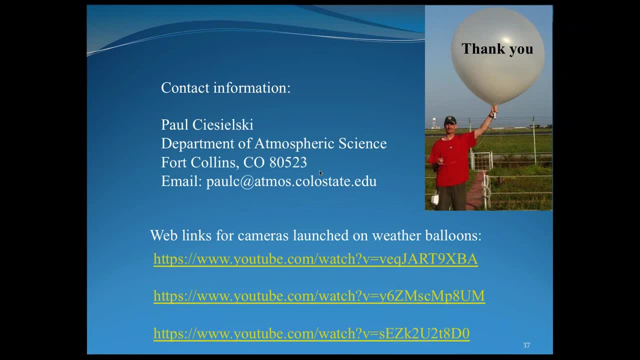 I'll have to get information on that. I don't know. He wants the cost of what was that? again The cost, weight and accuracy of that unit, Of which unit? The Sipicam? Oh, the ones that's. 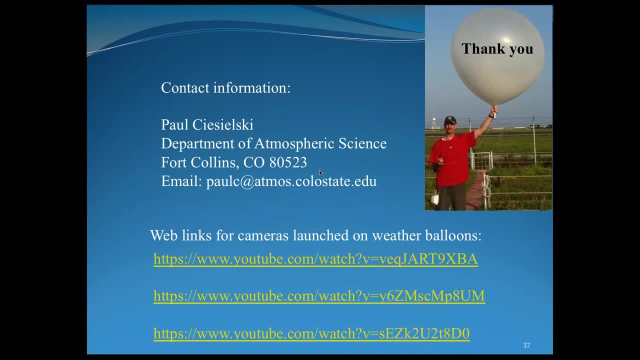 used in the US, Right? Well, I'll just say this. I know that the Vaisala Sond that we use in our field programs. I mentioned that they cost about $300. And the US uses. they use that type of Sond at a few. 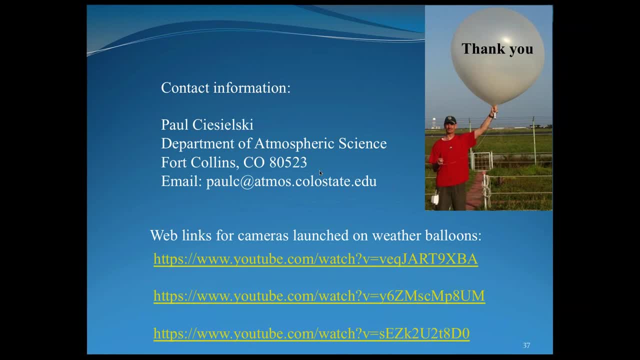 sites, But most of the sites use this Sond. that's a Sipicam Sond that was manufactured by Lockheed Martin And I'm sure one of the reasons why the US uses it is because it's cheaper than the Vaisala Sond. 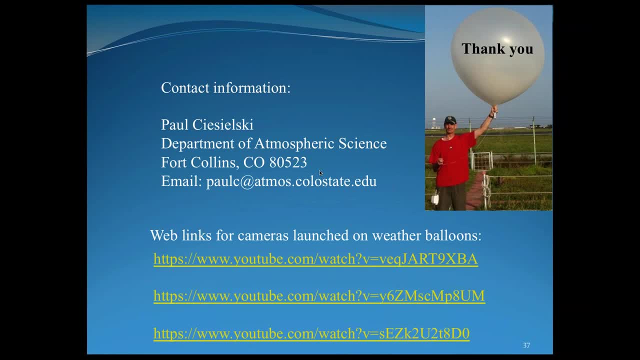 And it likely is not as accurate, though, But I'll try to get more information on that. Okay, great, Here's one coming in, Let's see. Mark wants to know: are you looking to replace Radiosond with drones? 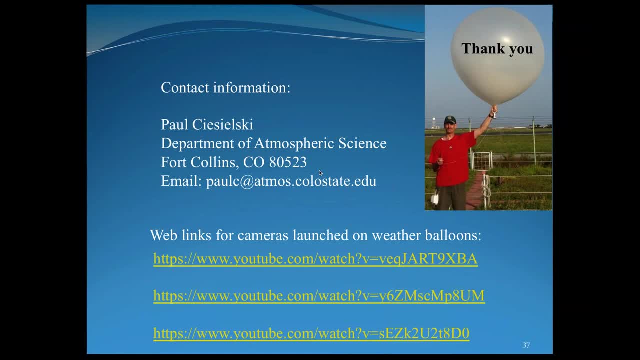 I guess that is an option, but no, we. the methods that I've talked about here are the current methods for taking observations. Now there is, there are some- what are they called? It's they actually put these instrumentations on very small piloted 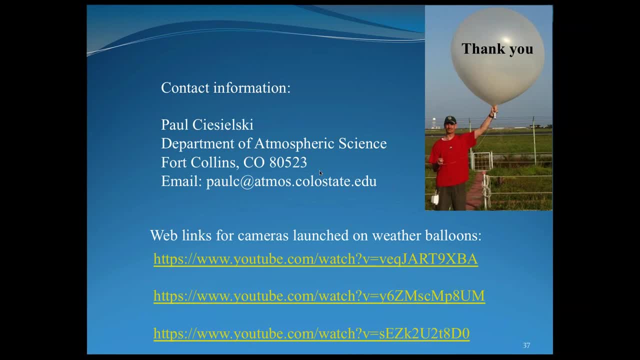 remotely piloted aircraft, Almost like toy ones, And we've used those to try to take measurements in some storms. but you know, if you release those in any kind of difficult weather, chances are you may not get the instrument back because they 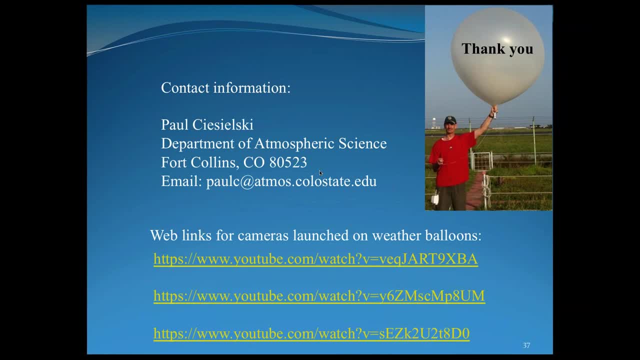 have a difficult time navigating the strong winds, like if you try to release them into hurricanes or thunderstorms. Okay, Travis writes in and he's referring to the Scuti diagram you showed earlier. I don't know if you can bring that up, but he wanted to know. 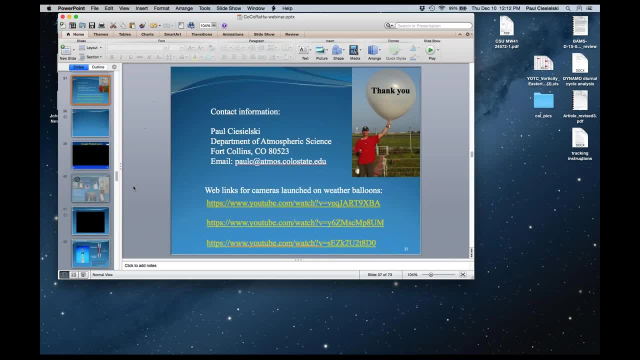 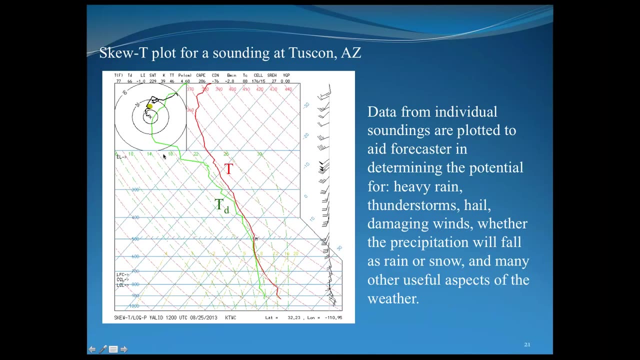 what information is shown by the Radiosond in the round circle on the Scuti graph. Okay, let me see if I can bring that up. I think he's probably. So probably the top left corner of the Scuti, that's the one. 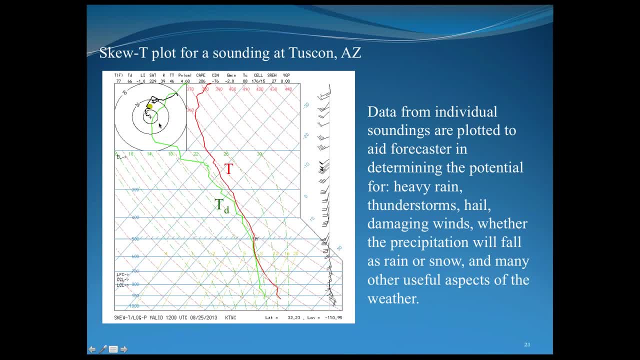 Yes, this here is what's called a wind hodograph, and it basically shows how the wind changes with height. Now, I'm not an expert in severe weather, but those who are could look at a hodograph and say, whoa, this wind shear here. 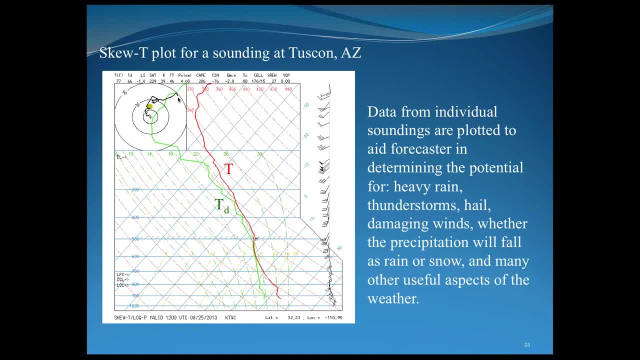 profile is conducive to severe storms or tornadoes. Usually, when you see a lot of wind shear in the lowest levels, that's an indication that the atmosphere has potential for tornadoes or very severe winds. So that is what's called a wind hodograph. 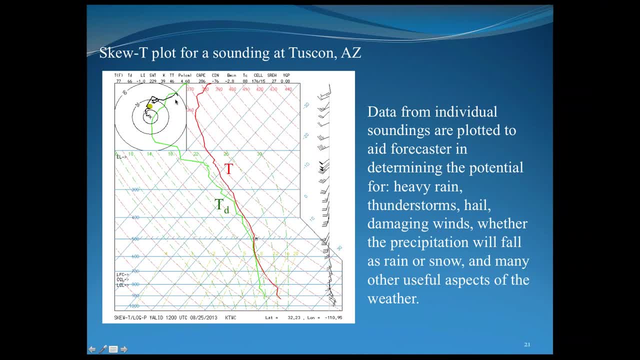 and it does show how the winds change with height, the wind direction. Jim writes in and he wants to know: has anybody ever been injured by a returning probe when it's falling back to Earth? That's a good question. The only injury I've heard. 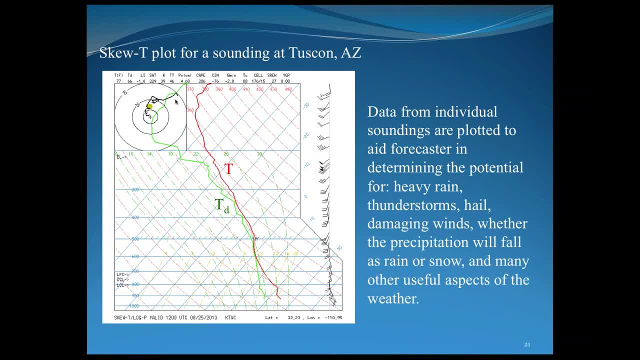 is that of a balloon that was hung up on a power line and the person who was trying to get it out of the power line was actually, unfortunately, electrocuted and died. But keep in mind that the National Weather Service they use. 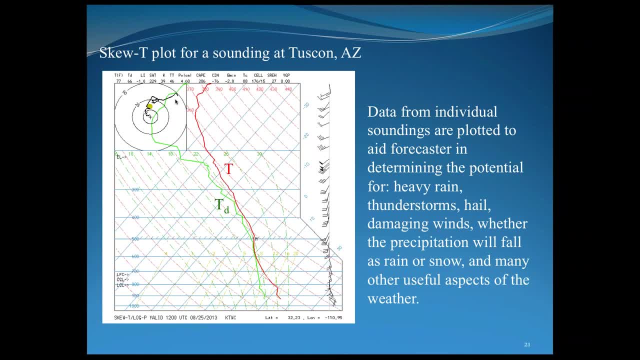 parachutes with these. so these systems, which weigh only about a pound, I don't think they would do much damage, even if you got hit in the head with one. Robin writes in and she wants to know that. she says: why not put a tracker of? 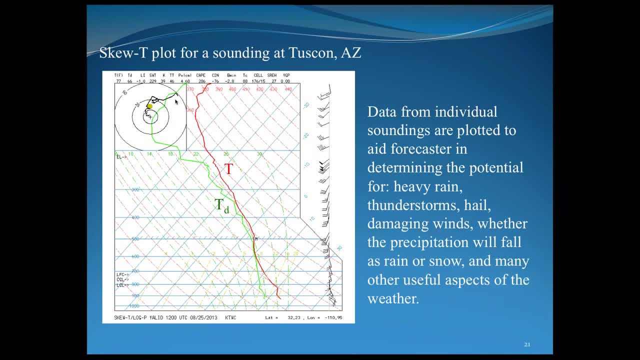 some sort on the signs to aid in their recovery. Okay, well, that's a good question, Robin, and actually these soundings have the GPS position when they're in flight, but when the sound say, we release a sound here at our building at Colorado. 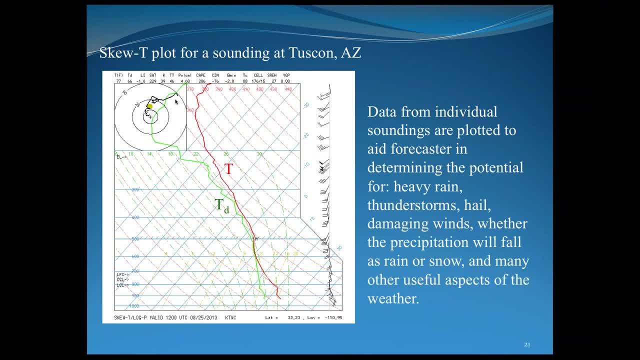 State University. well, it gets picked up by the westerly winds and those winds might transport that sound possibly 100 miles or 200 miles. So if we track that sounding on the way down, we usually lose communication with it at about. oh, I'd say one or two. 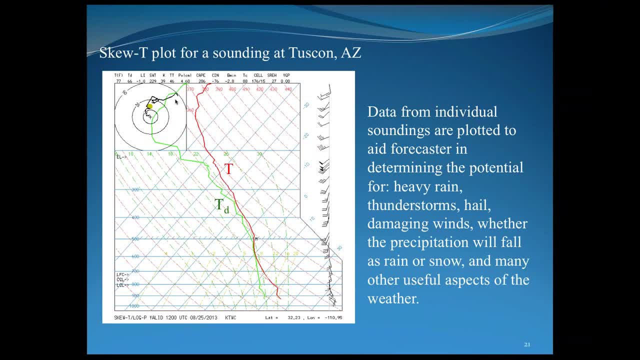 kilometers off the surface. because of the curvature of the Earth, It no longer can transmit the information back to our ground station. So that is a good idea and very expensive probes are often tracked that way and they try to estimate: oh, this is the last. 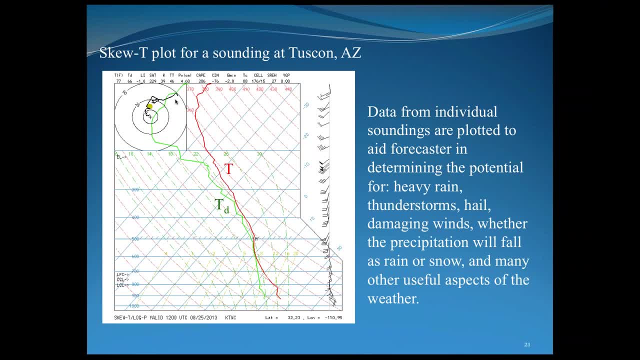 place. we saw it, so let's try to find it with GPS information. I guess it would be pretty costly too. if you had one. you found that it was 200 miles from your location and driving out there time-wise and so forth to pick it up. 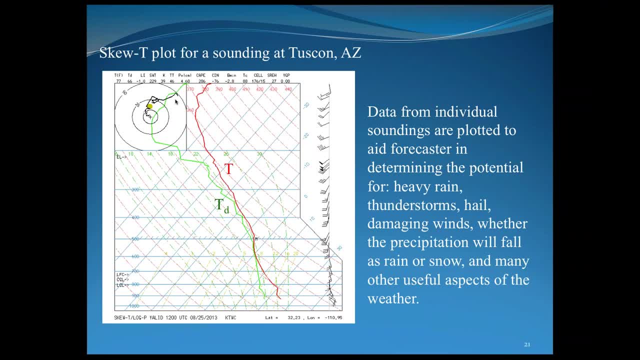 Yes, probably would. Larry's writing in and he wants to know: are the sounds in flight subject to lightning strikes? Any chance of anything getting affected by lightning? Oh, yes, I mean, if you launch these in severe weather, you'll often notice the data. 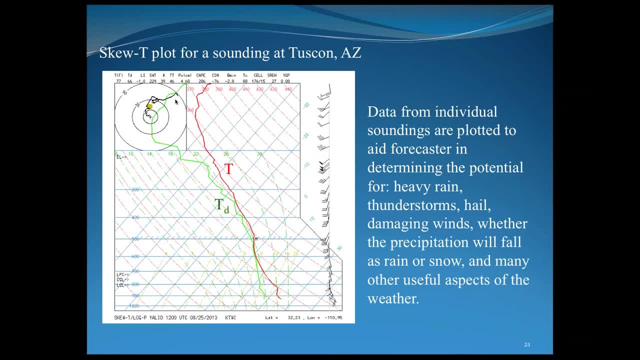 only goes up a few kilometers and then it just ends, and there could be a few reasons for that. One reason, as you probably can imagine, it got hit by lightning. Another reason might be is that the balloon has iced over and, as 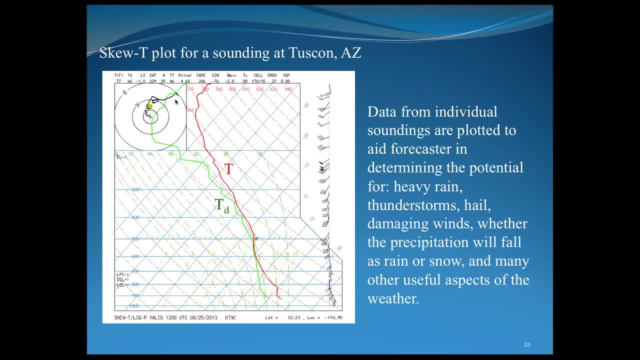 the ice on the balloon is so heavy it's not able to get any higher. So often what we might see is that the balloon ices up and then it descends. the balloon warms as it descends and the ice melts off again, and then it. 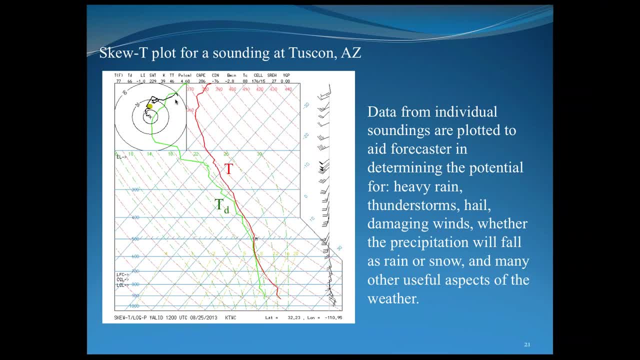 rises and it might hit that icing condition again, and this might happen several times. So that's happened. but yes, when balloons are launched in severe weather, we often lose the signal, probably because of the probe was hit by lightning. Here's a question by Ron. 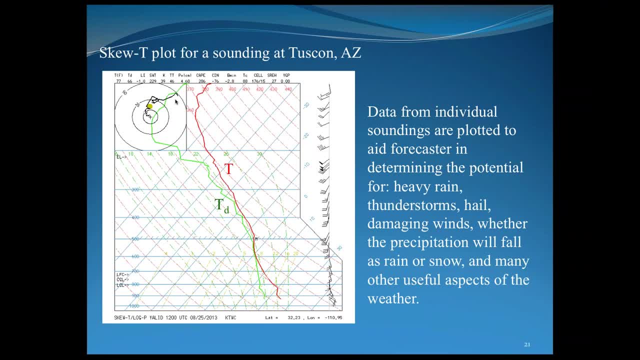 and Ron wants to know: is there any way that an amateur radio operator could possibly receive and decode radio sign information off the UHF data stream with a beam of some software that may exist out there? That's a good question and I would think, if you have a receiver, 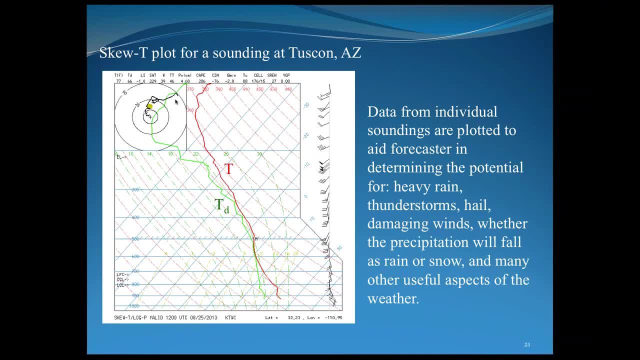 at about 400 megahertz, which is what we use, you could probably receive the data, but you probably need some sophisticated software which is around these ground stations in order to make sense and basically process and decode the data, for it to make sense. 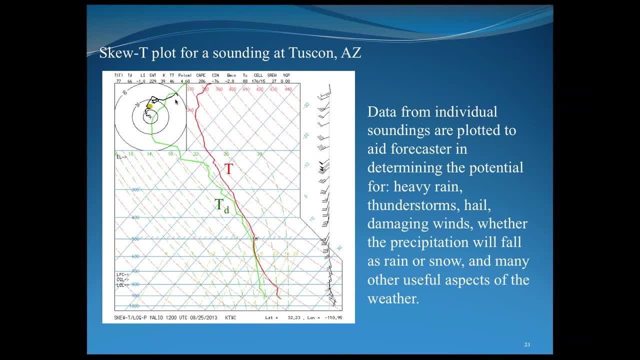 Here's one similar question, one by Ted, and also another one coming in from Gail, and they're wondering why there are holes in the radio sign network, budget, population density and so forth. and then Ted was wondering the lack of stations in the northeast. 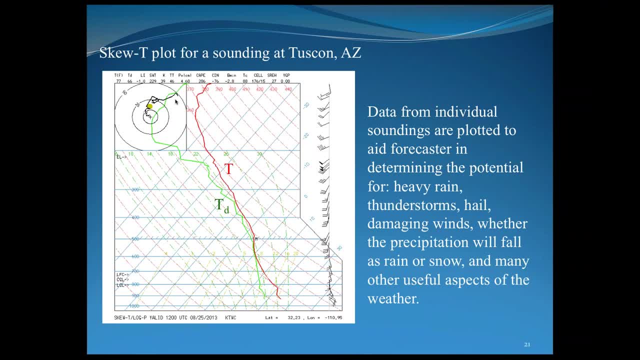 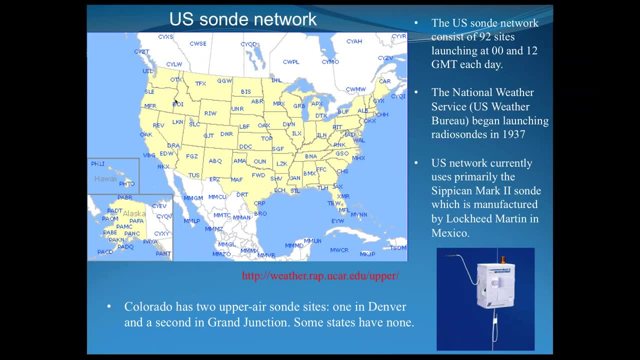 and I think if you brought up that map, it shows Vermont was again. the states are pretty small in the northeast so I'm sure the area is covered pretty well, but there's one on the Cape, there's one in Albany, there's one in. 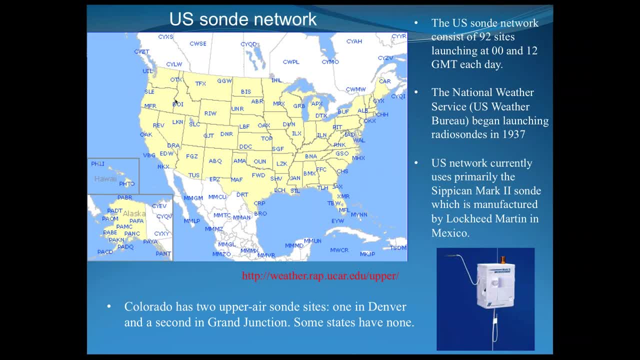 Portland, Maine. Yeah, that's a very good question. As I look at this map, it looks like they've put a radio sign station, or these observations, every two to three hundred miles, and the reason why there's not more is because it's expensive. 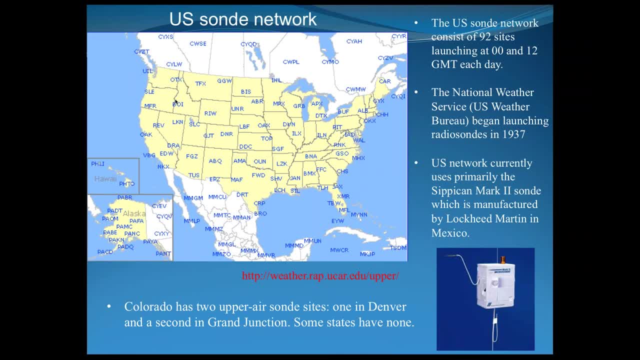 And why they are where they are. I'm not really sure. You know, this network was set up, was actually designed in 1937, and I guess we'd have to ask some of those guys why they put these sites where exactly they were. but yeah, 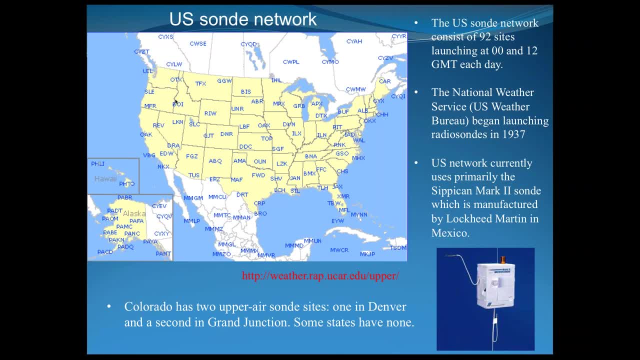 there are definitely holes in the network. Okay, this looks like the last question of the day and actually it's funny. both George and Jim in Missouri both asked a similar question at the same time and they're wondering: why don't you use 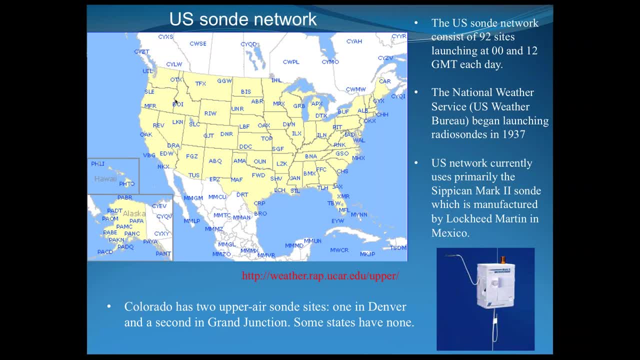 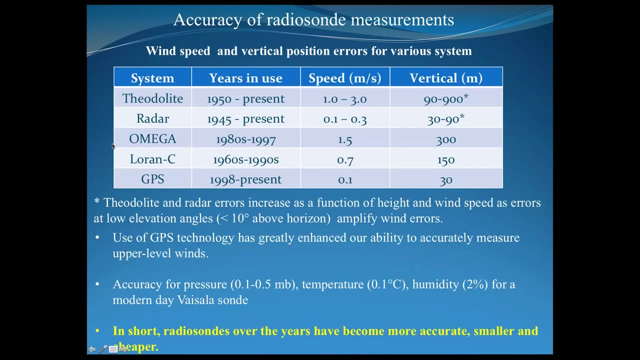 the same type of locator used in the marine XOS beacons to find downed pilots in the ocean. so is that type of transmitter could be used? I would assume that would get pretty expensive. Okay, actually, if you look on this table, 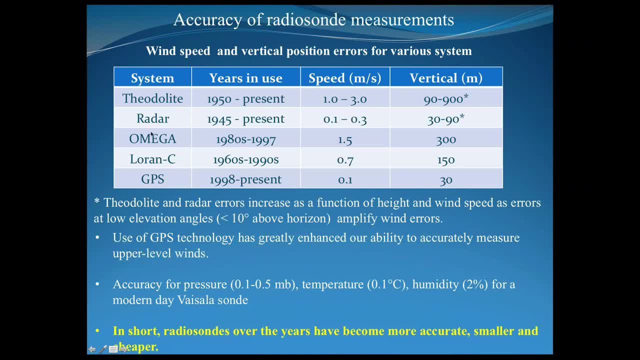 this actually shows that we used some of these navigational aids. The Omega system and the Loran C system were actually navigational systems that have been used by our government, So we've used those in the past. They are not as accurate. they're prone to data drop-off. 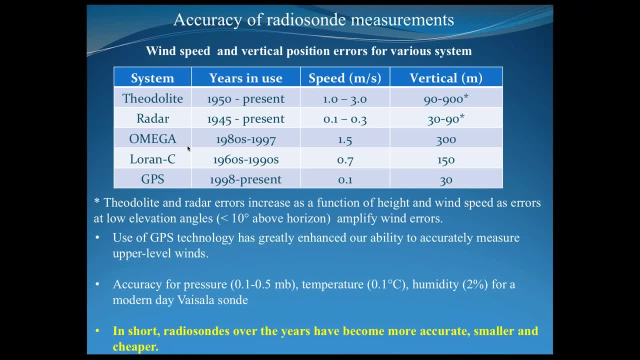 you need to get a good signal from all these ground-based emitters to the sonde, and we just found that the GPS technology- I think I misspoke when I said with GPS, the global positioning system- gives us the most accurate way to determine.